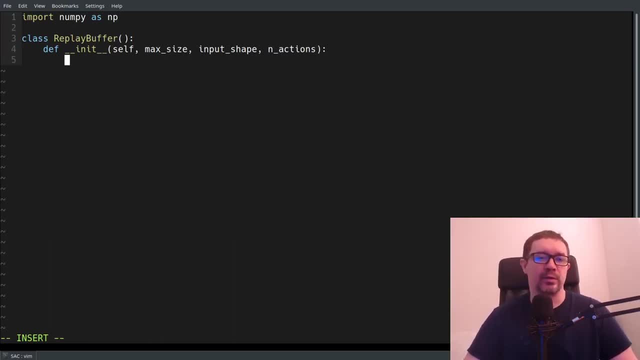 a continuous action environment, And so number of actions means the number of components of that action. So we'll go ahead and save our variables And we need to instantiate a memory counter which keeps track of the position of the first available memory. And we're going to 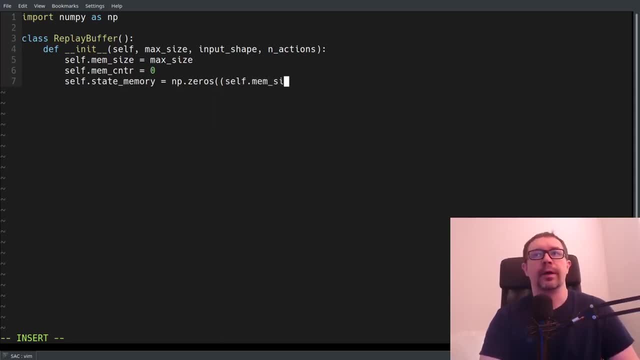 go ahead and start initializing our memory, So that will be shape mem size by input shape. We'll also need a new state memory that keeps track of the states that result after our actions And that is functionally the same size as the state memory. 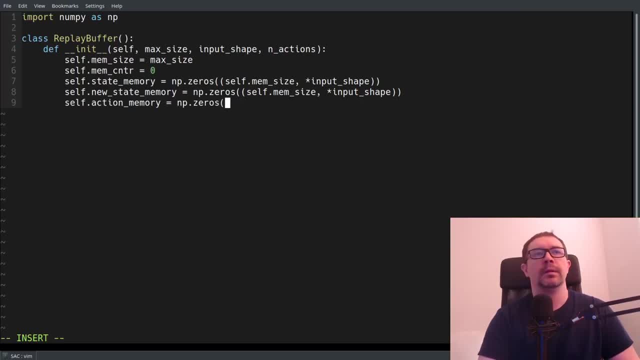 The number of actions. excuse me, the action memory will have shape, mem size by an actions. Again, those are a number of components of the actions. a reward memory to keep track of the rewards the agent receives with each step of the environment, And that's just going to be an array of scalars. 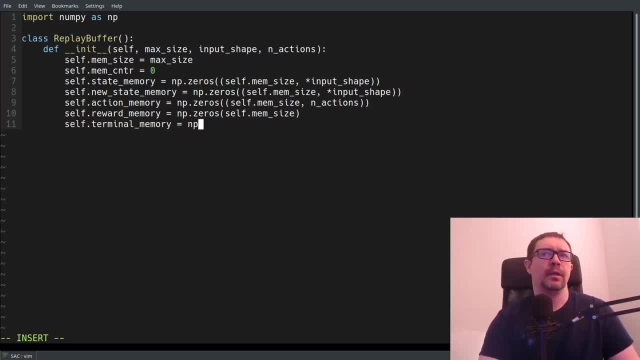 And then we have the terminal memory. Now, the reason we need this is because the value for the terminal state is identically zero And we're going to be storing the done flags from the environment as a way of setting the values for those terminal states to 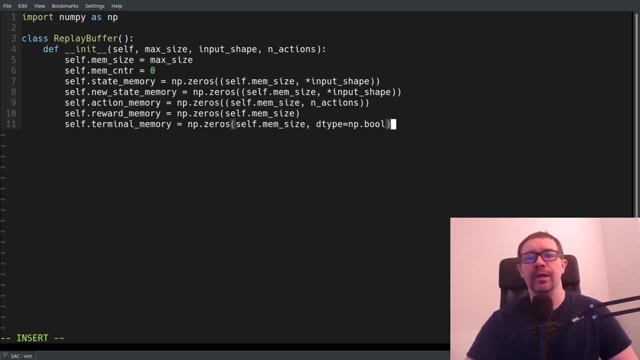 zero And the data type on that is going to be a Boolean. Our first function is to store a transition And that'll take a new state, action, reward, new state and terminal flag as input. The first thing we want to do is figure out where our data is going to be stored, And that's going to be. 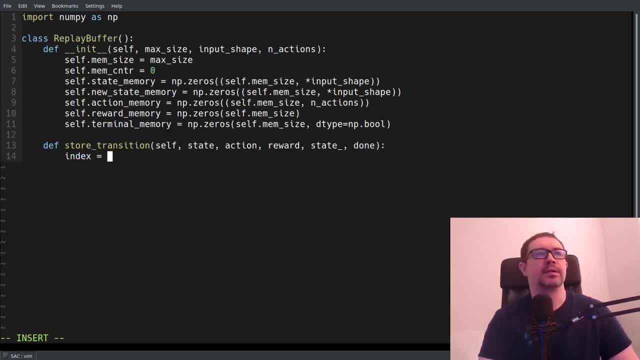 the first thing we want to do is figure out where our first available memory is. So we're going to get that index by taking the modulus of the memory counter and the memory size- Evidently, I can't talk and type at the same time- And then we're going to set the numpy arrays at that index equal. 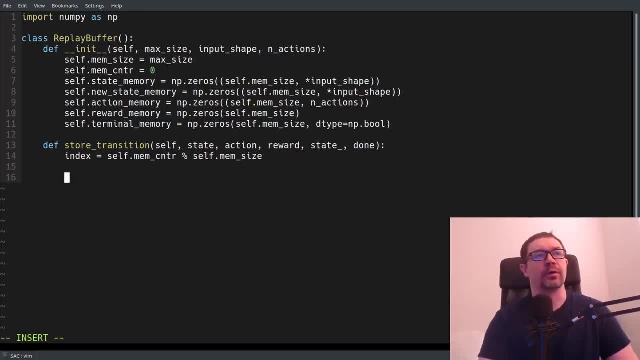 to the parameters that we passed in from our function: terminal memory state, new state action. and we're done. I believe that is it. And then, finally, we want to increment our memory counter by one. So next we want to handle the function to sample our 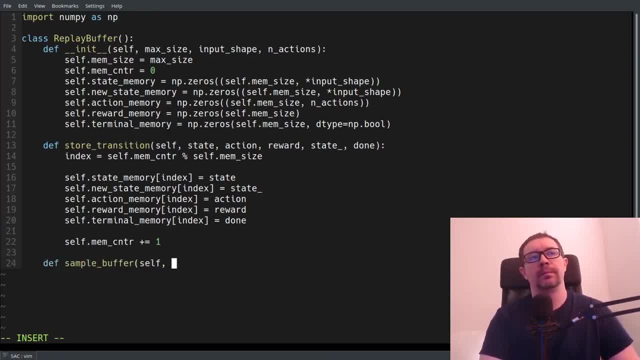 buffer And that will take a batch size as input, And alternatively you can make the batch size a member variable of the replay buffer. it doesn't really matter. The first thing you want to know is: how many memories have you actually stored in your buffer? And it's given by the minimum of the mem. 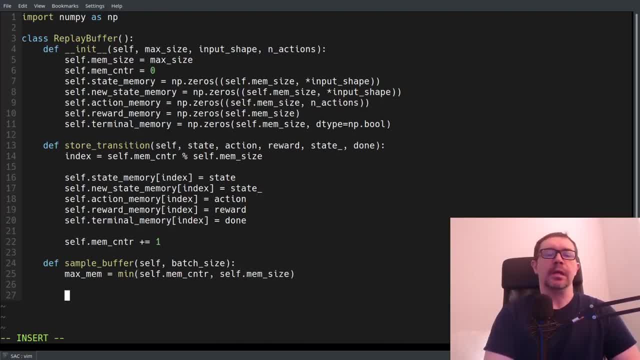 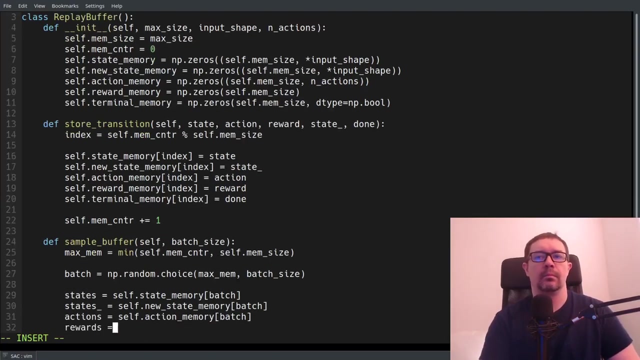 counter and the mem size, And then you want to select a sequence of random integers between zero and that maximum memory And then go ahead and sample those memories. Of course I forgot the self here. Remember he said bad, Which and duns. 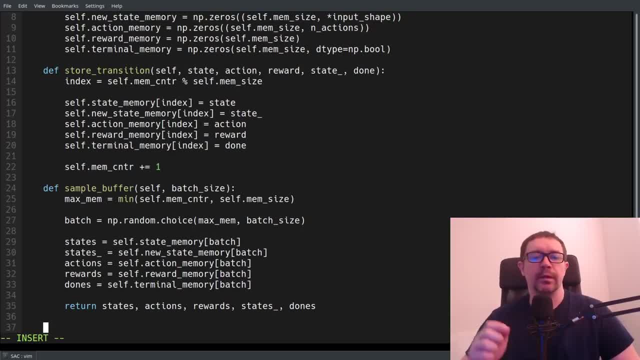 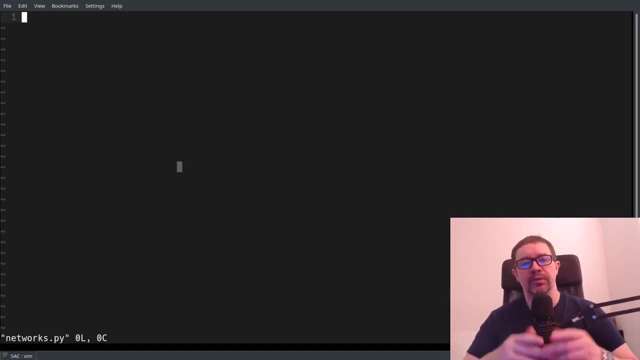 Alright, so that wraps up our replay buffer. Now we're ready to move on to the relatively hard part of the problem, which are is the deep neural networks. So, before we proceed, I want to give a brief- you know, theoretical- overview of what it is we're trying to accomplish. 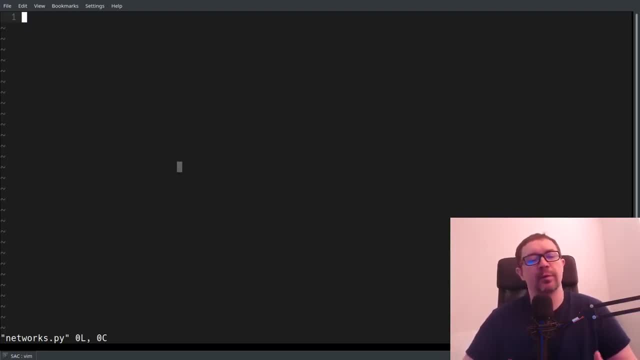 with soft actor critic. So in the soft actor critic algorithm we want to solve the problem of how to get robust and stable learning in continuous action space environments. You can also use algorithms like DDPG or TD three for continuous action environments, And TD three in particular works really well. it's on par with the soft actor critic algorithm. they were developed to. 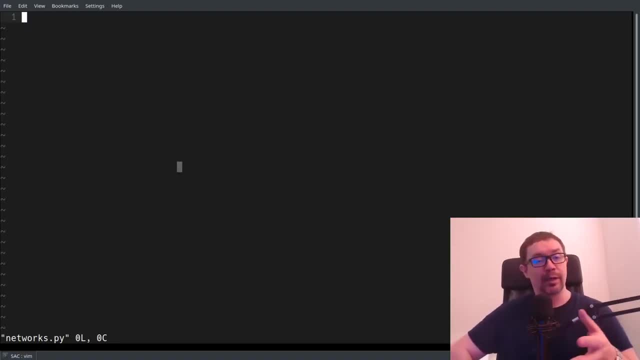 concurrently by separate groups. So they're kind of you know, comparable algorithms in terms of their quality. DDPG falls a little bit short. it doesn't do quite as well as the other two. The basic idea in soft actor critic is that we want to use something called the maximum. 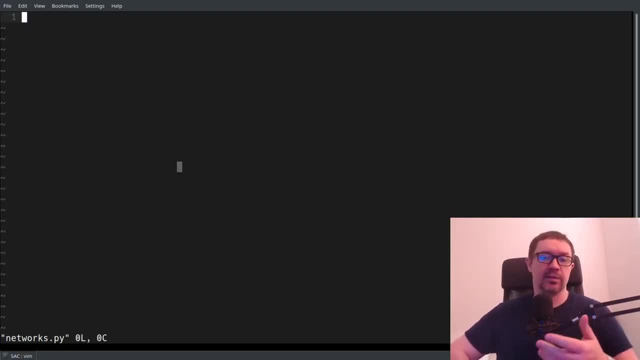 entropy framework. Entropy just means disorder in this case. So it's going to add a parameter to the cost function, or rather, it's going to scale the cost function in such a way that it encourages exploration, but it does so in a way that is robust to random seeds. 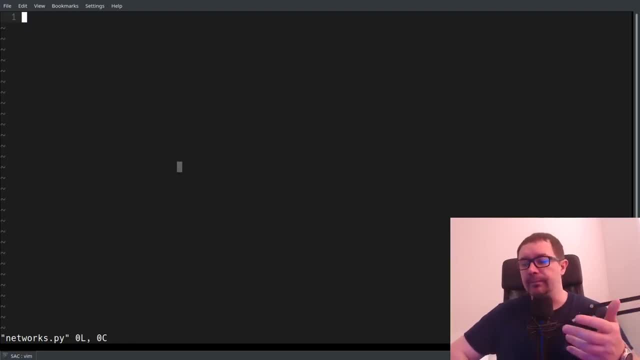 random seeds. How does soft actor critic help us understand this kind of situation? it usually helps us acquire data, So to see that another tool that might help我们可以用这个感应 Wilson的设计让我们能 utveck prizem. 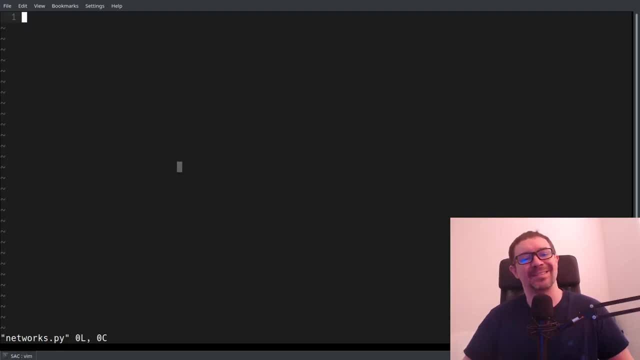 fact that it is maximizing not just the total reward over time, but the stochasticity, the randomness, the entropy of how the agent behaves. As far as the neural networks we're going to need, we're going to need a network to handle the actor, which is the policy, And we're 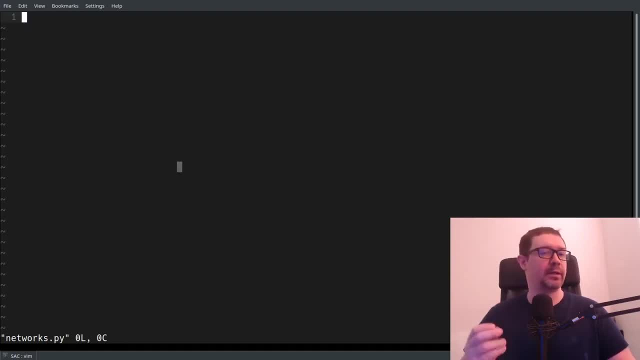 going to be handling how the agent selects actions differently in this particular technique than with respect to something like TDPG or TD3. In those two cases, the neural network output the action directly. In this case we're going to output a mean and standard deviation for a normal 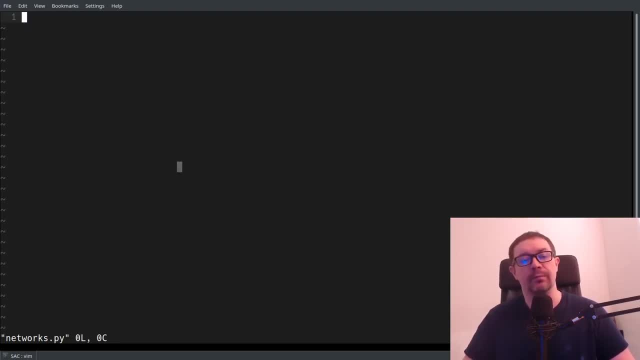 distribution that we will then sample to get the actions for our agent. We will also need a critic network that takes a state and action as input and says: hey, actor, I think the action you took was really good, Or hey, actor, I think that action was terrible. And then we're also going. 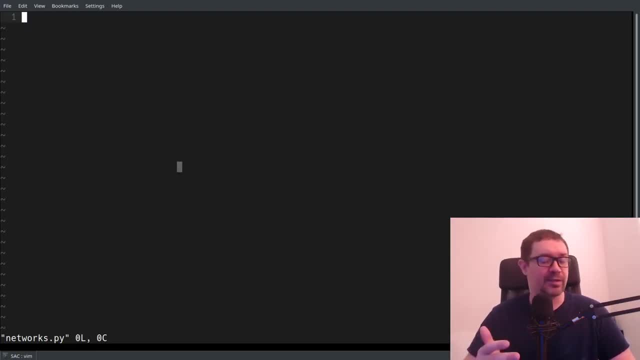 to have a value network that says this state is valuable or that state is not valuable And there will be an interplay between the three to figure out For any given state. you know what is the best action, What is the best sequence of states to 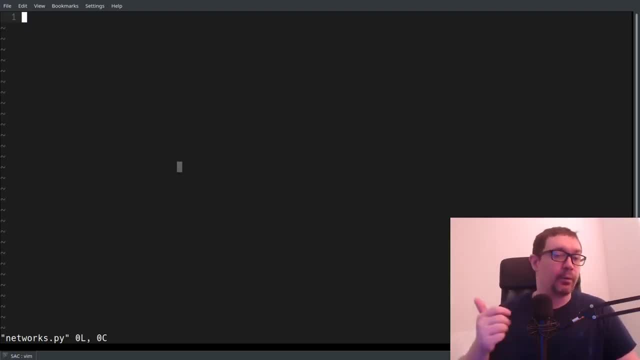 access So you can know what actions to take over time. But we do need three networks and we are going to define those presently. So we will need OS to handle model checkpointing because with the cart pull- excuse me, the inverted pendulum environment- it learns relatively. 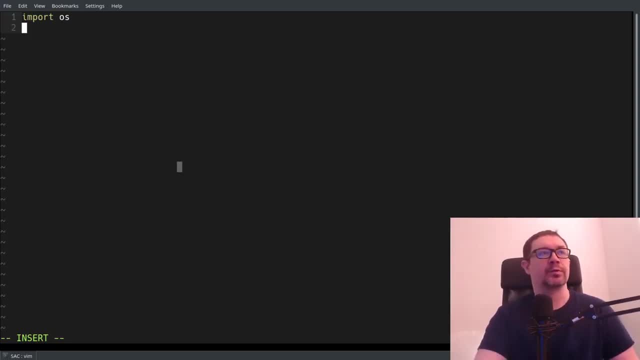 quickly, But for other more complex environments it learns rather slowly. We need torch, We need functional, We need NN for our layers optimizers And we will need our normal distribution as well as NumPy. So we will start with the critic network And that derives from: 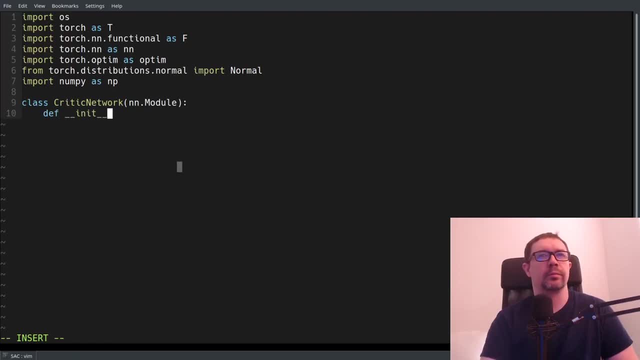 NNmodule. This is just standard fare for PyTorch. We will take a learning rate- I'll call it beta- Number of input dimensions from our environment Dimensions for the first and second fully connected layers. I'm going to go ahead and rewrite things on the fly, So we're going to default these to 256 because 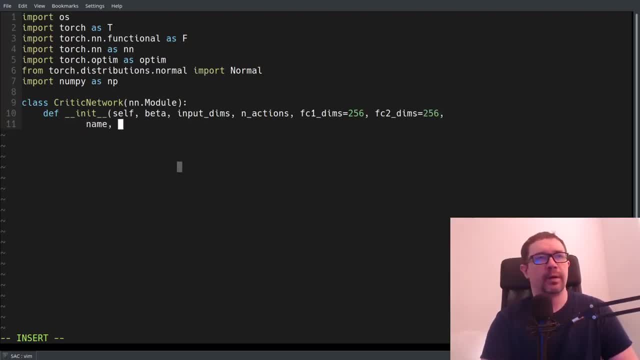 that's what they use in the paper- A name for model checkpointing And a checkpoint directory, And the first thing we want to do is call our super constructor And start saving our parameters. And so we're going to have a checkpoint directory and file for our network that handles model. 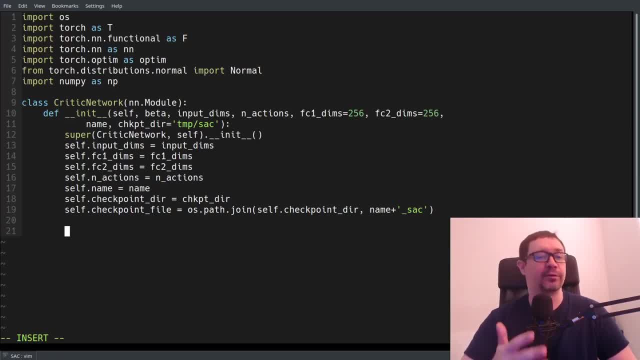 checkpointing, as I said. So we'll have to be very careful to do a make directory before we run the program, Otherwise it's going to complain. The next thing we want to do is define the model- checkpointing, And we're going to call our super. 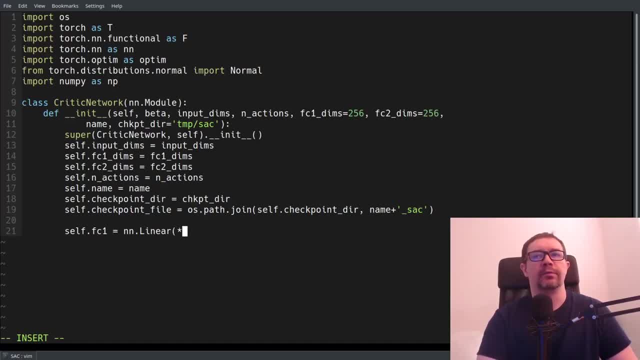 constructor And we're going to define our neural network And that will take input dim sub zero plus an actions as input And again. so, if this is mysterious to you, the reason we have to do this is because the critic evaluates the value of a state and action pair, And so we want to incorporate the 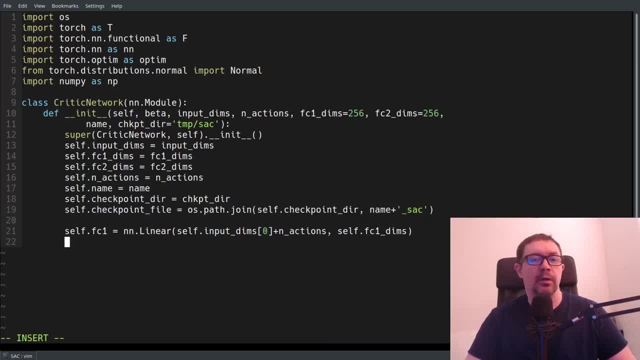 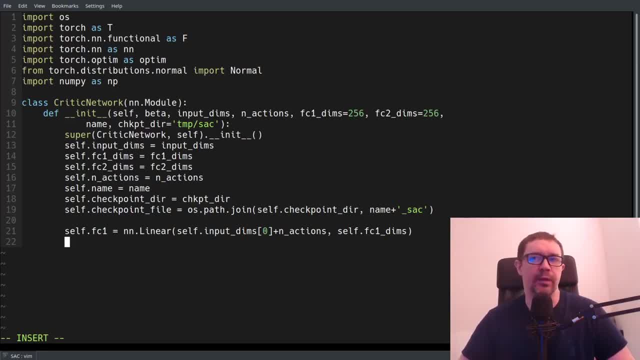 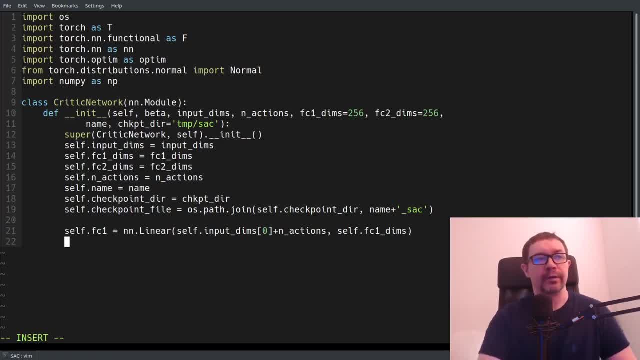 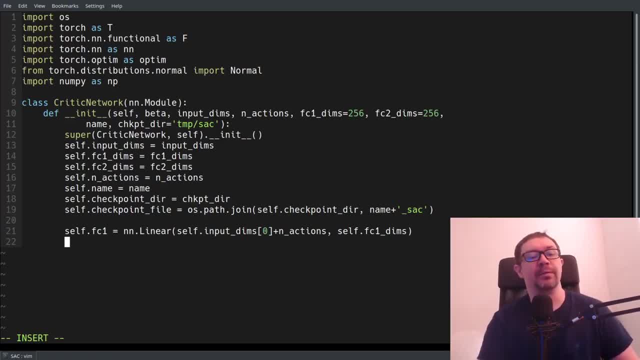 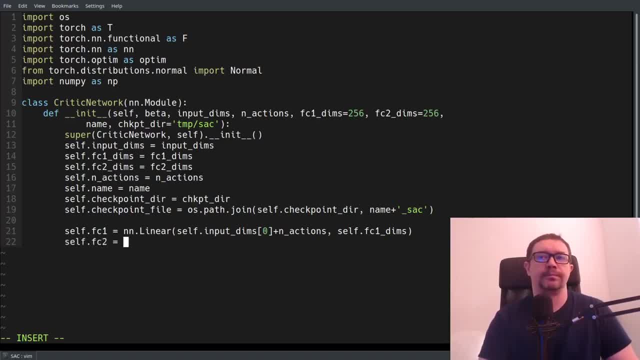 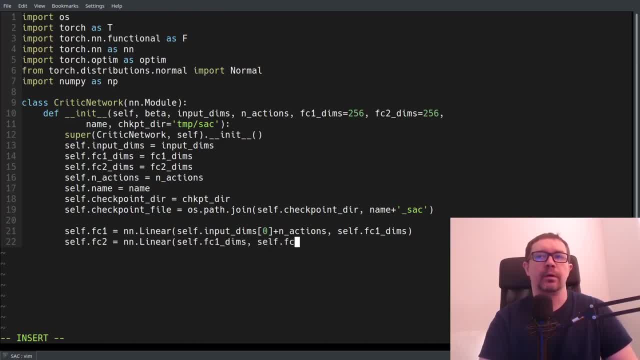 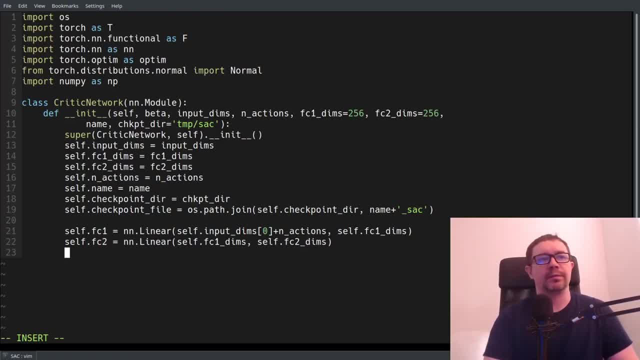 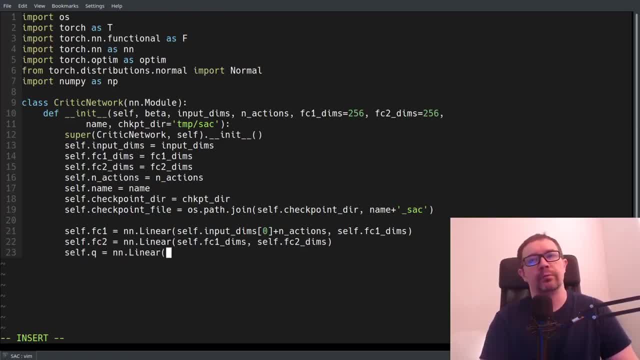 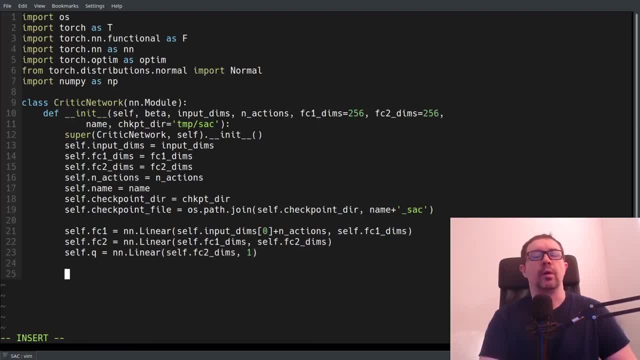 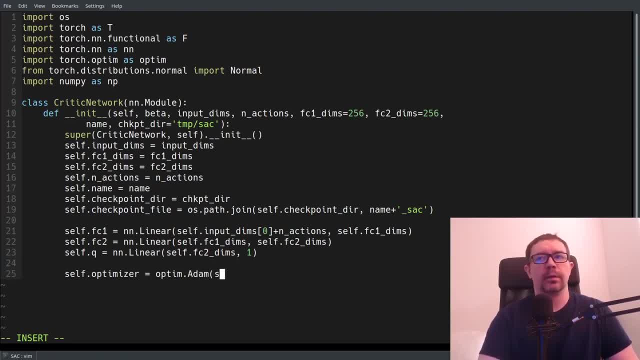 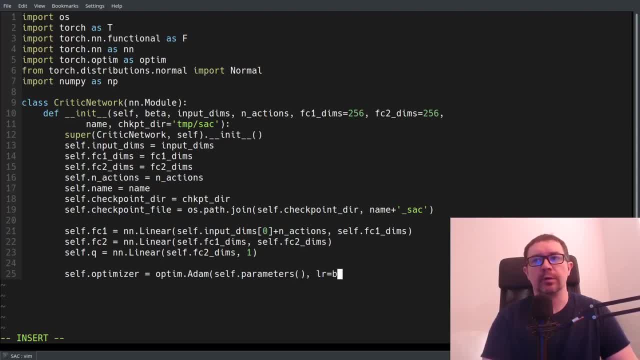 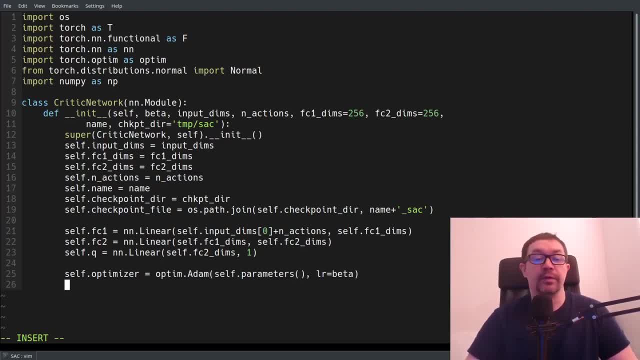 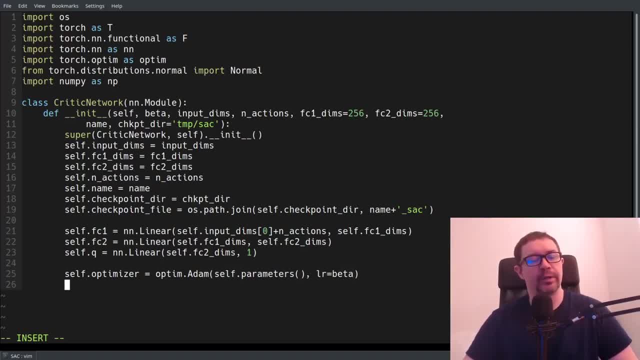 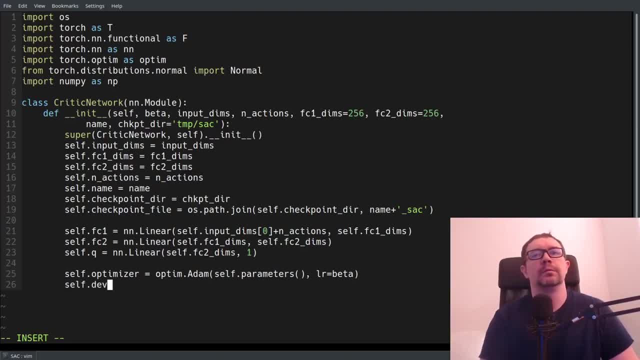 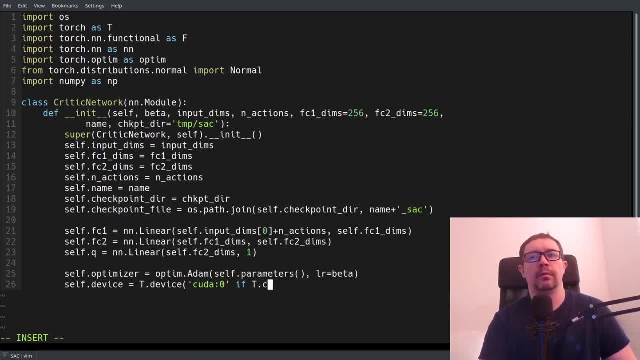 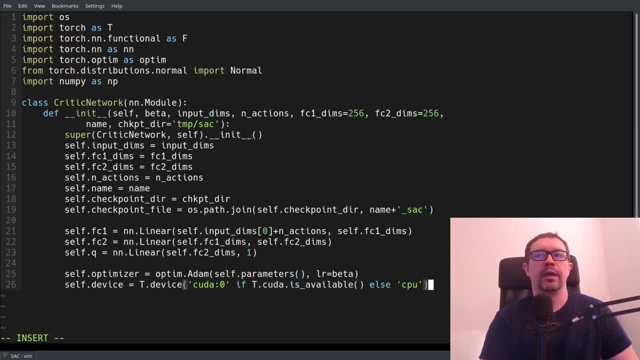 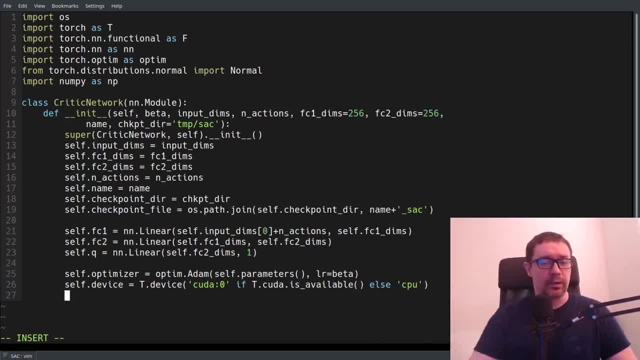 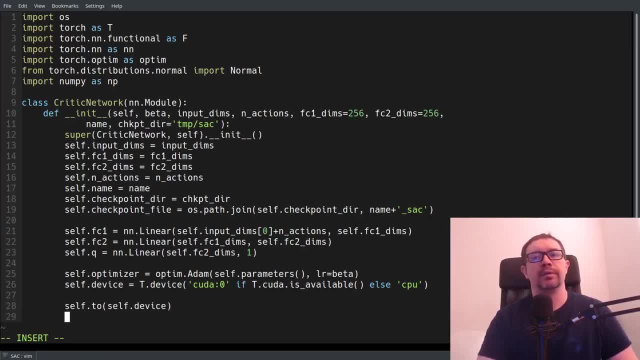 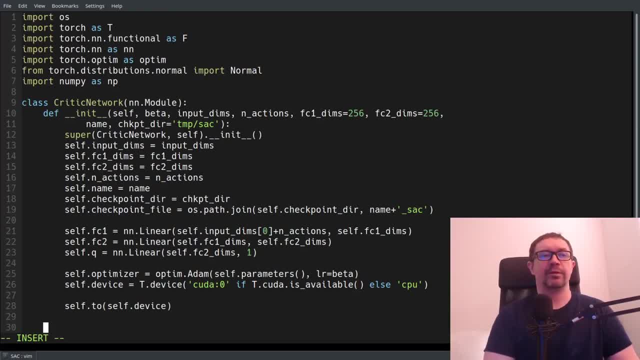 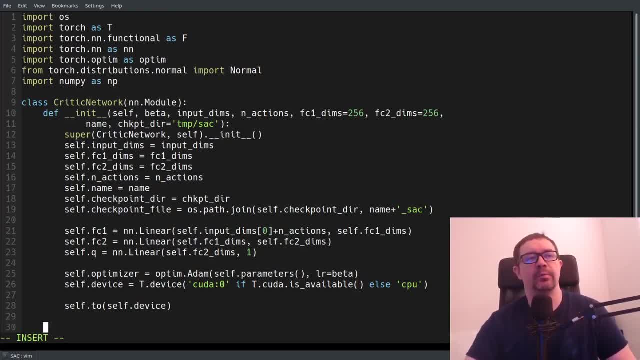 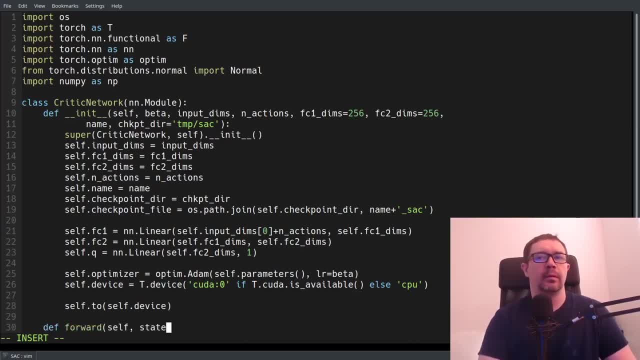 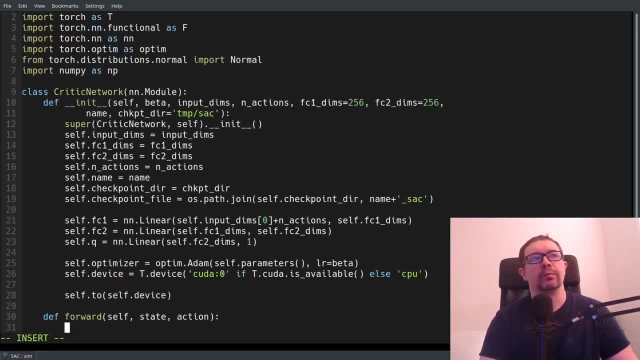 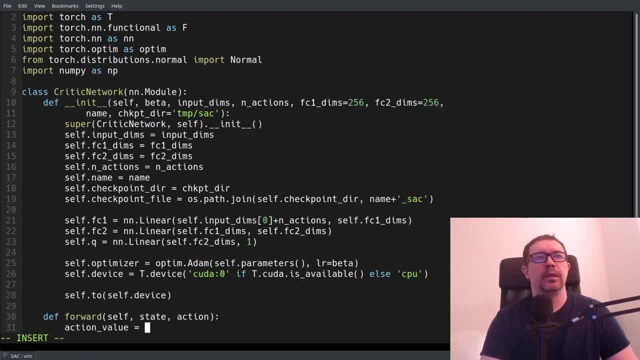 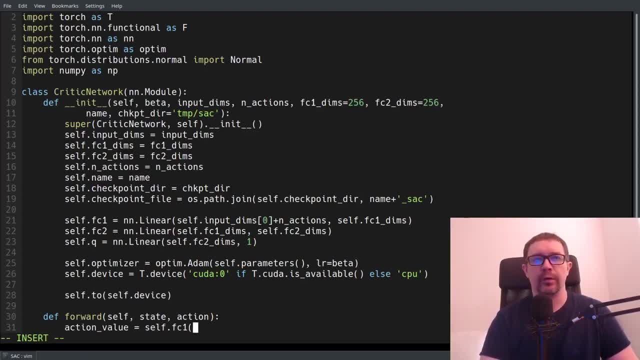 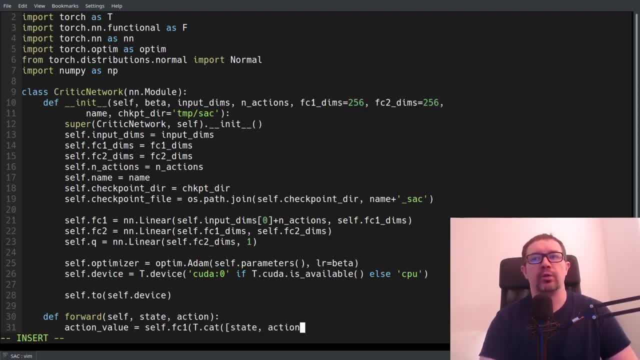 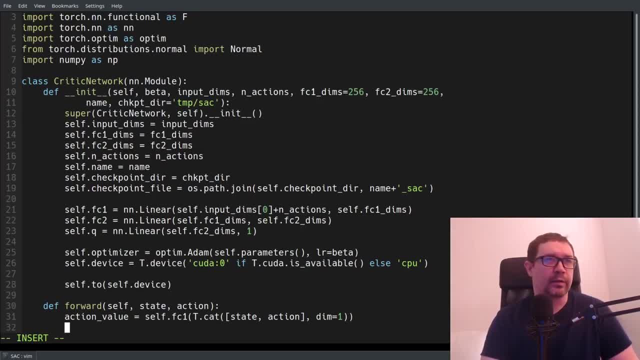 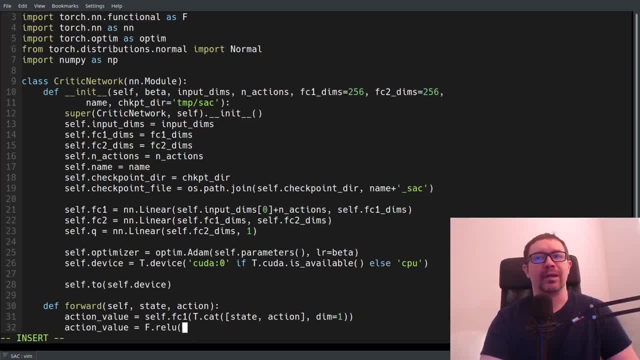 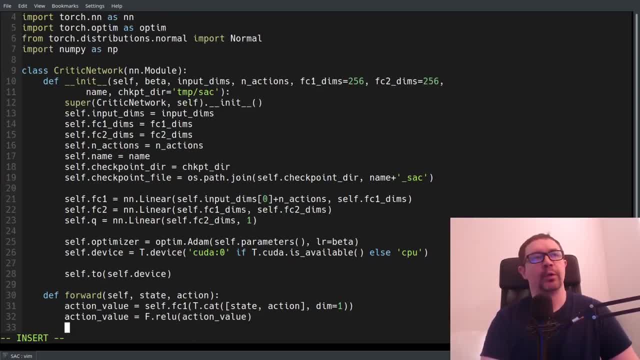 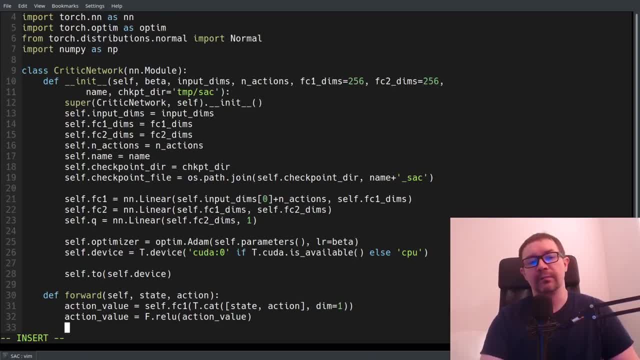 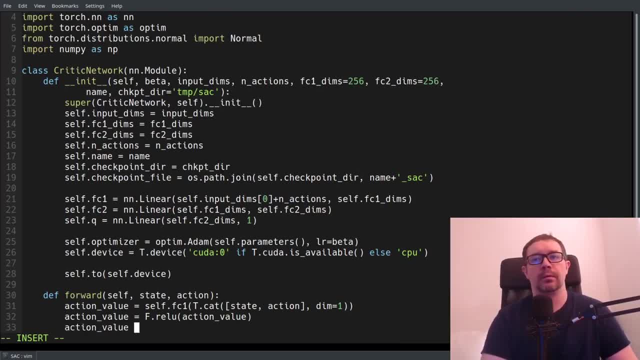 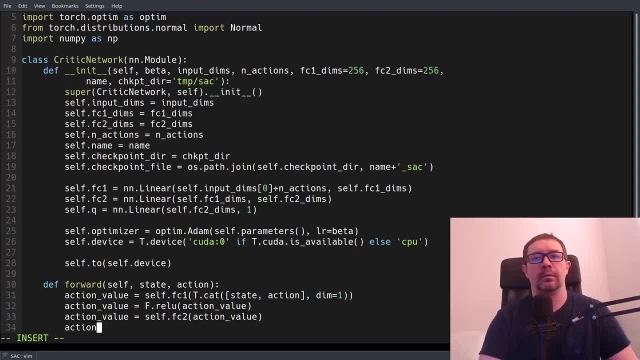 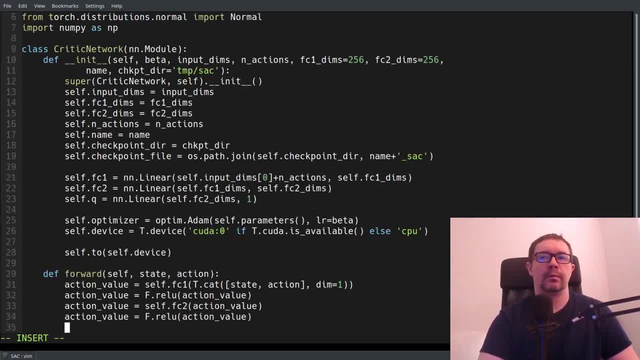 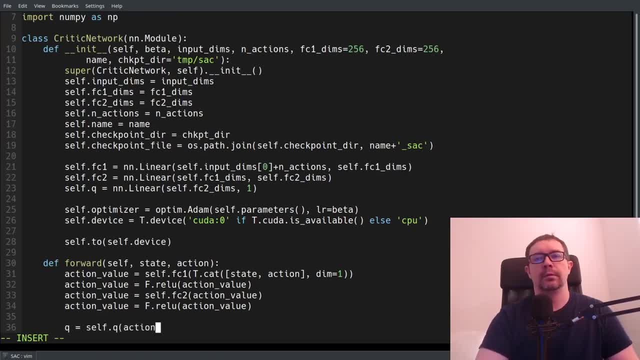 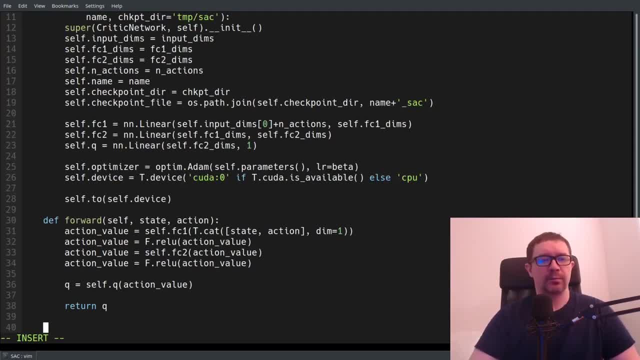 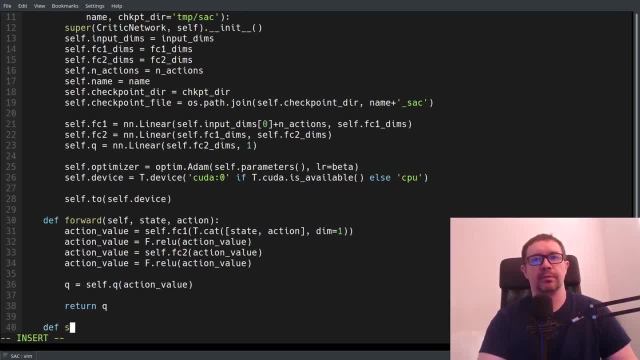 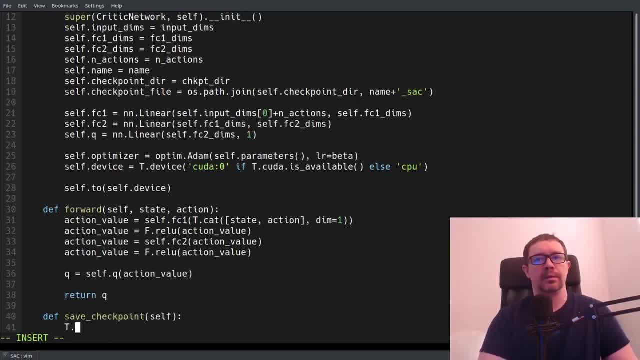 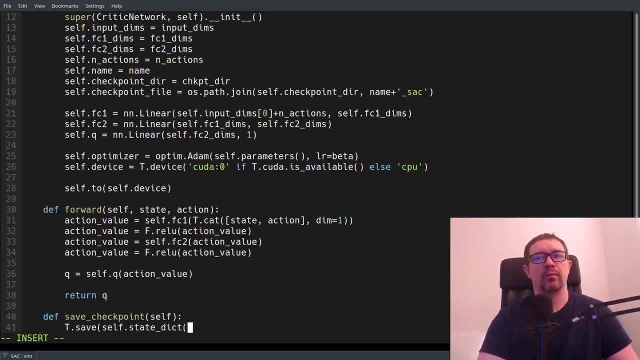 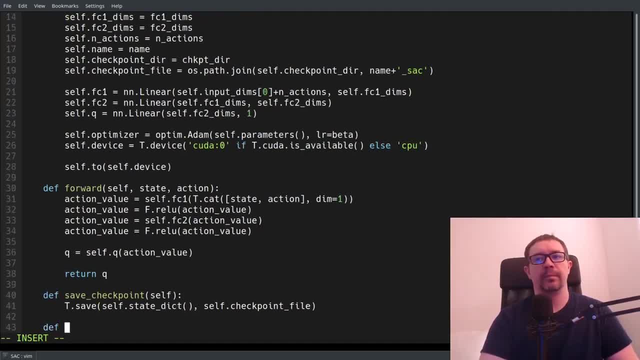 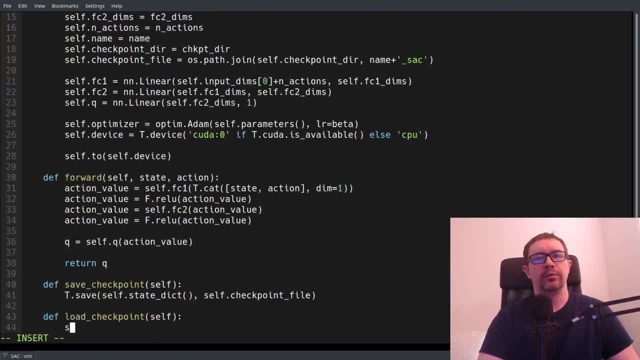 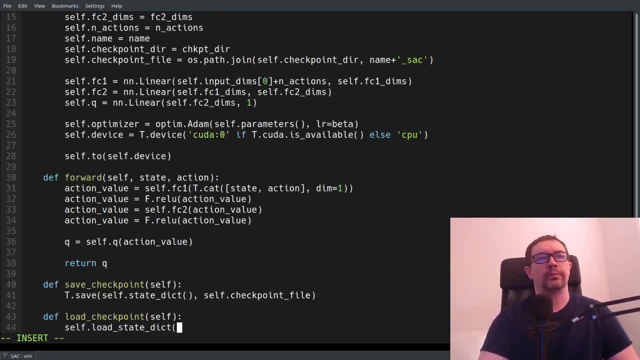 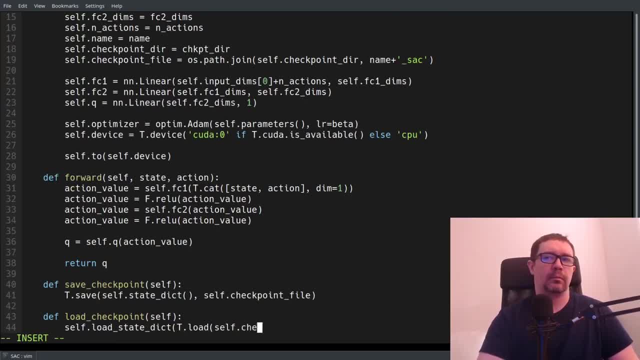 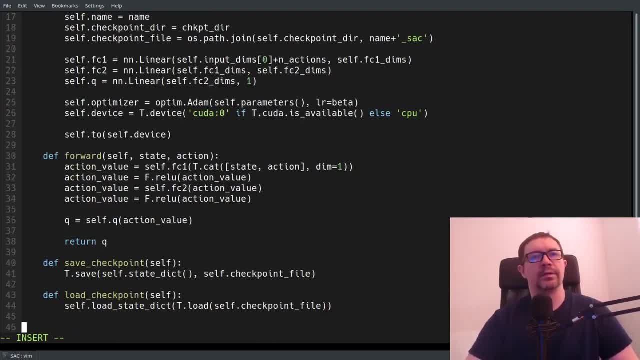 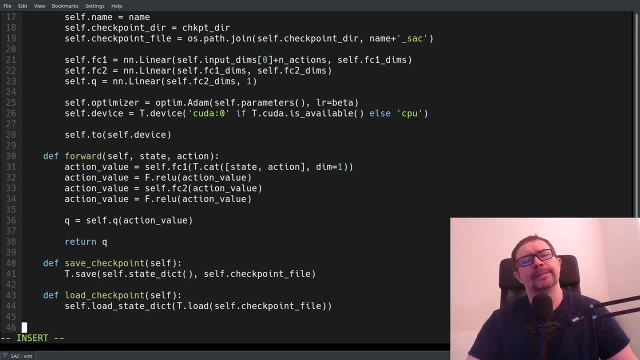 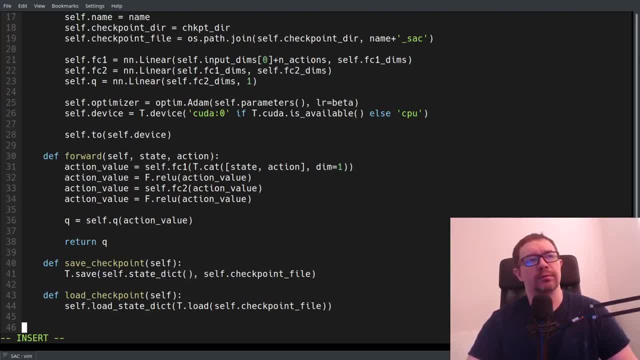 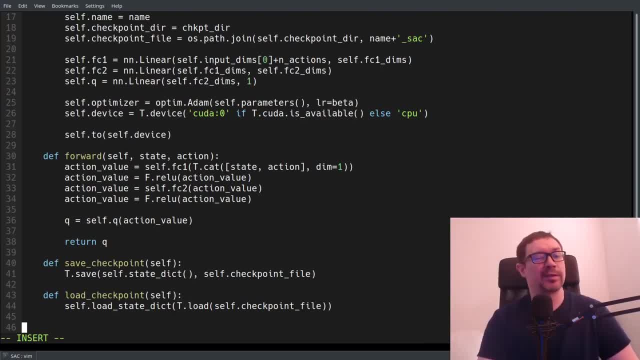 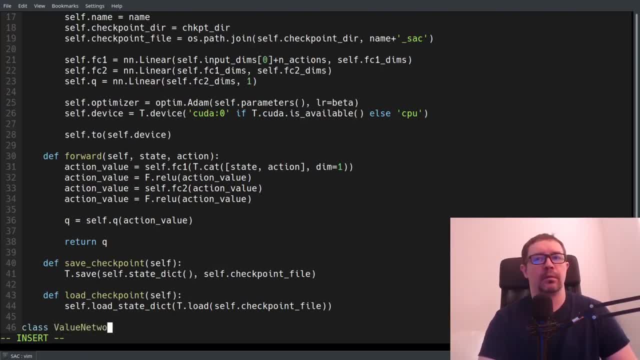 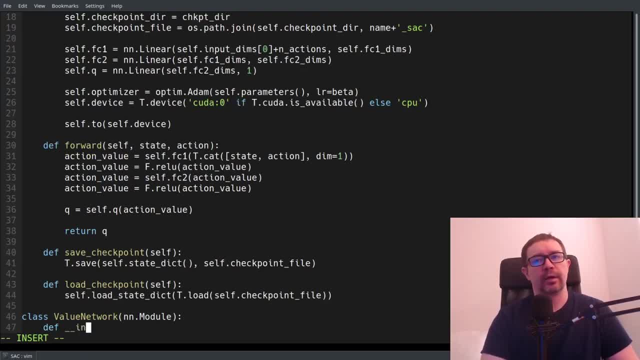 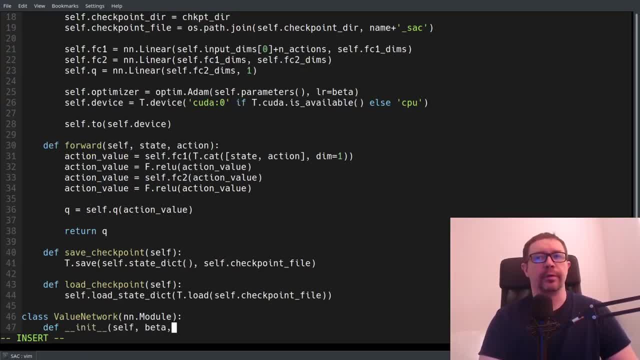 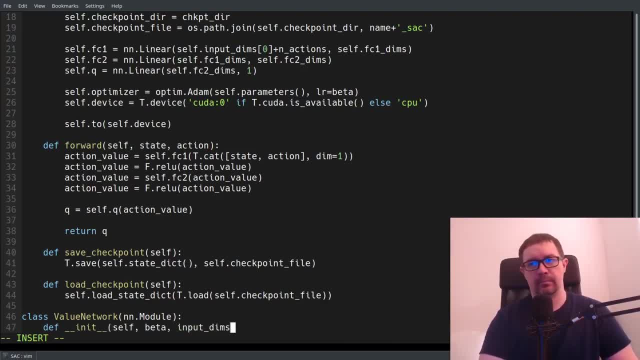 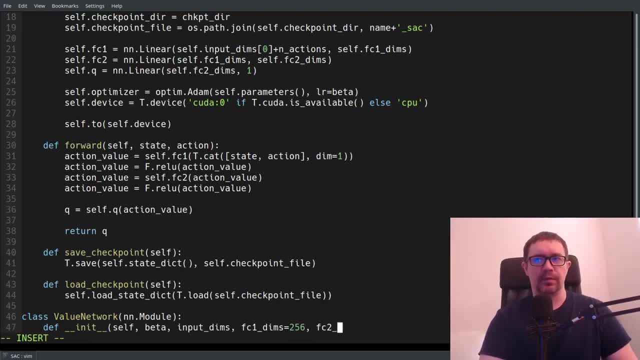 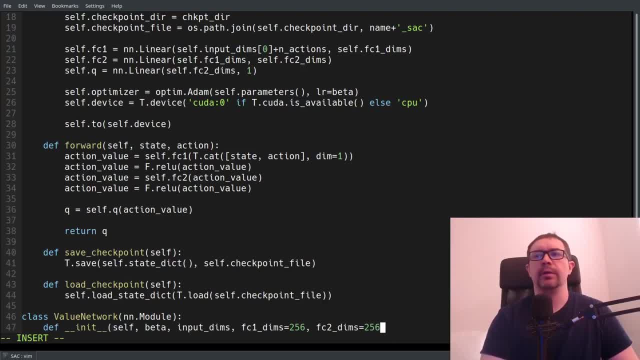 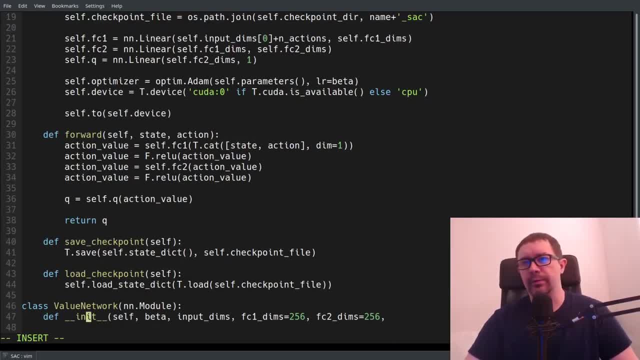 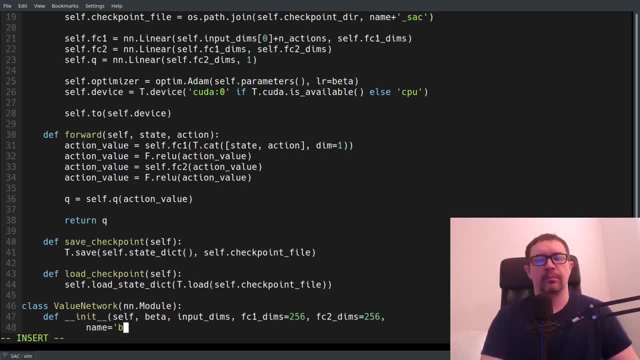 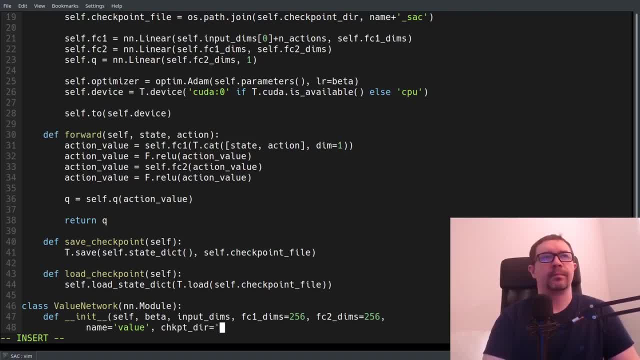 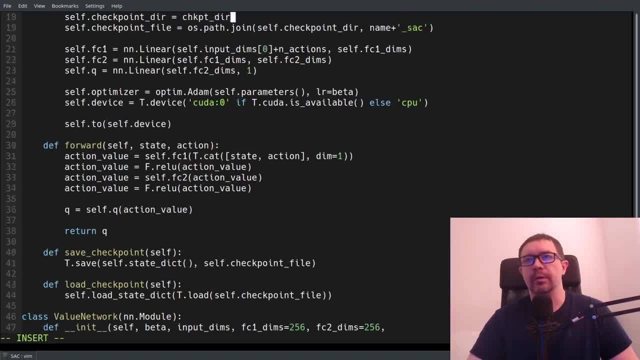 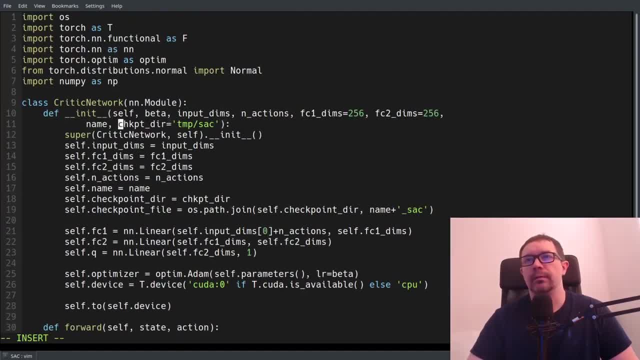 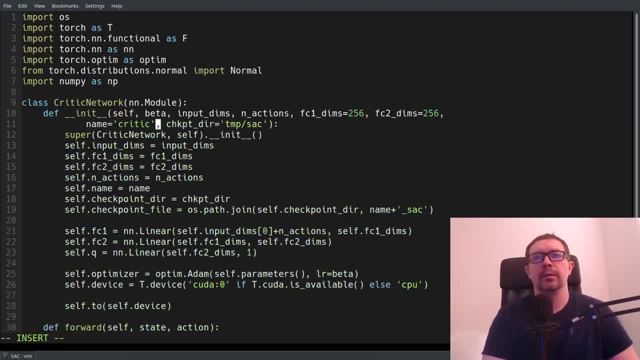 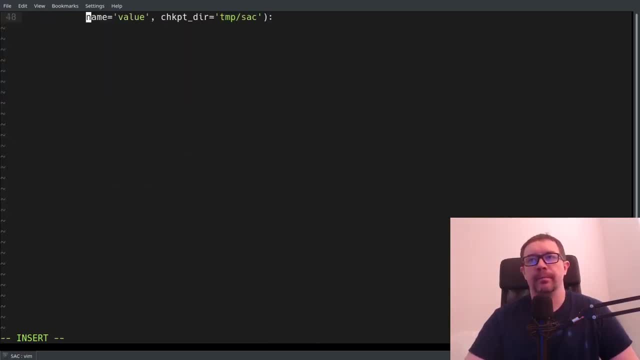 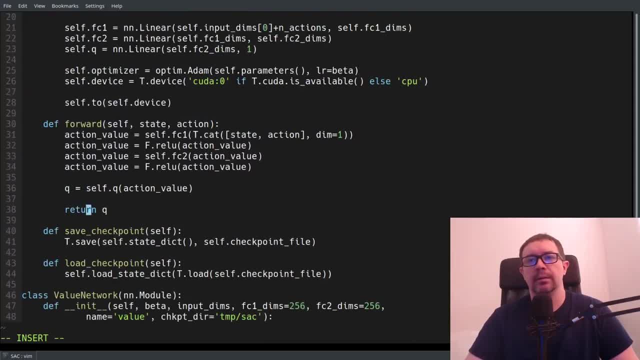 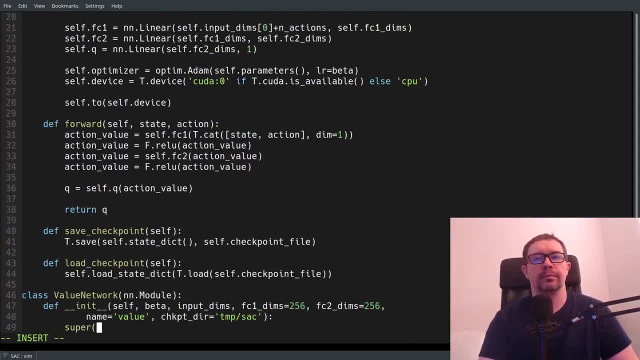 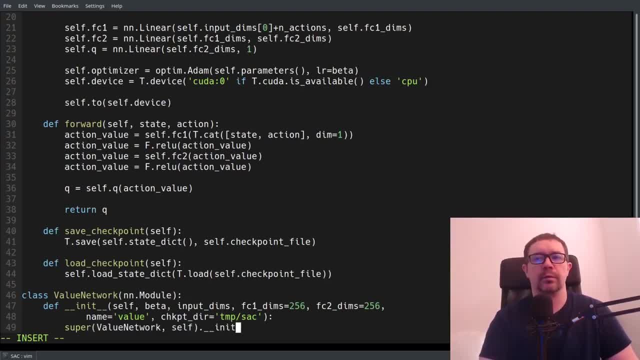 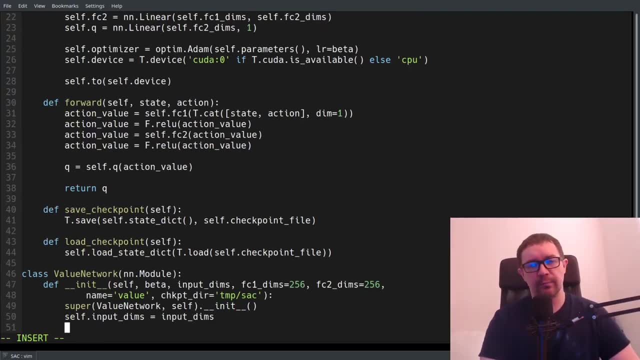 constructor, And that's it. So we're going to call our super constructor, And that's it. So we're going to call our super constructor, Of course, And we don't need the number of actions here, because the value function just. 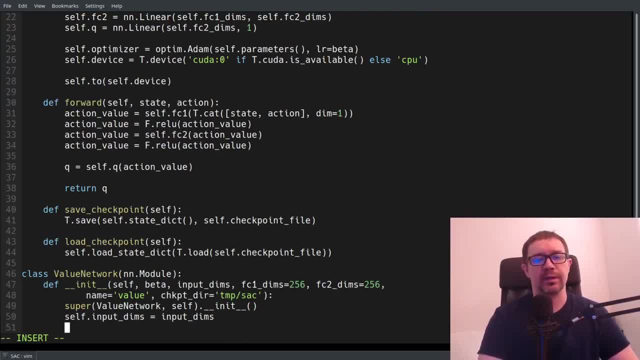 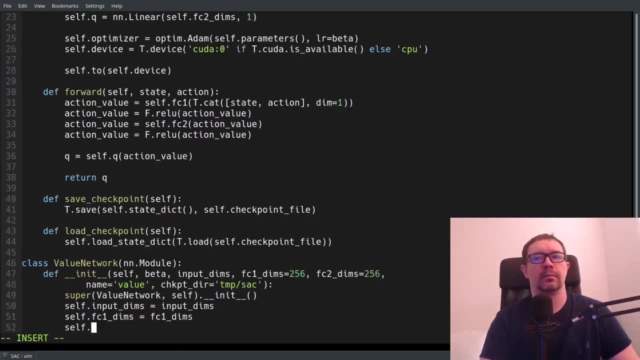 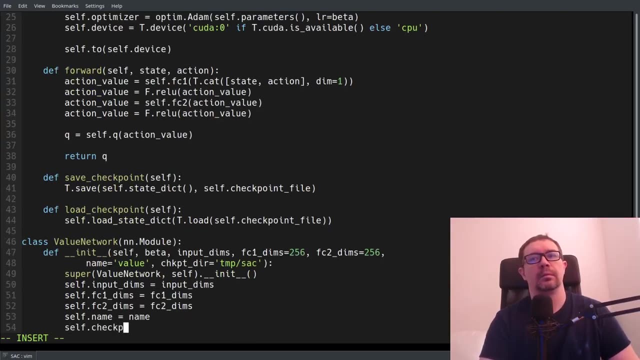 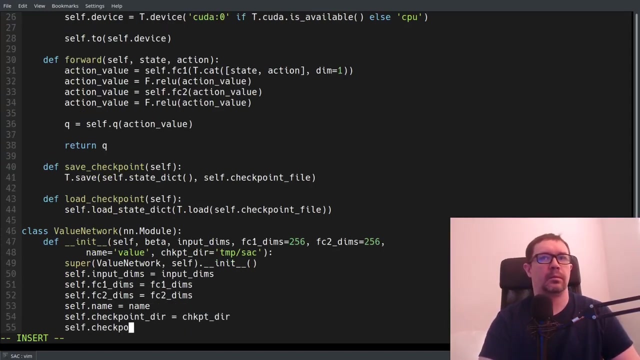 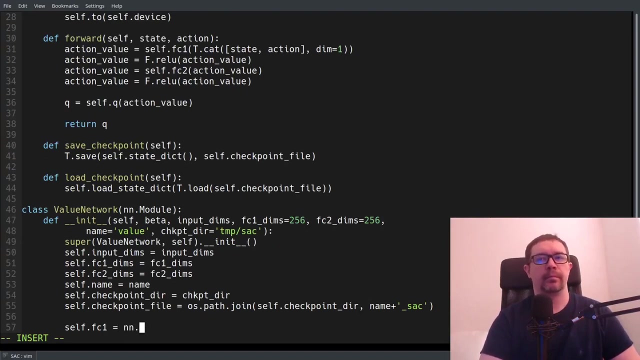 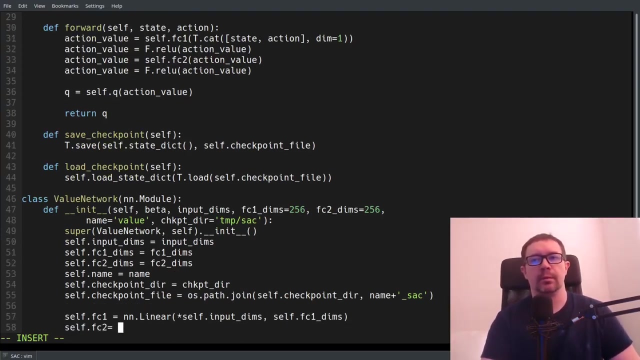 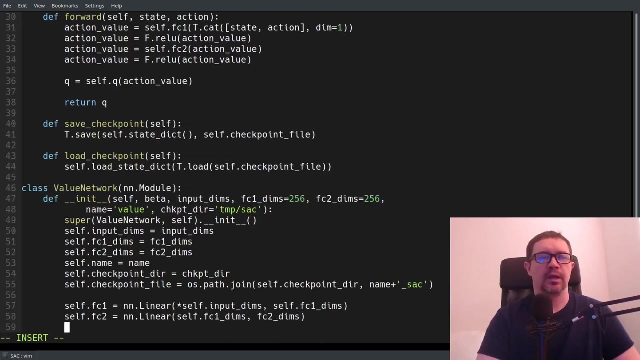 estimates the value of a particular state or set of states. it doesn't care about what action you took or are taking. Then we have our network, and that's just a very simple neural network. We're going to go from input DIMMs to FC1 DIMMs, second connected layer, and an output. 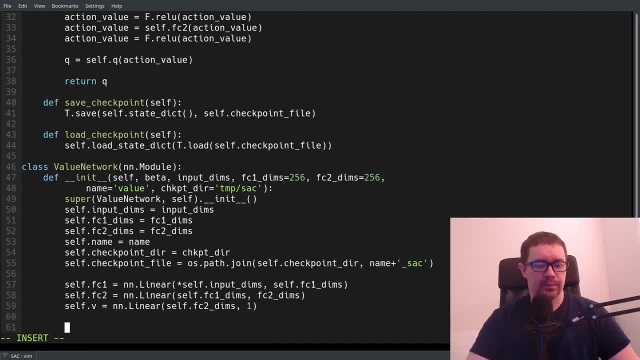 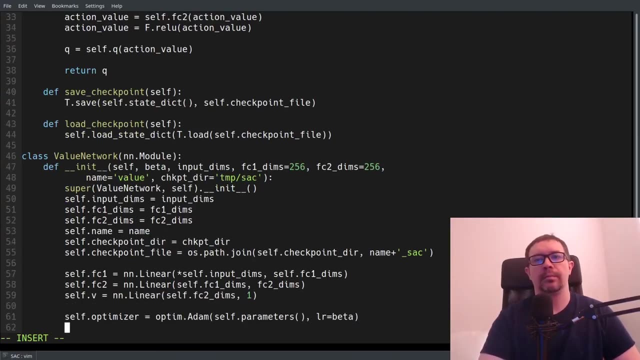 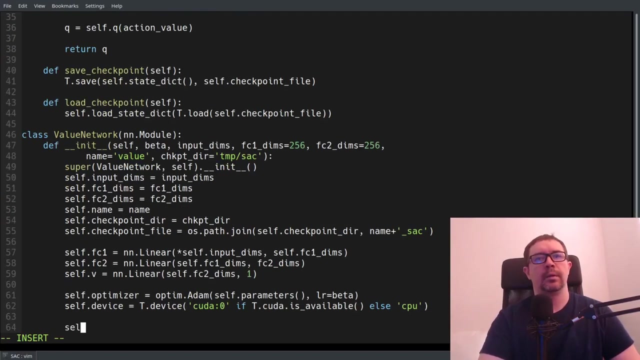 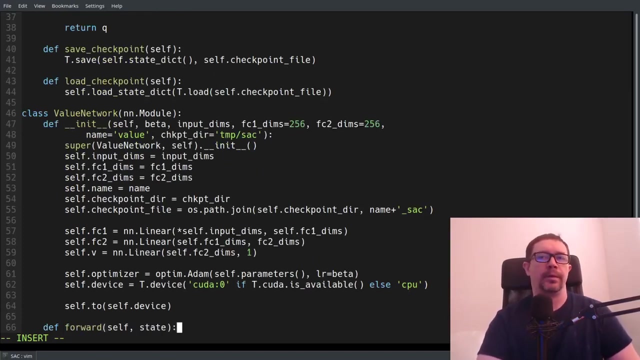 layer And that'll be a scalar quantity, so it's just FC2 DIMMs by one, And of course we also need an optimizer and device. So we'll go through this network as well And then we'll send everything to the device. 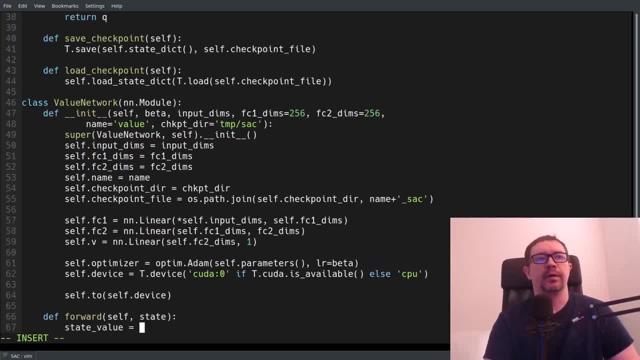 The feature is that we can also send data to the device, And then we'll send everything to the device. The feature is that we can also send data to the device. So the straightforward function is pretty straightforward: We want a state value And then we want to activate it. 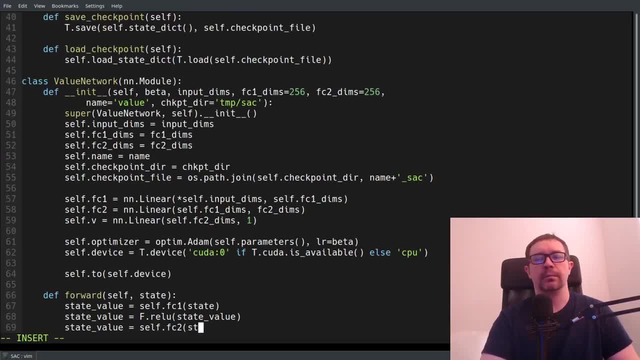 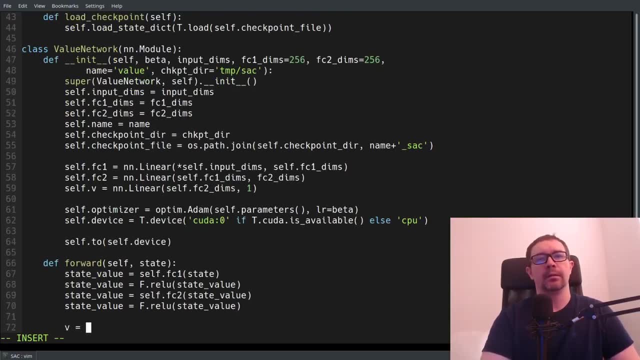 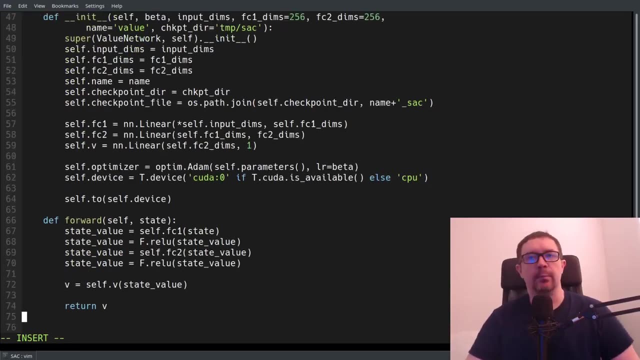 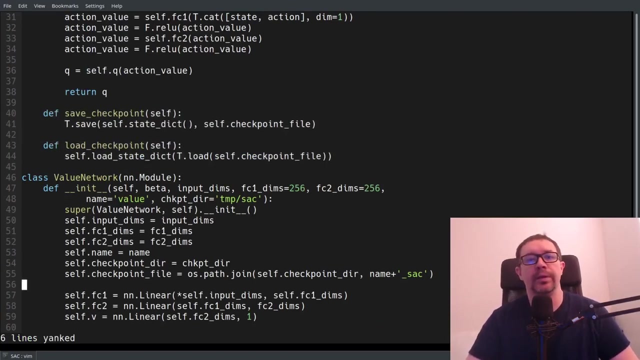 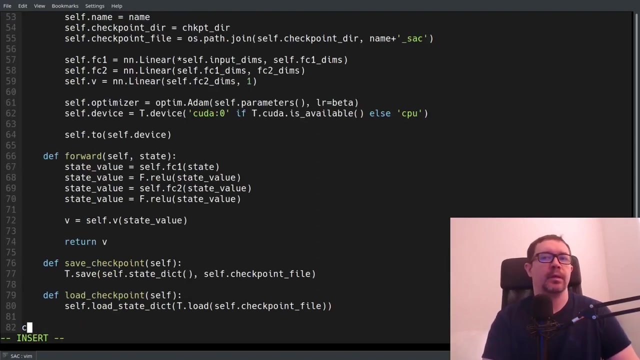 And pass it through our second fully connected layer, Activate it again- We got our output And return it. And then we also want save and load checkpoint functions. I am going to copy and paste those, Because that is just significantly easier. And then we want the actor network. 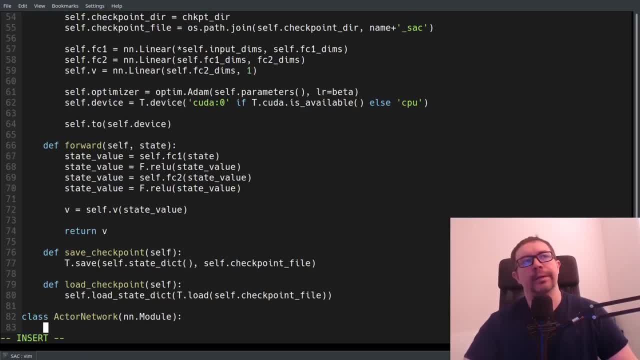 Now this is the relatively hard part of the problem, because we're going to have to handle sampling and probability distribution instead of just doing the actual distribution. So we're just doing a simple feed forward. So we're going to start with our initializer, of course. 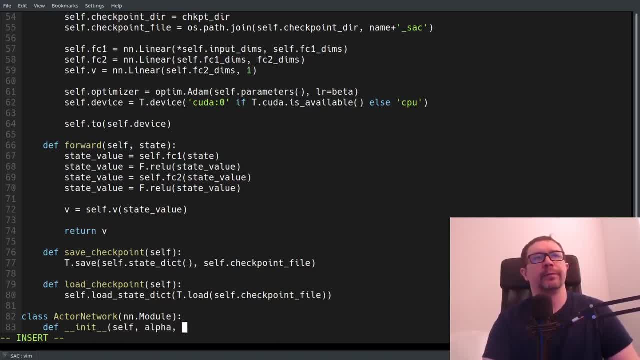 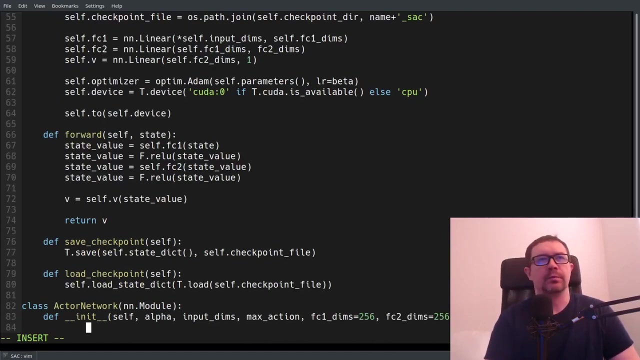 It takes a learning rate, alpha input, DIMMs. I'm going to default this to what we use in the paper, Max action. Let's not give that a default value. We will also give it a default value. We will also need a num actions, a name and a checkpoint directory. 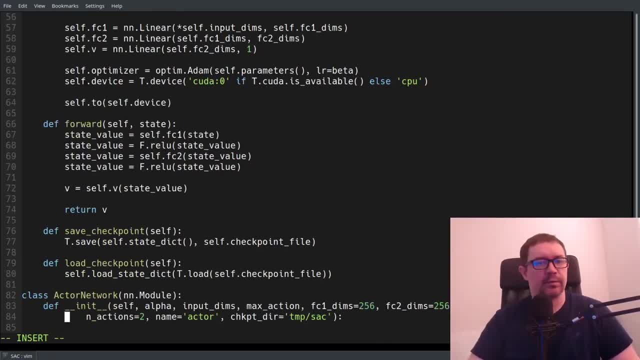 Now the point of the max action. Now, sorry, this stuff is a little bit hard for you to see, isn't it? Because of my ugly mug. So the point of the max actions is that the deep neural network is going to be constrained. 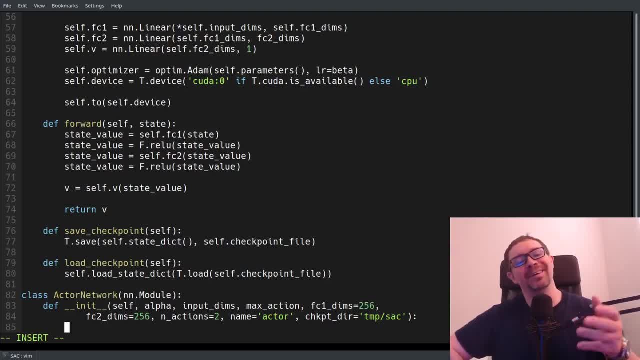 Or rather R2.. So these action function, or sorry, our policy sampling is going to be restricted to plus or minus one with a tangent hyperbolic function, But in an environment may very well have an action bound that is greater than that. 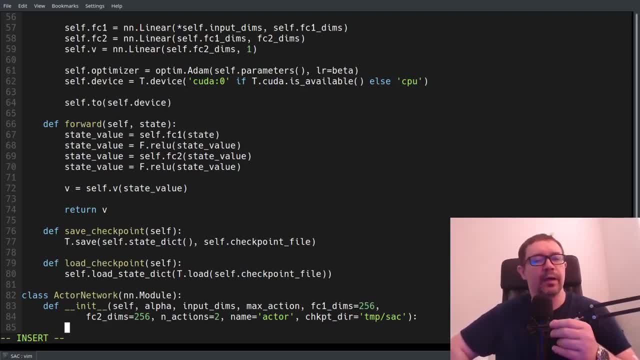 It may have an action bound of two or three or five or whatever, And so you want to output a. you want the output of the deep neural network, of the sampling function to be multiplied by the max action, So that way you get the appropriate range of actions for your environment. 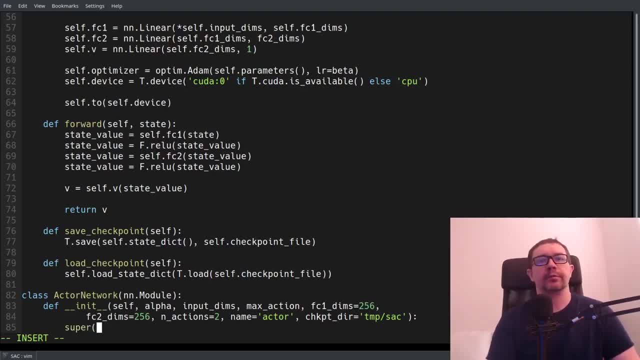 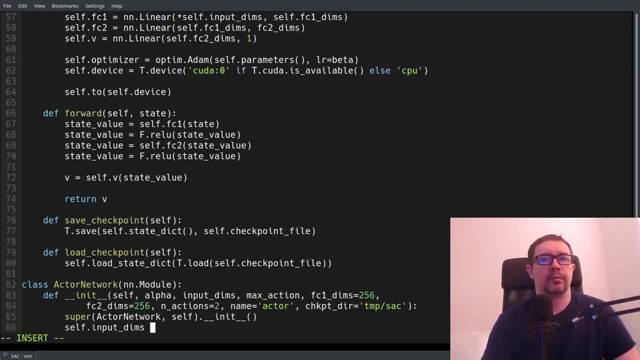 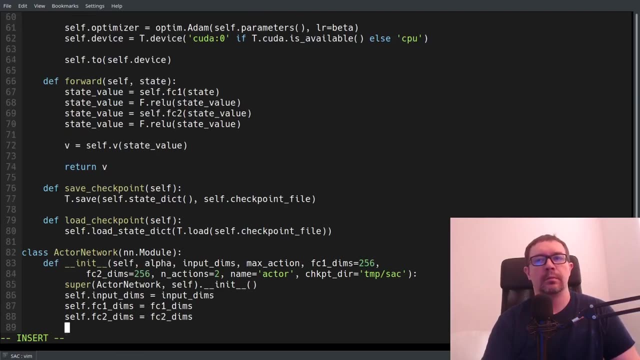 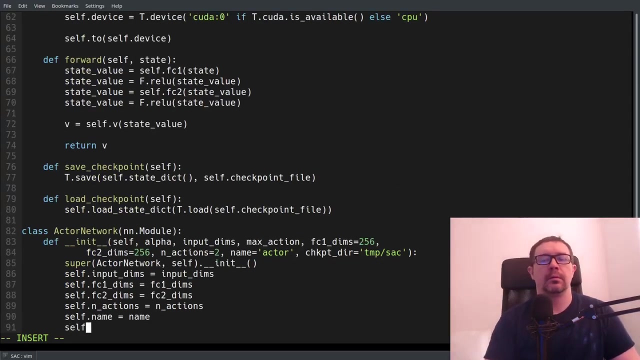 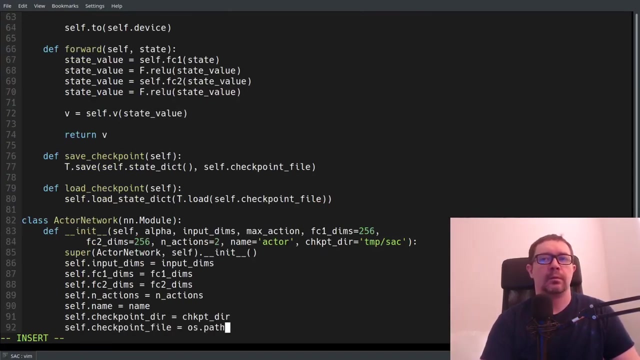 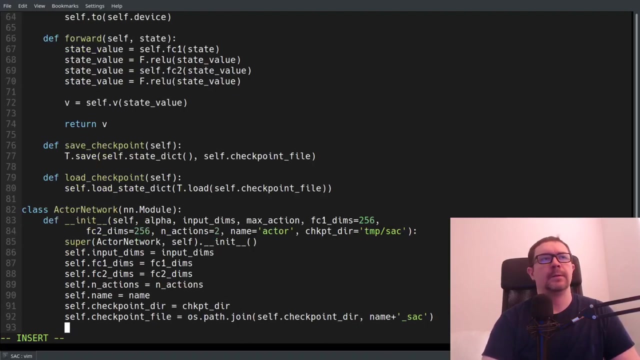 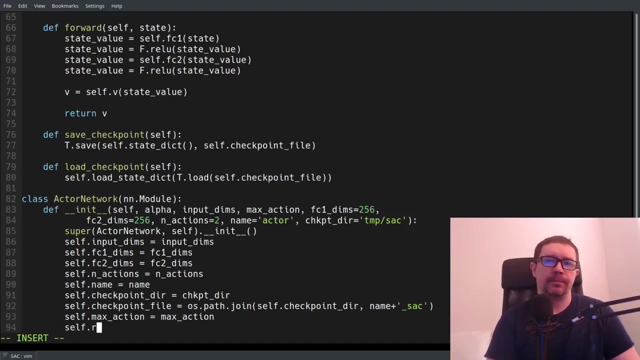 So we will call our superconductor. So we will call our superconductor. So we will call our superconductor And save our variables. We're going to need number of actions, we need our max action and, oh, we also need something called re-parameterization. noise now. 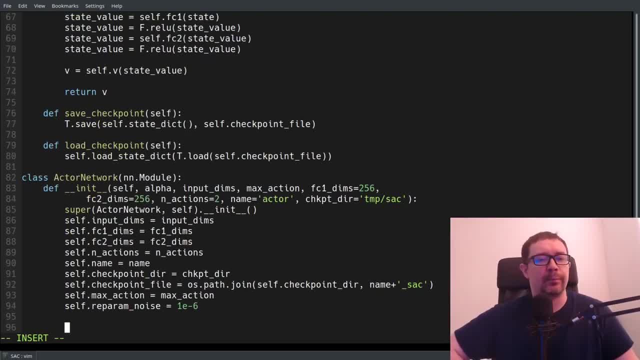 the need for the re-parameterization noise will be a little bit more apparent when we handle the calculation of the policy. it's going to be there to serve a number of functions. first of all, it's going to make sure that we don't try to take the log of zero, which is undefined. that'll break the. 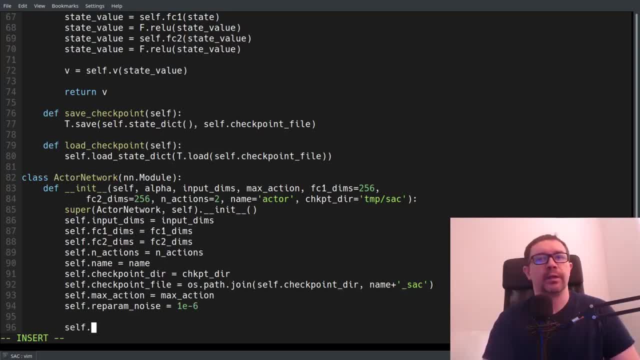 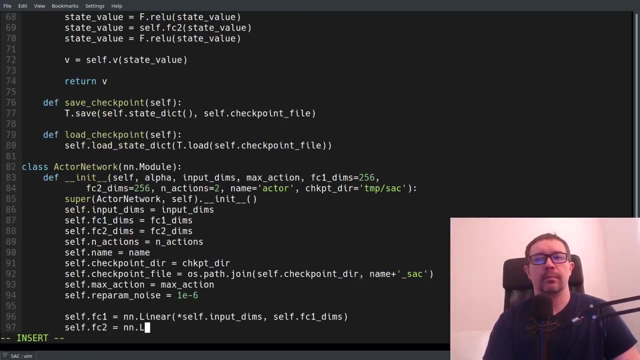 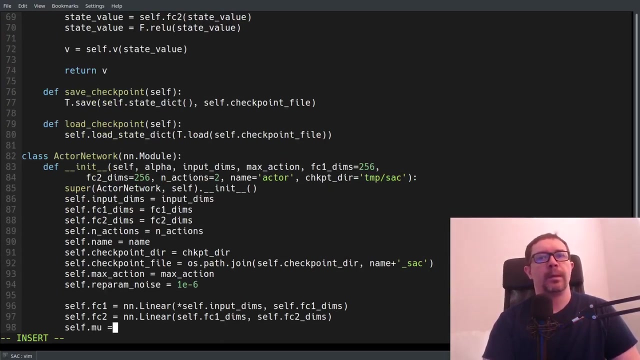 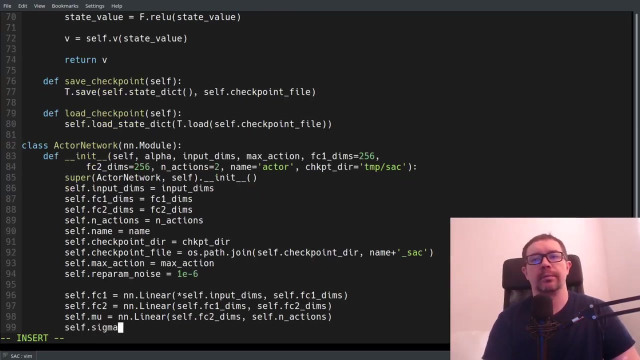 software. so we need a noise factor for that. but first let us define our deep neural network input, DIMMs, by SC1, and then we have two outputs: a mu, which is going to be the mean of the distribution for our policy, and that will have as many outputs as we have components to our actions, and a standard deviation. and then 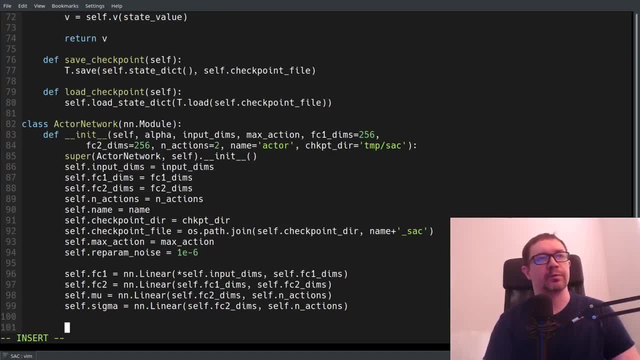 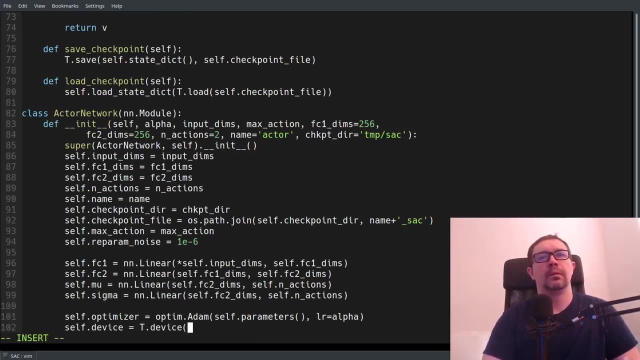 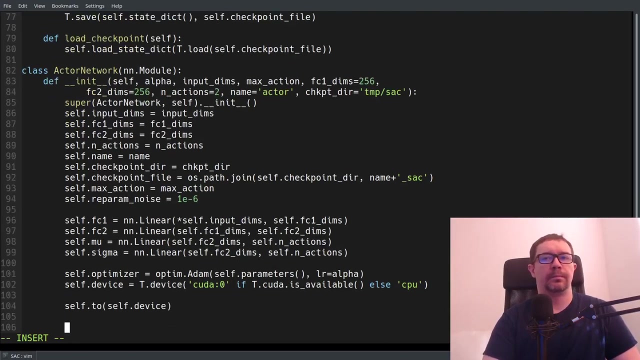 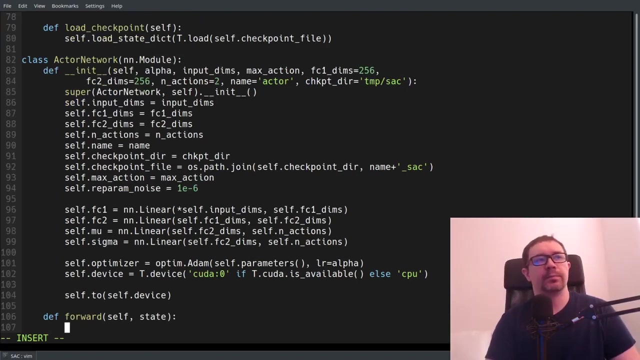 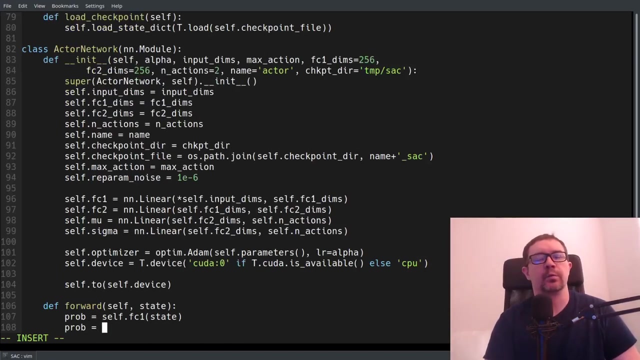 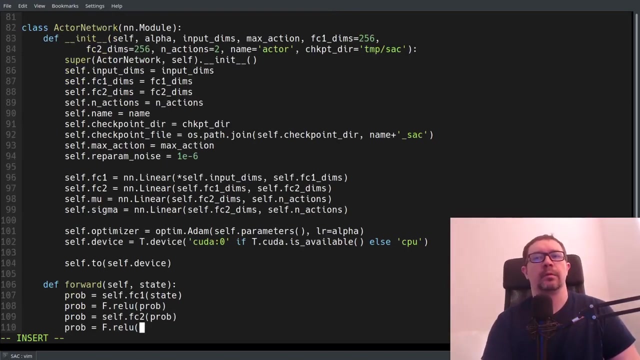 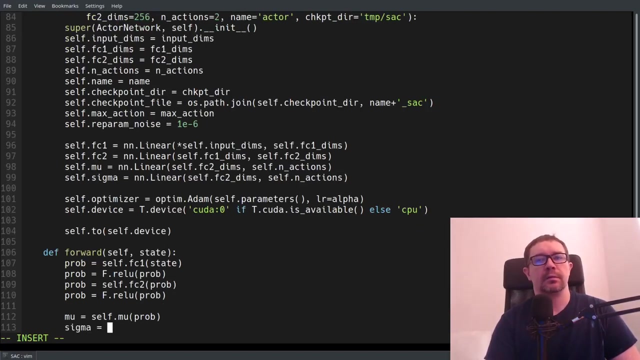 again, we need an optimizer and device and to send the network to the device now. so we have some a desease. next we handle our feed forward with mistakes. a word state as input and I'm gonna call it prob for probability. it's kind of a misnomer, I suppose, but sue me. and then we'll say mu is that, and then we have to. 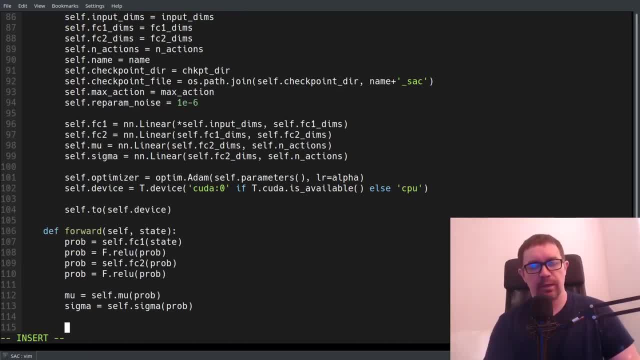 do something a little bit mysterious. it makes sense if you think about it. the next step is to clamp our Sigma, and the reason is: you don't want your distribution, for your policy, to be arbitrarily broad. right, the standard deviation determines the width of your distribution. effectively, right the mean. 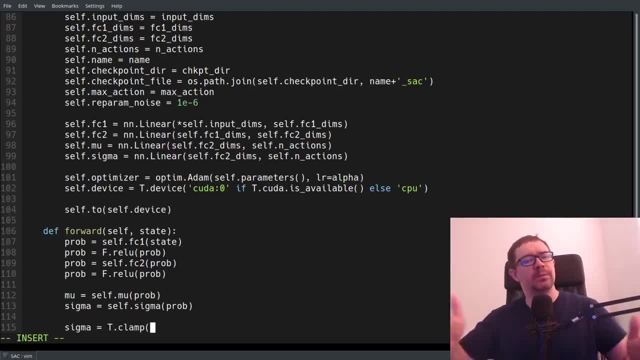 is the center point and the standard deviation is its width. you don't want that to be really, really broad. you want that to be some finite and constrained value. now the authors of the original paper. if you take a look at their code, they use a clamp, which makes a lot of sense because it's computationally cheap, but they use 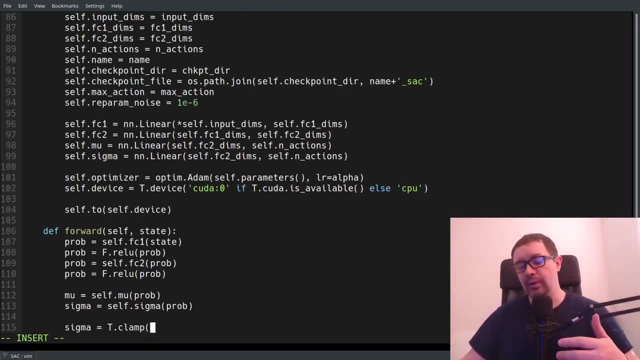 of a lower end of minus 20 and a higher end of positive 2. now I don't know how they came about that I'm certain it's just a consequence of experimentation. but if you use a negative value for your standard deviation or, sorry, a negative, 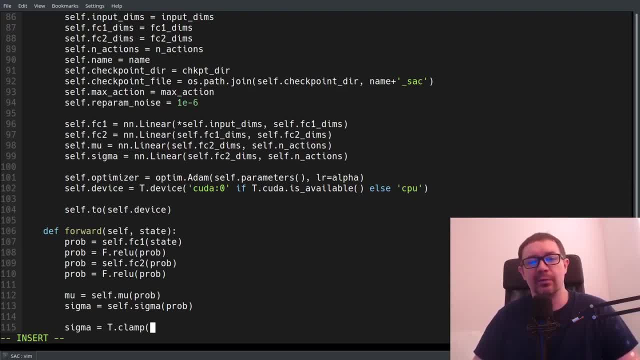 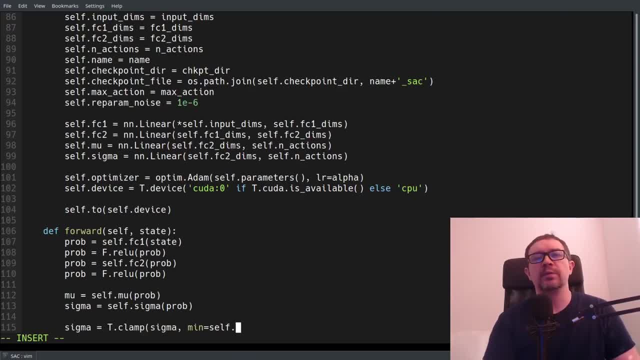 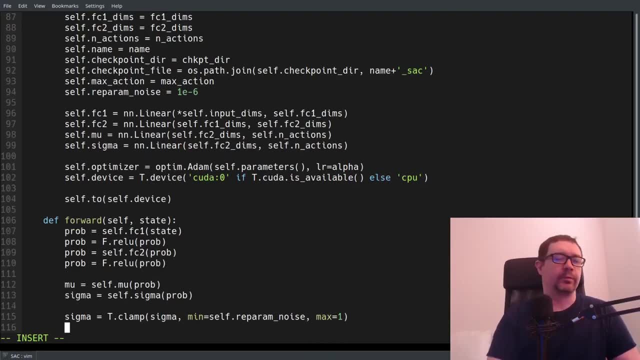 you're going to get a sigma of 0, so you're going to get a sigma of 0, so you're going to use a very small number, which is the reprogram noise, 1 by 10 to the minus 6 and a max of 1. so between 0 and 1 you can also use a sigmoid function. 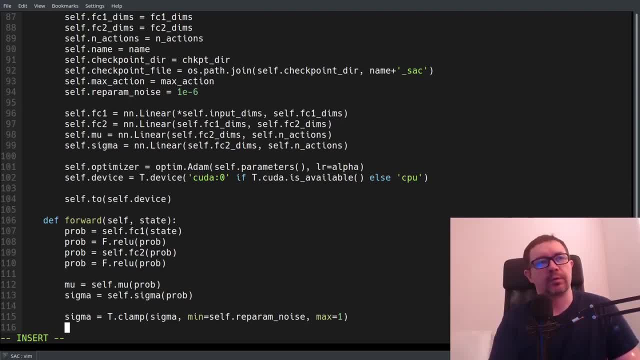 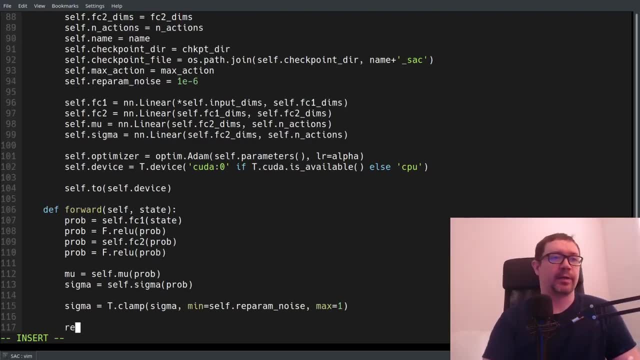 here to have a nonlinear activation between 0 and 1, and that works just fine. the issue is that it's a little bit slow in terms of computational speed, so the clamp is much faster, and this is already a computationally expensive algorithm, so I make the the optimization to use. 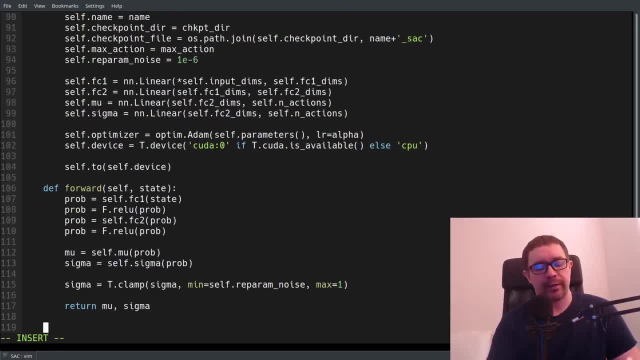 the clamp function. so then, once you have calculated them, you want to return the mu and sigma and the next we have to handle the calculation of the actual policy. now, if you're new to deep reinforcement learning, a policy is a probability distribution that tells you the probability of selecting any action. 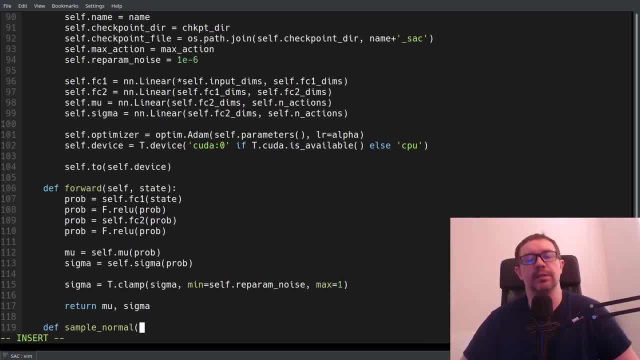 in your action space, given some state or set of states. so you're in some state. you have some available actions. what's the probability of choosing each? if you have a discreet interpretation of the action space, then you're going to have a discrete environment. it's, excuse me, an environment with the discrete action. 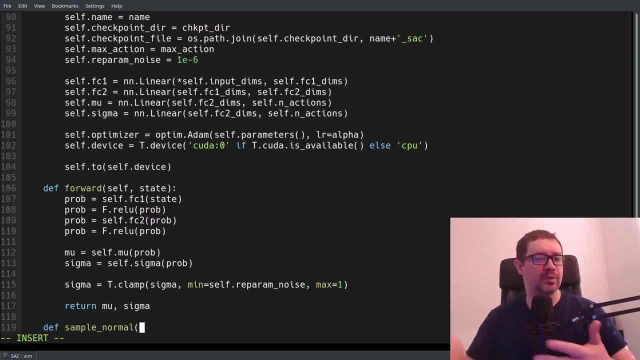 space, then it's pretty simple: you just assign some probability to each of those actions and it's a discrete probability distribution. but if you have a continuous action space, then we need some sort of distribution like a Gaussian, in this case a normal, which is how we're going to handle this, and we 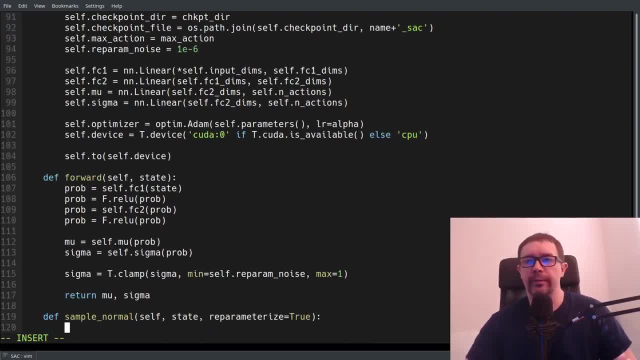 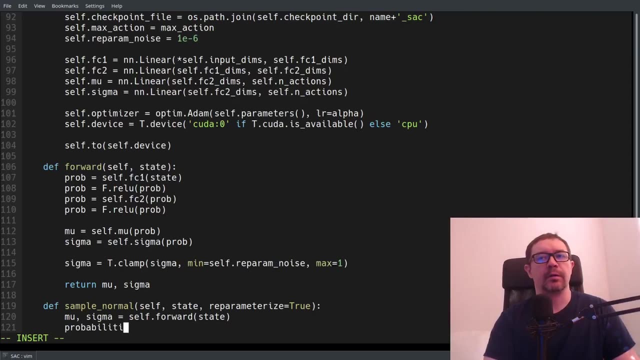 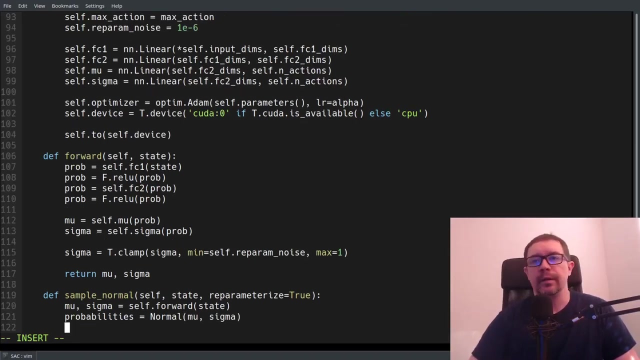 have some parameter here called re-parameterize. don't worry about that too much. I go more in depth on that in the paper because it's a trick. the don't worry about that for now. it's not something to be overly concerned about. it just changes something down here. so we want our actual distribution, that is. 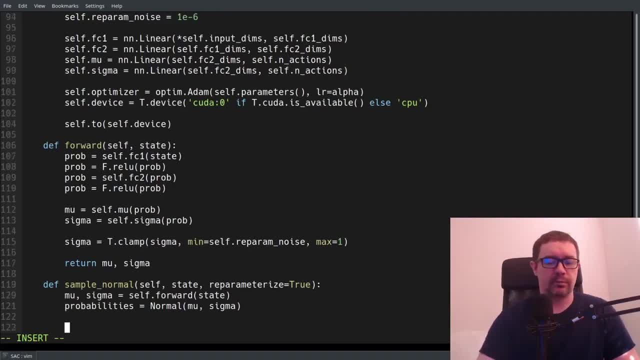 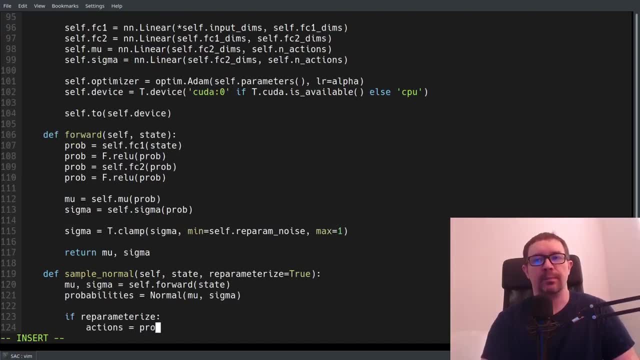 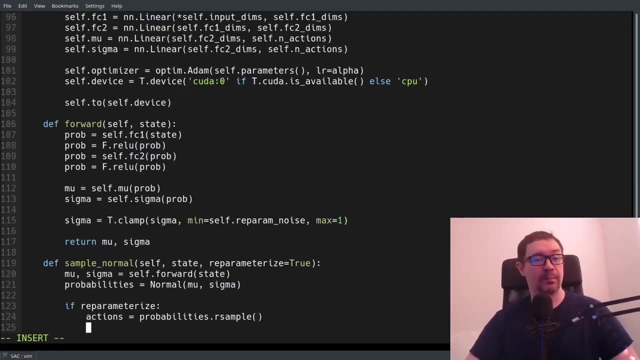 mu and Sigma. normal distribution defined in terms of mu and Sigma. if we're going to re-parameterize, then our actions are going to be a sample- sorry, in our sample- and what this does is there are two sample functions for the normal distribution. one gives you just a normal sample. the other one gives you a sample. 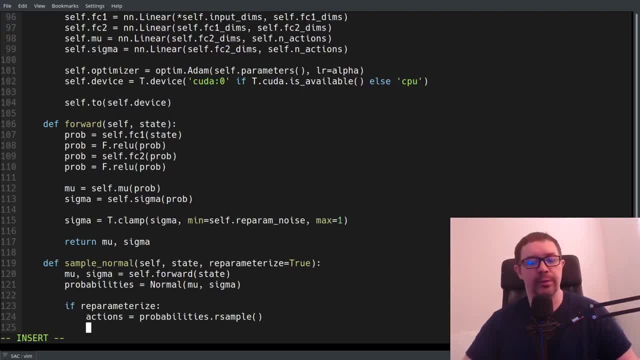 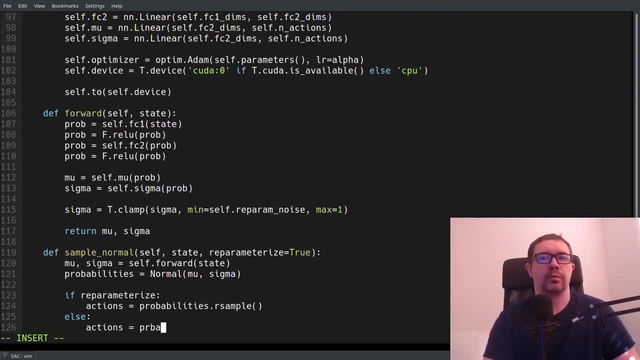 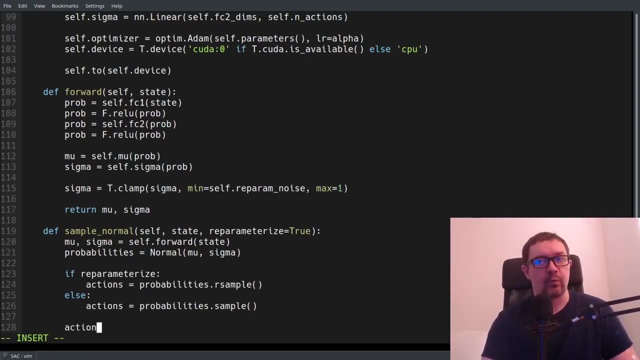 plus some noise. so we're adding some noise, some additional exploration factor to the actions. if we're not re-parameterizing, we just want to sample the distribution. next we want to get our action for our agent and that is a tan hyperbolic activation multiplied by the max action, because, remember the 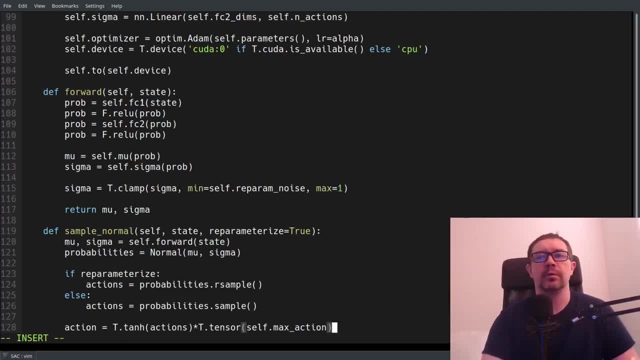 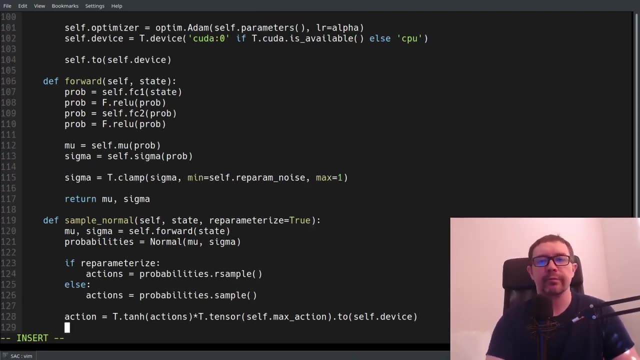 environment could very well have a maximum action beyond plus or minus one. and to make pytorch happy, we have to send that max action tensor to our device, because we have to have the same data types for everything in the entire graph and we're dealing with CUDA tensors elsewhere, so this has to be a 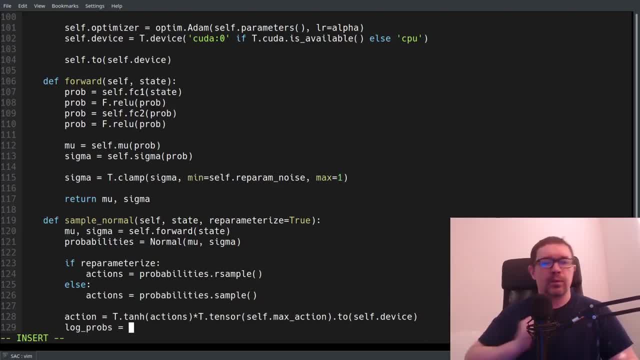 CUDA tensor as well. next, we want the log of the probability and this is for our, the calculation over loss function. it doesn't go into the calculation of what actually to take, but rather the loss function for updating the weights of our deep neural network. bill tease dot log prob. that's just a built-in function and we want to take it. 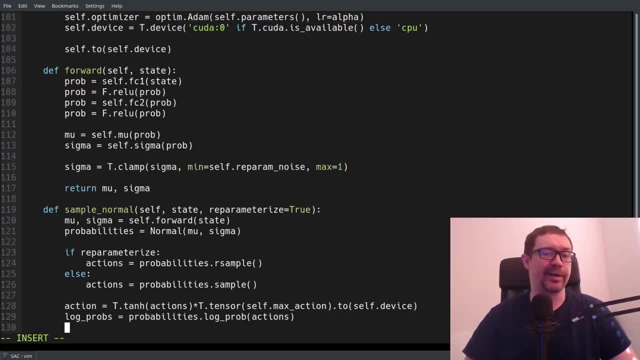 on the actions, not the action, so plural, not singular. the reason is that the you case here is proportional to the tan hyperbolic and the max action of our environment, whereas the actions are what we actually sampled from the probability distribution. so when we come here we're changing that. so we're not. we didn't actually draw the tan hyperbolic from the 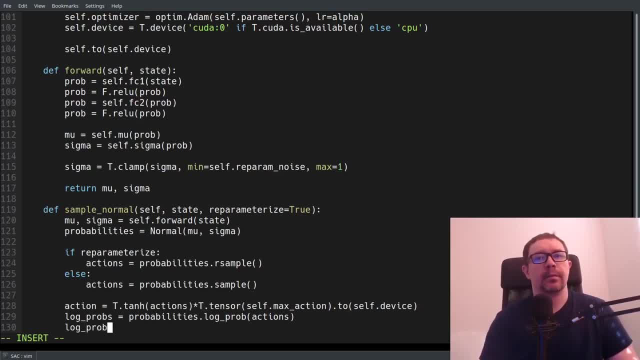 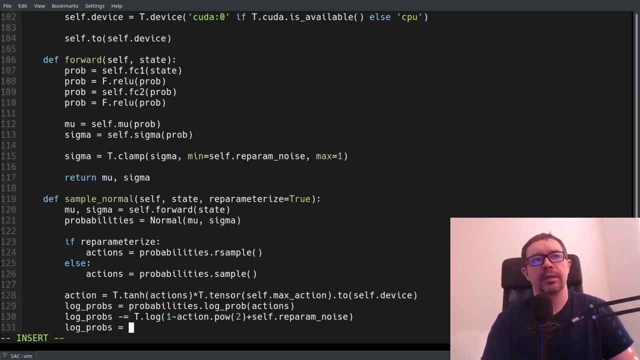 distribution very important. then you want to subtract off the log of one minus the square of the action, plus some reparam noise, because this could very well be one minus one, which would be zero. log of zero is undefined. and then we want to take the sum. the reason we want to take the sum: 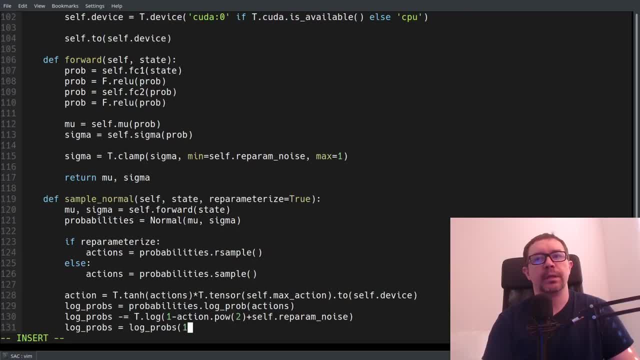 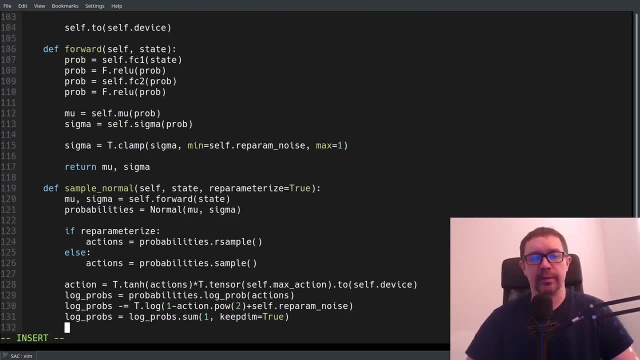 is because we need a scalar quantity here and the calculation of our loss and this log props will have uh number of components equal to number of actions, and this line here comes from the appendix of the paper. it's just how they handle the scaling of the action, you know. 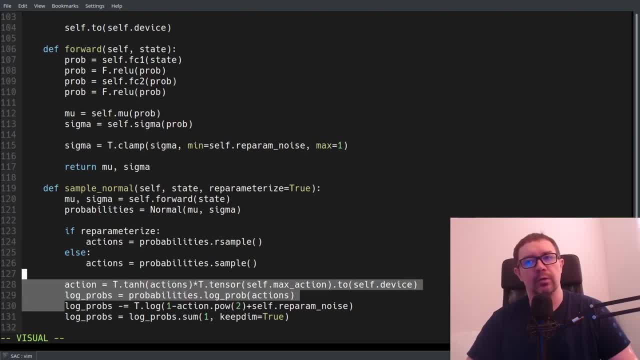 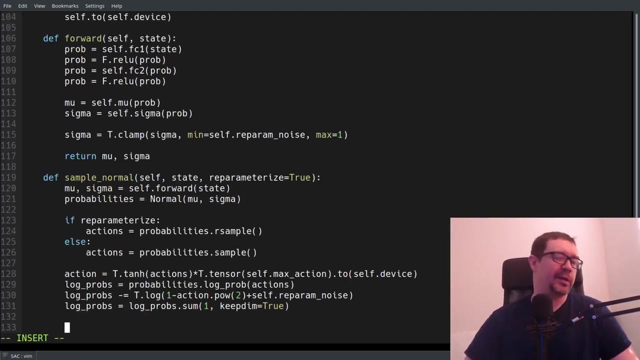 they do this. hyperbolic tan, hyperbolic activation- take the log problem and subtract off this term here and then. we have to do this because the pytorch framework outputs something that has dimensionality corresponding to the number of components of your action, and you need a scalar quantity for your loss. okay, so now that is clear as mud. again, i go into more. 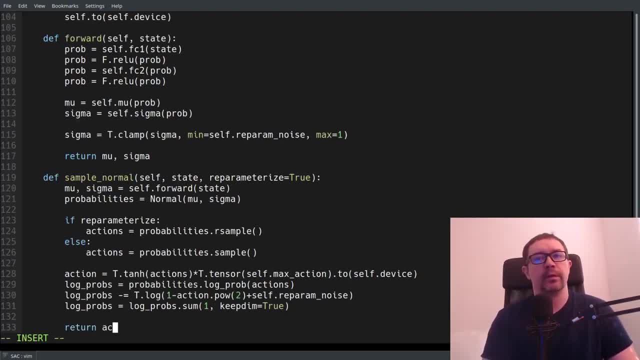 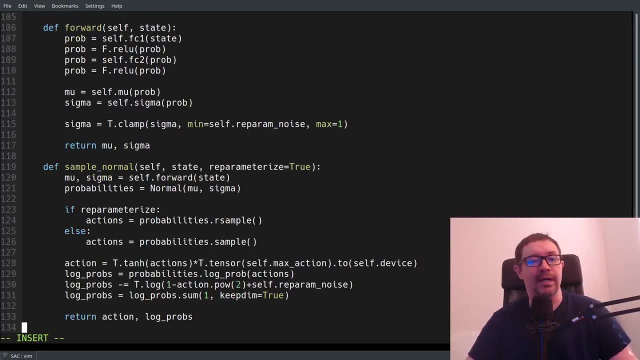 detail in the course. it's a little bit slower pace and it makes more sense when you see it in the context of the analysis of the paper. but we have limited time here so you just get the quick and dirty version. if you want, you can read the paper. it's very easy to find it's on the archive. 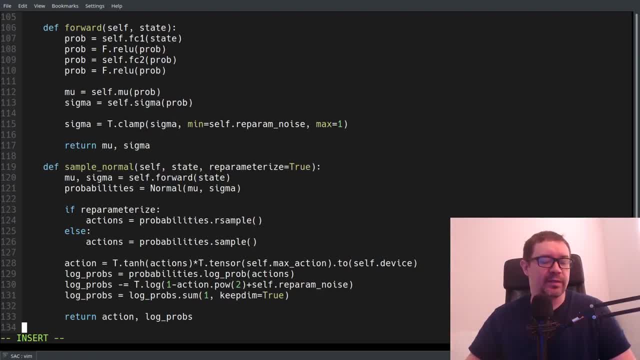 it's a very dense paper. that's where my course adds value is that i help break it down for you, but it's certainly readable by the you know advanced and dedicated student on their own. so you don't need me if you're you know, if you're really really good at this, but i do help. so 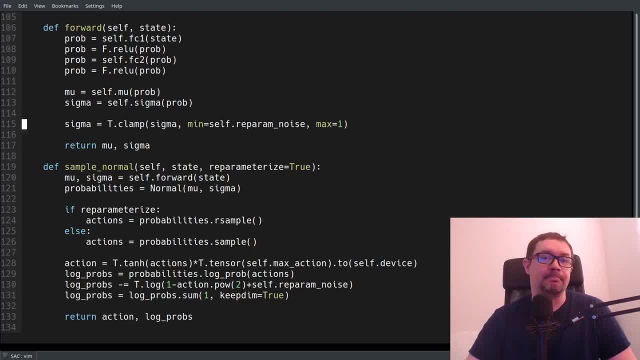 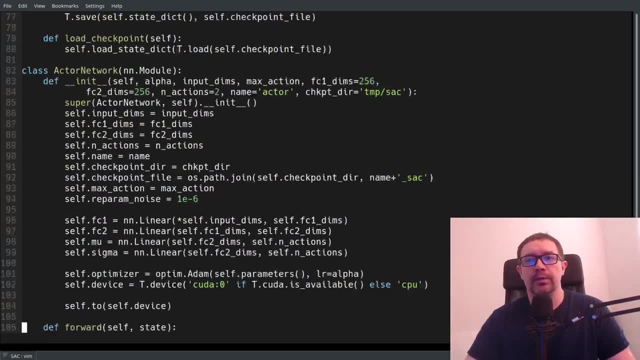 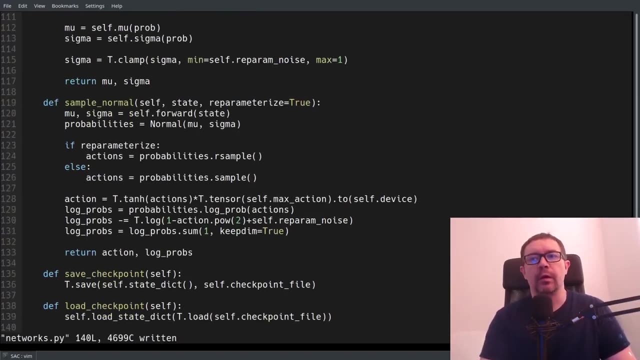 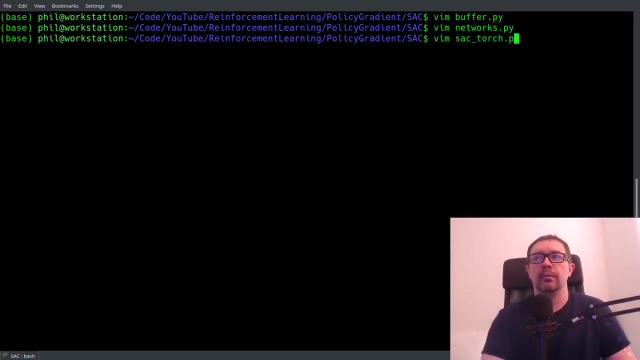 uh, that is it. uh, excuse me, we need our um functionality to save and load checkpoints. we'll just yank and paste those and now i believe we are done with our networks. okay, now we can handle the actual agent itself, so we'll begin with our imports. we will need os. 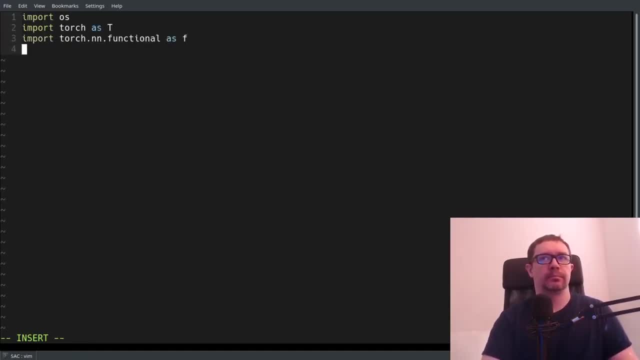 torch. we will also need numpy, we will need our uh replay buffer, we will need all of our networks and we're going to put all of our functionality in an agent class. we will need an alpha, a beta. you know what? um, let's do this alpha. i'm just going to use the defaults from the paper right away. 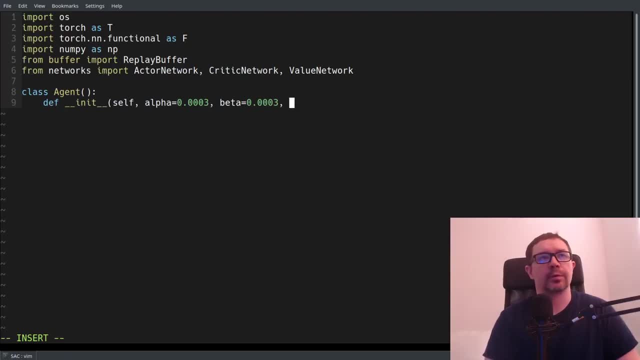 to use the default of 3 by 10 to the minus 4 for all of the networks. i'm just going to use something like 8 for the input dims, none for the environment and a gamma of 0.99. sorry, we also need a bunch of other stuff like and actions, uh. max size, that's uh 1 million. 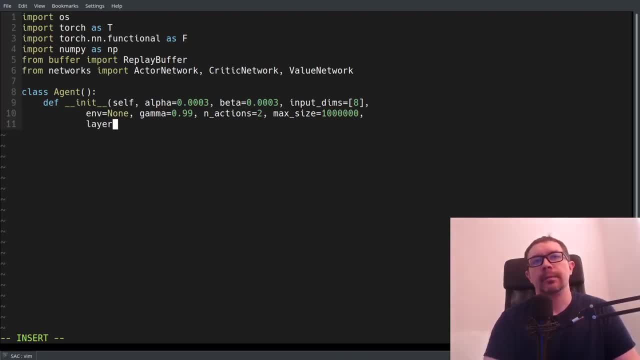 transitions for our memory um layer one size, a batch size, that is a default of 256 and a reward scale of two. so, uh, the reward scaling is how we're going to account for the entropy in the framework. basically, we're going to scale the rewards in the critic loss by some. 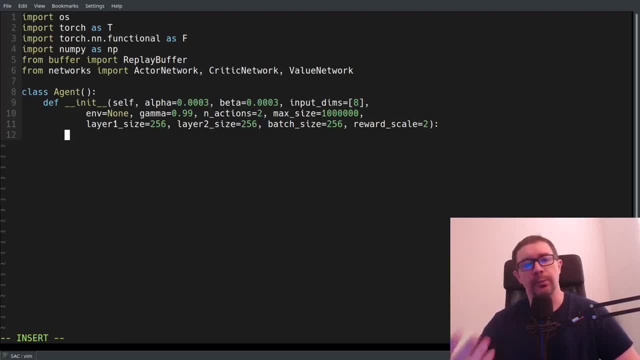 factor in this case. two because that works for our environment. we're going to be taking a look at the authors experiment with a wide variety of reward scaling factors and that is going to depend on the number of action dimensions for your environment. So we have a simple environment for this tutorial, so a reward scale of 2 is 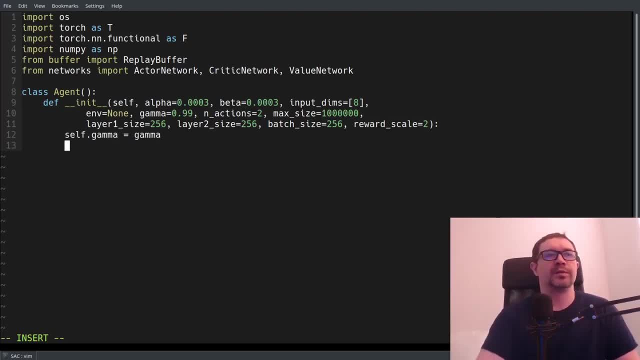 sufficient. So we're going to want to save the relevant parameters. and it looks like I forgot my tau. So the tau is the factor by which we're going to modulate the parameters of our target value network, So we're going to have a. 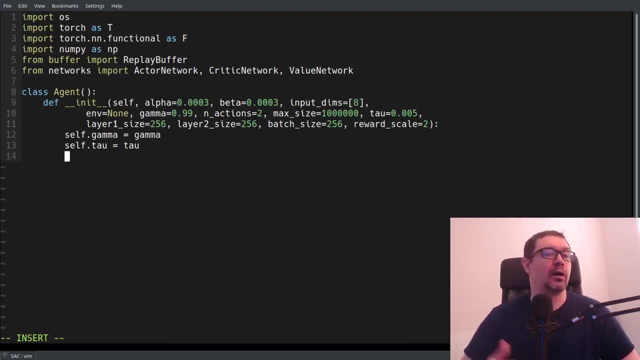 value network and a target value network and rather than do a hard copy of the value network, we're going to do a soft copy, meaning we're going to detune the parameters somewhat. This is reminiscent of DDPG in my code: td3, replay, buffer, max size actions. we also need our batch size. we need our n. 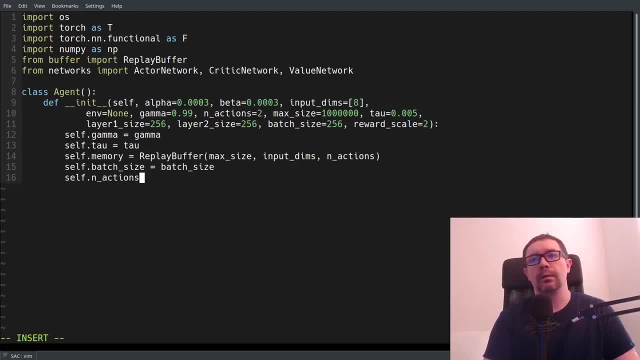 actions. and then we need our networks. so our actor, that's an actor network, and we need alpha and input dims. we already have strong defaults for our layer sizes, so we'll use n, actions, equals and actions. the name is going to be equal to actor and our max action. 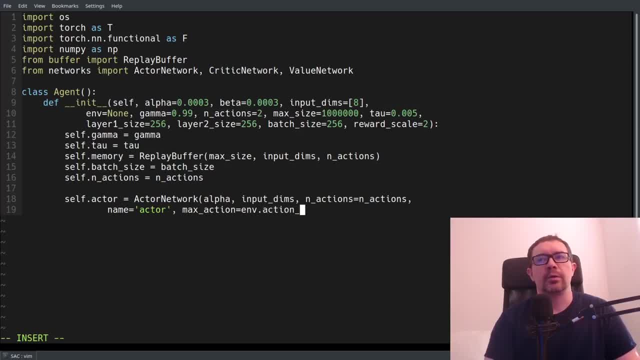 it's going to be equal to envaction space dot hi. and so I'm kind of wincing here, because I did some things differently in the course where I did a lot of experimentation with environments, and so I have some other parameters in here for my agent that. 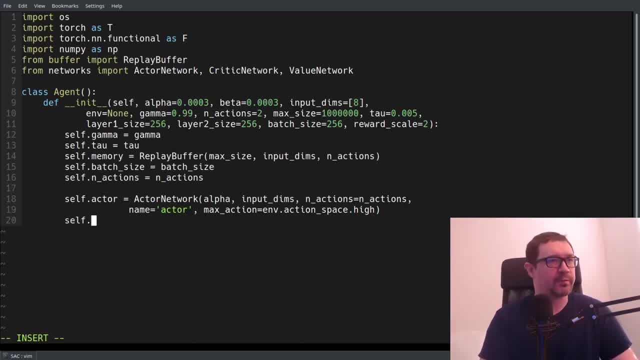 wouldn't really make sense for this tutorial, so I'm doing some changes on the fly. next, we're going to use two critics. so I said there's a critic network but in reality there are two and we're going to take the minimum of the evaluation of the state for those two networks in the calculation of our loss function for 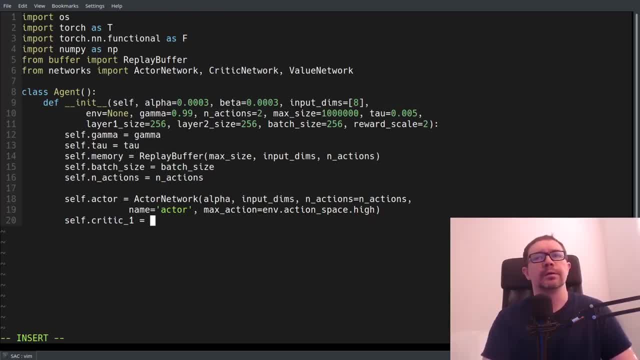 the value and actor networks, I believe. so we have critic one, that is a critic network, takes beta input, dims and actions equals and actions name equals critic one and that doesn't need a max action. similarly, for critic two, good grief, all right. and then we need a value network. 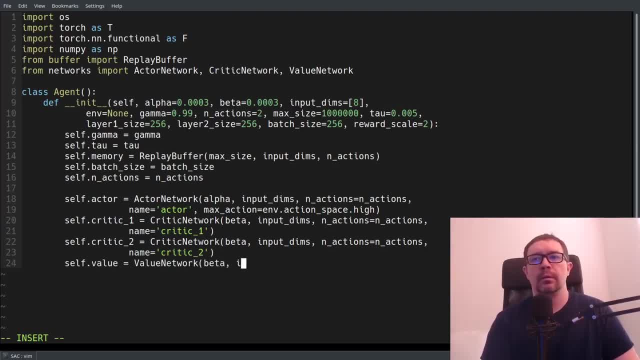 and a name of value. I think that's all the parameters we need to be able to use for this, for the value network, because we don't have number of actions. we already have strong defaults for the layer sizes. then we need our target value network and the 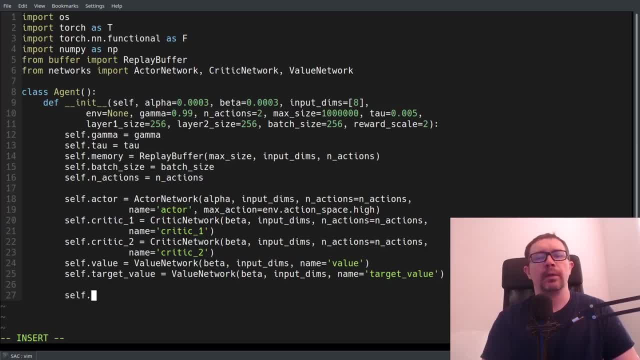 only real difference. there is the name, and then we need our reef word scaling factor and to call function called update network parameters. what this will do is it will set the parameters of our value network, our target value network, exactly equal to the values of the target network to. 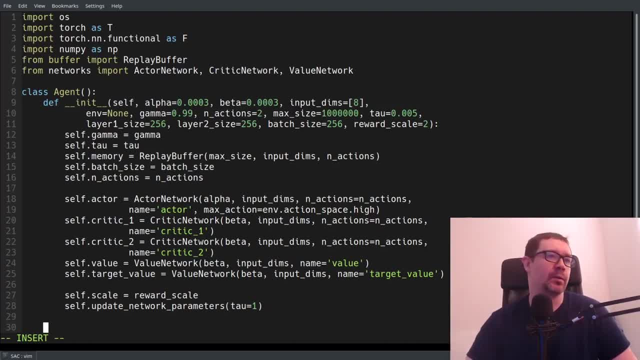 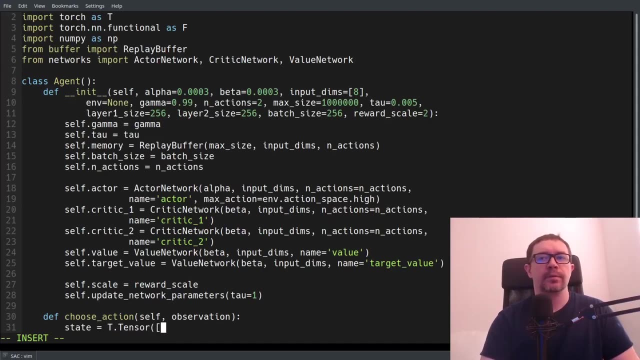 start and and on every other update, we're going to slightly detune them. we're going to update them with a slightly detuned version. so now we need to function, to choose our action. that takes an observation of the current state of our environment as input, so let's go ahead and turn our observation. 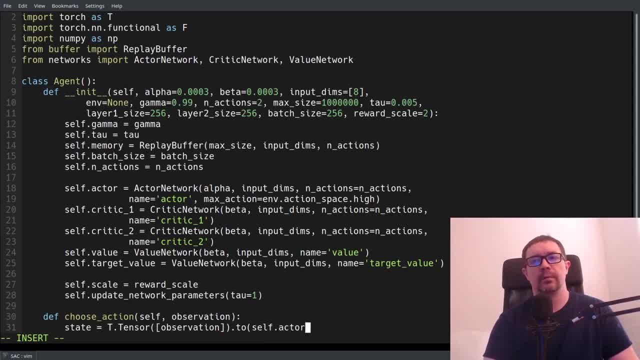 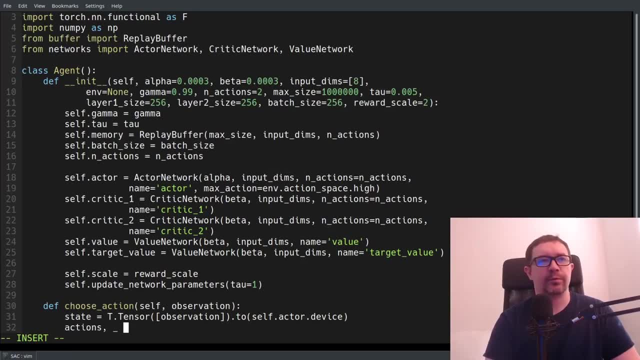 into a pie torch tensor and send it to our device, so it is a CUDA tensor, and then we're going to feed that state forward through the sampling function for our actor to get the actions and ostensibly or nominally the log probes back. but we don't care about the log probes, so we just use a blank state and 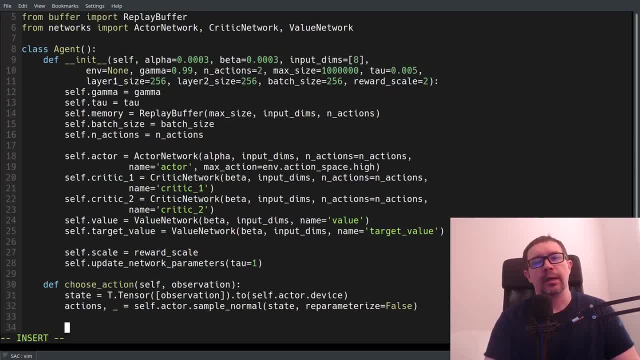 we're not going to re-parameterize for our action selection now, then we're going to return it. it is a CUDA tensor, so we have to send it to the CPU, we have to detach it from the graph and we have to turn it to into a numpy array and take the zeroth element. that's one of the 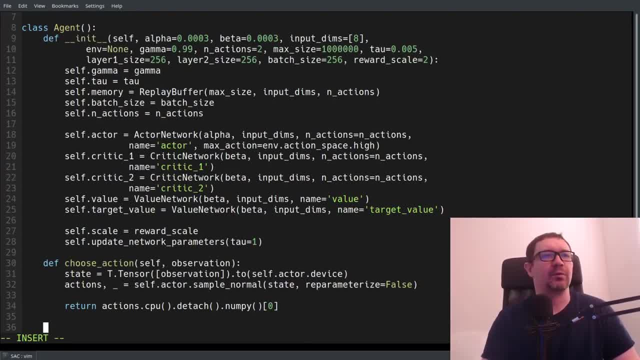 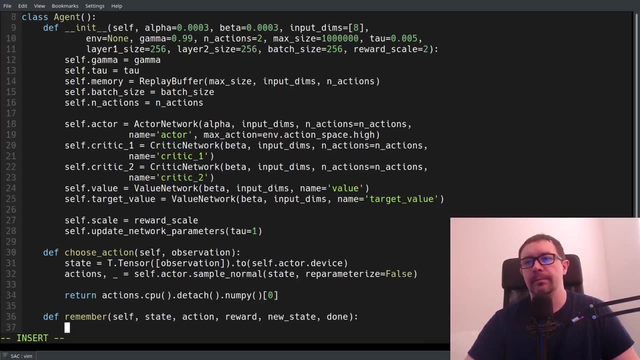 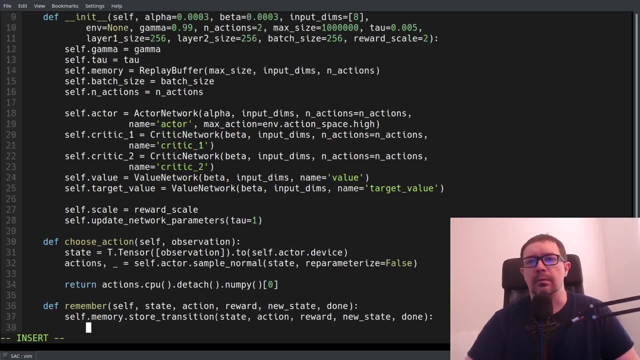 quirks of the pie torch framework. it's something we can live with, though then we need an interface function between the agent and its memory. so we'll take a new state action, reward new state and done flat as input, and then we're going to store that transition. all right, oh, I don't. 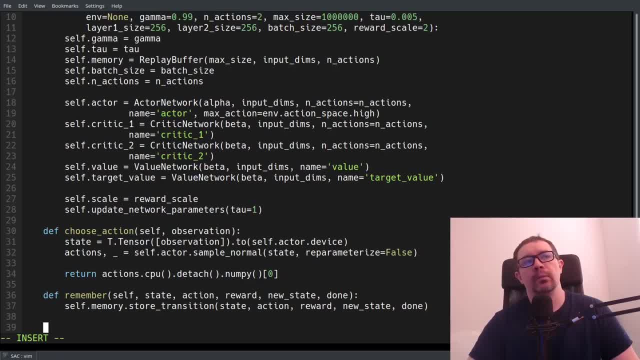 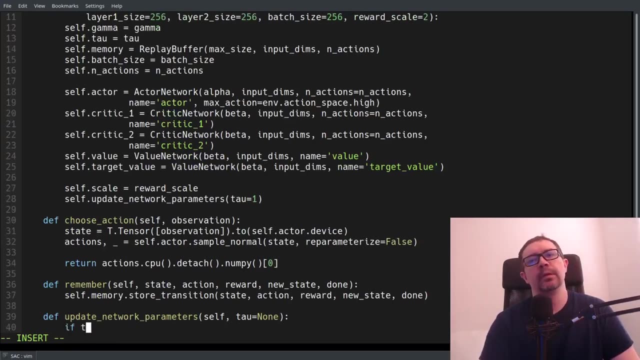 need a colon there. don't know what I was thinking, and then I'm going to write the let's get the two bookkeeping functions out of the way list to update network parameters. now, this is kind of a clunky function, so if tau is none, then we're going to set. 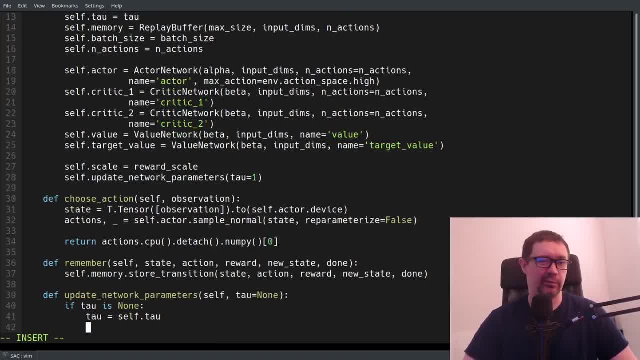 tau to the stored value for agent. and the reason we have to do this is because at the beginning of the simulation we want to set the values for the target network to an exact copy of the value network. so the target value network should be an exact copy of the value network. but on every other step we will. 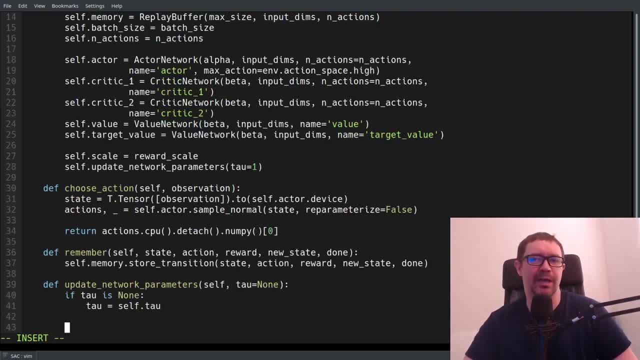 put as a 클�ew theですね. ok, here we have the target value of the session and then say target Silva and if we do that it should take in the first case a Stan. that is in the solution which that maybe is stuck into un spoilers, because I want it to be a. 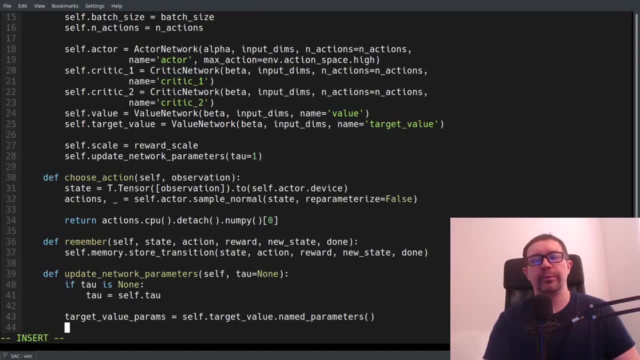 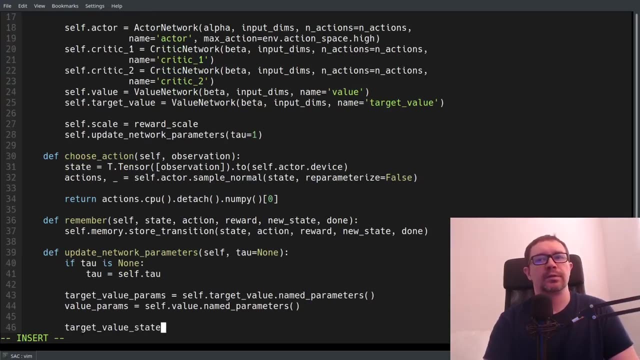 soft copy, so I use this mechanism with tau equals none to facilitate that, and then my solution here is kind of ugly as well, so we'll say target value params. basically, what I'm gonna do is create a copy of the parameters and modify them. ValueNamed parameters. valueStateDictionary equals Dictionary. 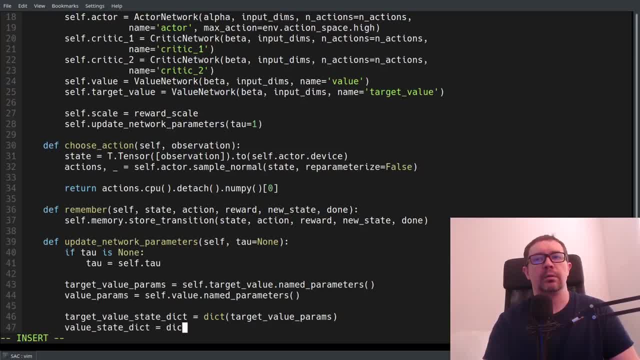 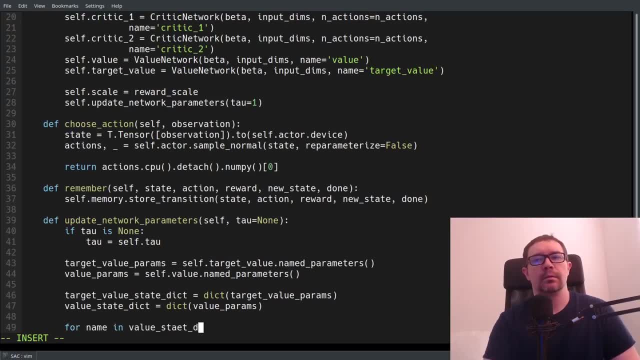 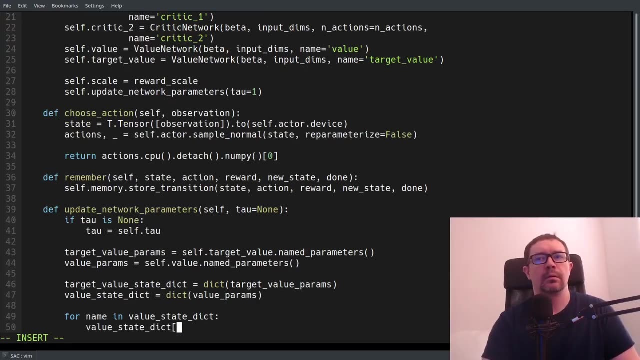 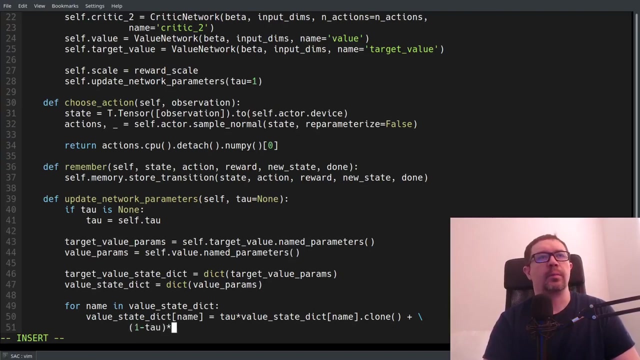 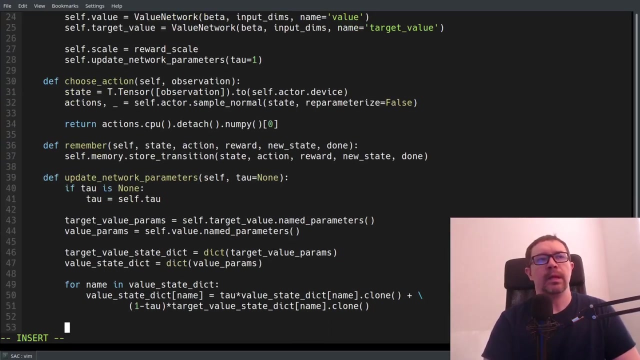 And then valueStateDictionary dictionary of value params for name. in stateDictionary We're going to set the parameter to tau multiplied by the stateDictionary and 1, 1 minus tau multiplied by target valueStateDictionary clone. And then we're going to load that dictionary selftarget. 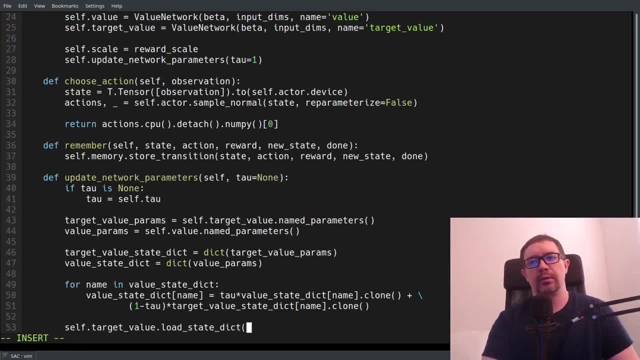 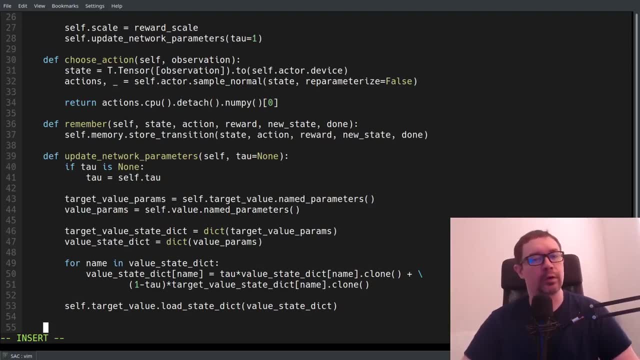 Value: loadStateDictionary- valueStateDictionary. Okay, so that is the function to update. to perform a soft or hard update for the value network parameters, Then we need two functions to handle the interface with the agent's network: save model checkpointing functions. 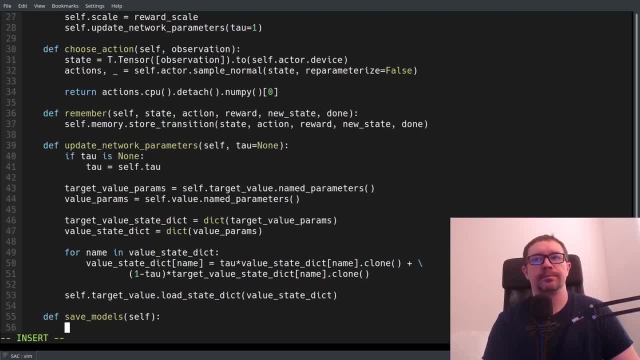 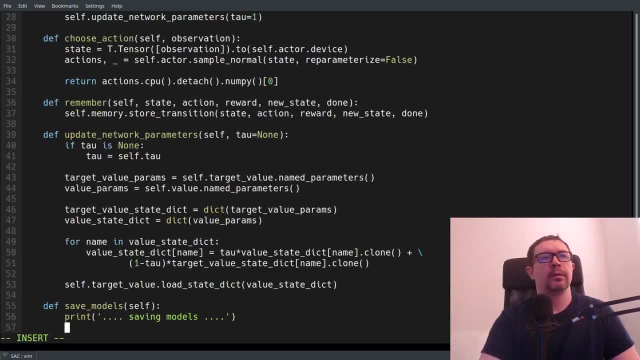 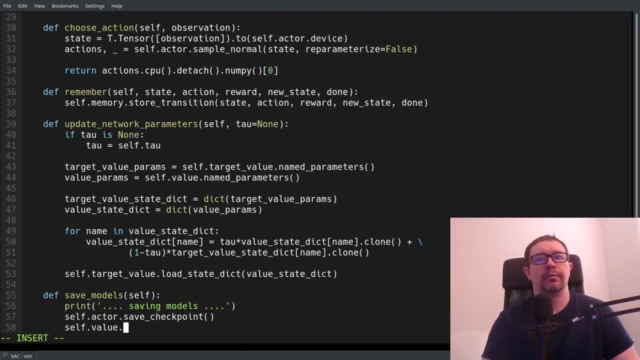 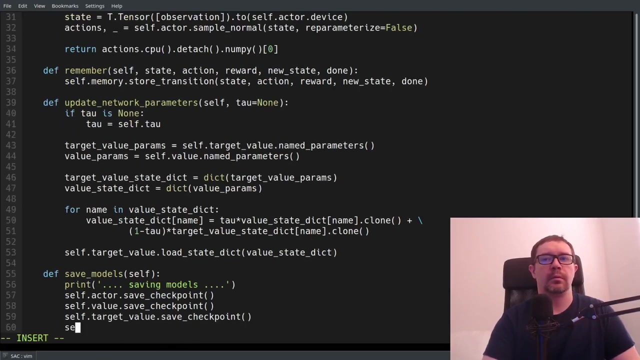 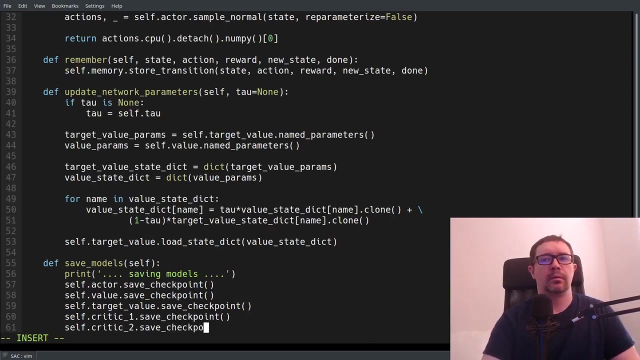 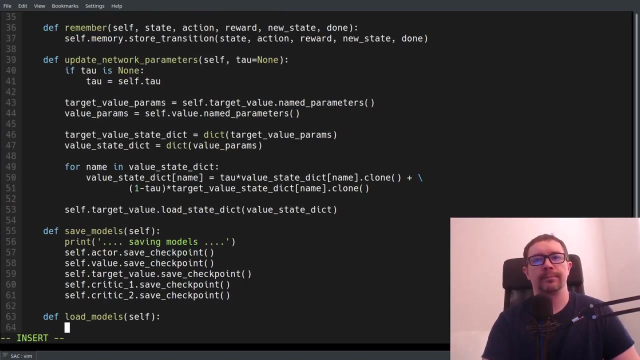 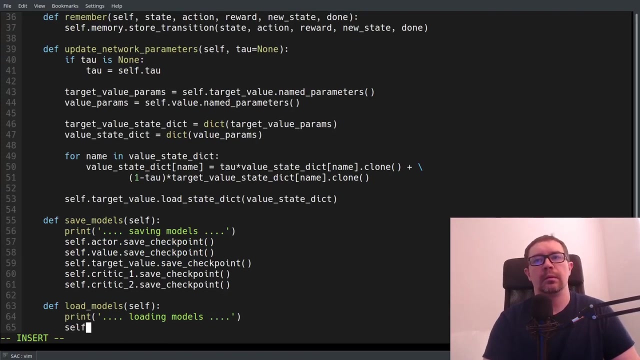 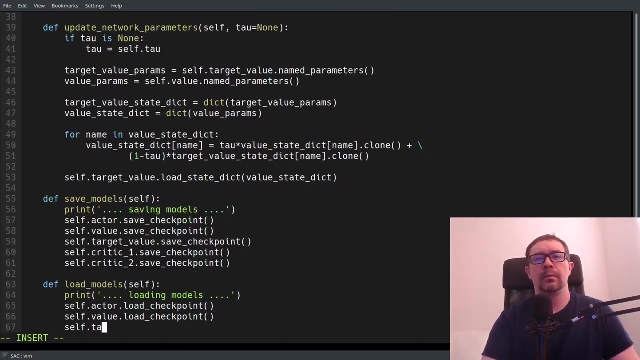 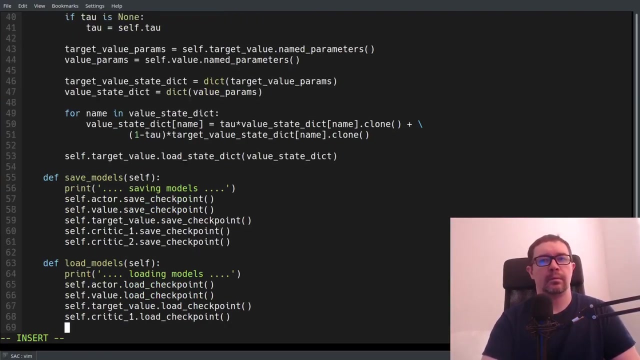 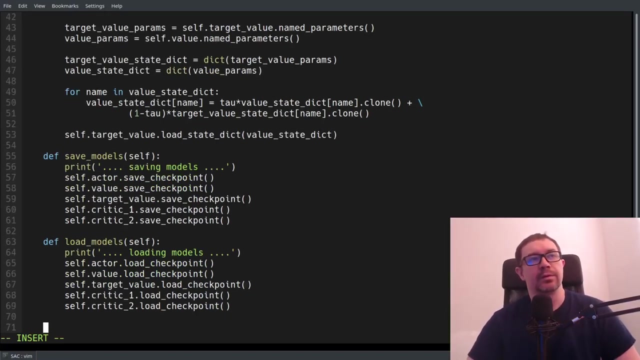 So we'll say def- save models, And then, similarly, we need a function to load our models, And then we need a function to load our models, And then we need a function to load our models. So that stuff is over. And now we have to worry about the actual learning functionality of our agent. 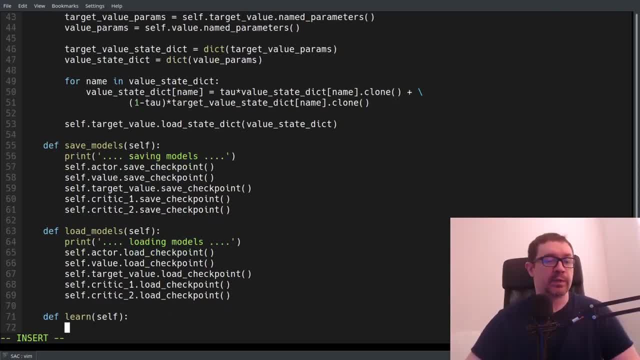 And that is the heart of the problem. So the first thing we want to do is see if we have filled up at least batch size of our memory, And if not, we're not going to bother learning, We're just going to go back to the main loop of the program. 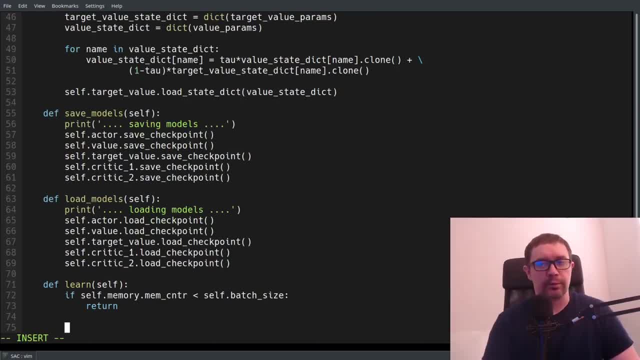 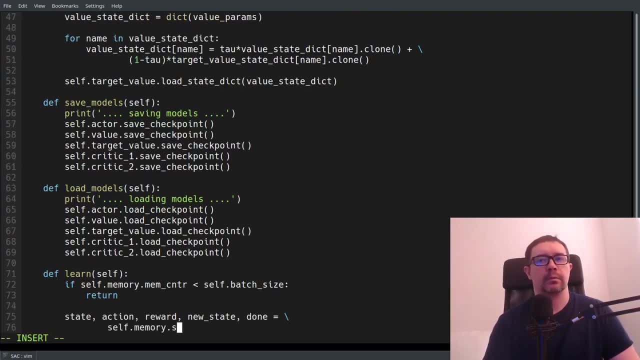 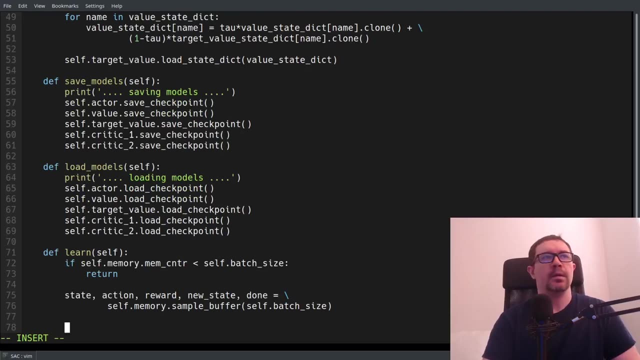 And if we have filled up our batch size, we're ready to go ahead and start learning. The first thing we want to do is sample our buffer And then transform those numpy arrays into PyTorch tensors. Now you may ask: why don't I just handle this in the replay buffer class? 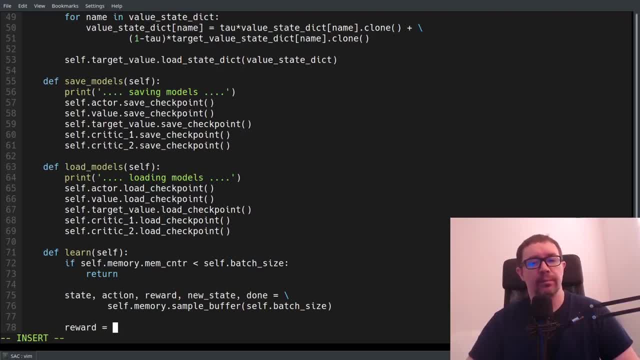 And that's because I want the replay buffer to be framework agnostic. I want it to work with Keras, TensorFlow and PyTorch, So it just It just should be stored or written in terms of numpy arrays or some other structure that is, you know. 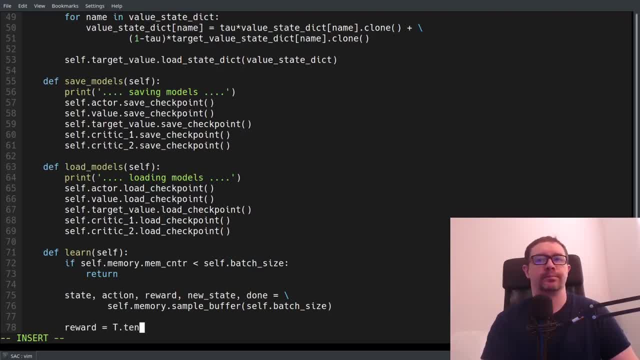 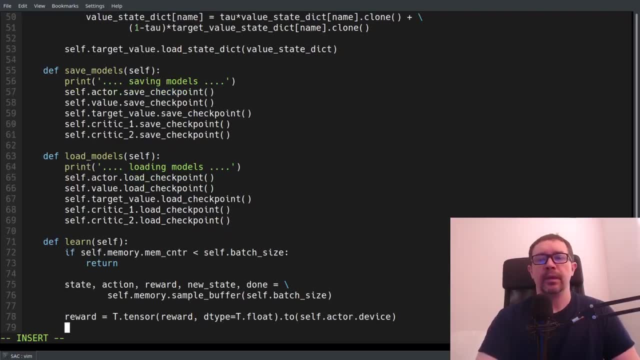 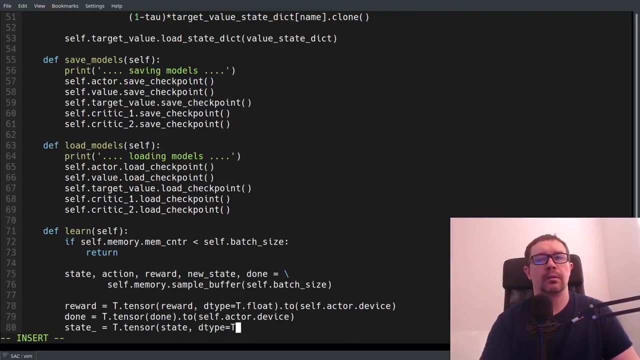 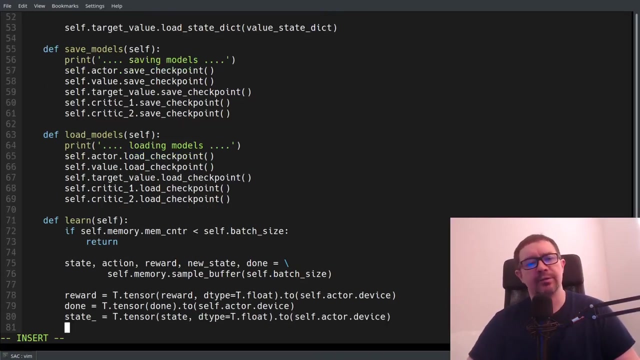 ambivalent about whatever type of tensor we choose to use later, And so I'm going to turn them into CUDA tensors. We will need our state. I'm setting all of these to the actor device. It doesn't really matter, because all the devices for the networks are the same. 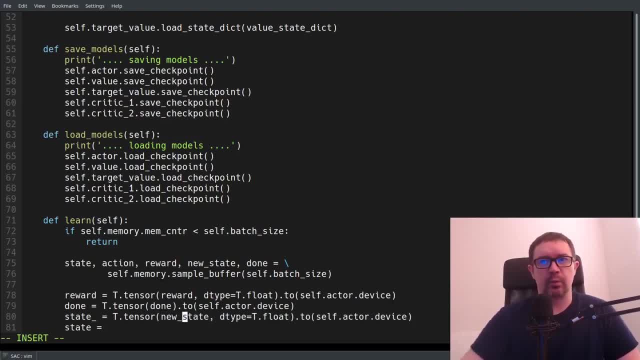 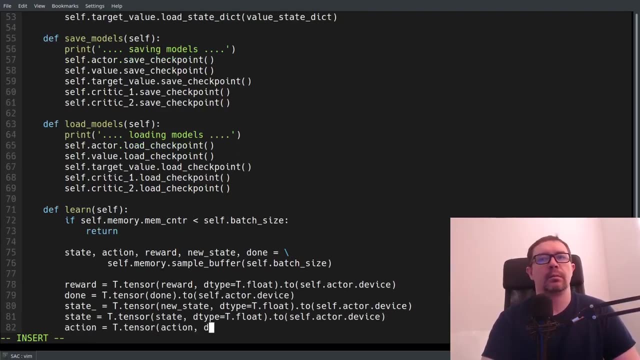 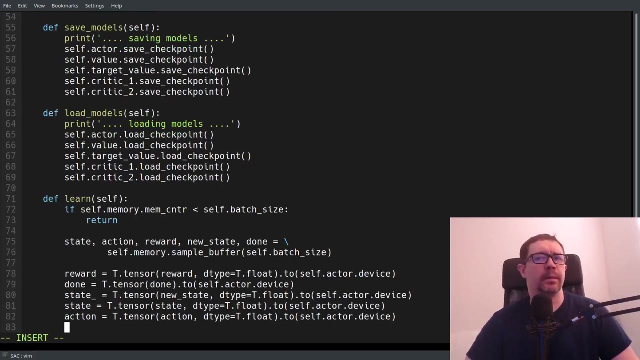 It should be new state, Otherwise this will not work. That will be horribly broken. That would be a tough bug to hunt down Because it's not something I would think to check, And I'm being very pedantic about the data types here because PyTorch is quite particular. 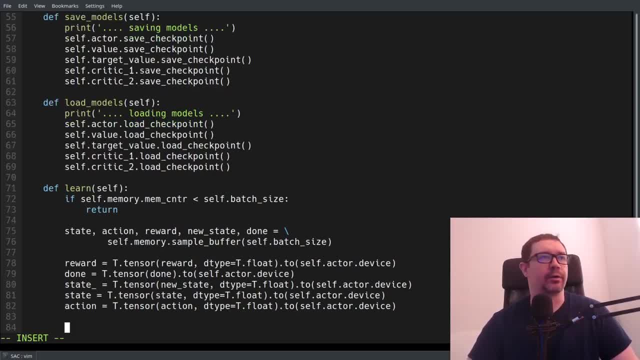 And so I want to be sure that I don't, you know, flag an error when the software is running later. So next we have to calculate the values of the states and new states according to the value and target value networks respectively. 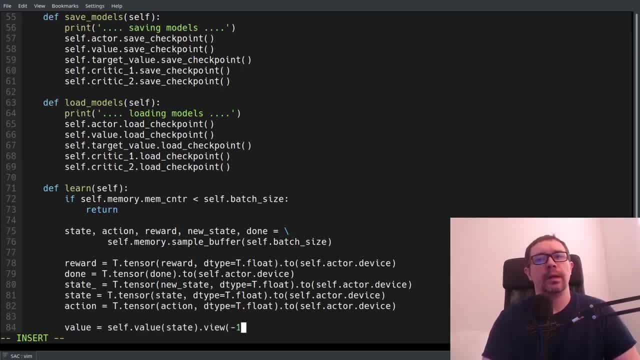 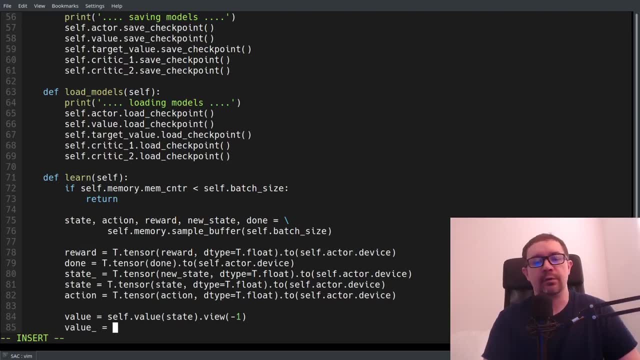 So value state and I have to collapse along the batch dimension due to the way the loss is calculated. So you'll see a dot view minus one. That just means it returns a view of the tensor with one less dimension And it collapses it, in this case, along the batch dimension because this will return a tensor of tensors, which doesn't make sense for a tensor of scalars. 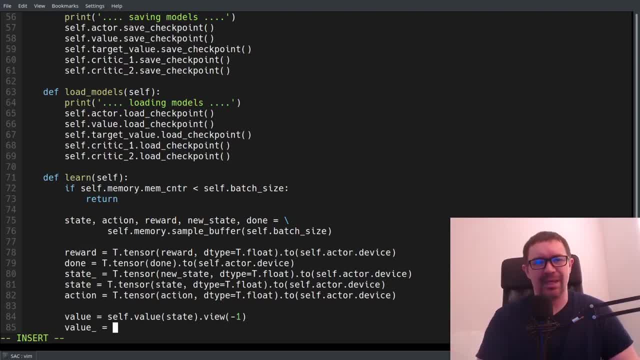 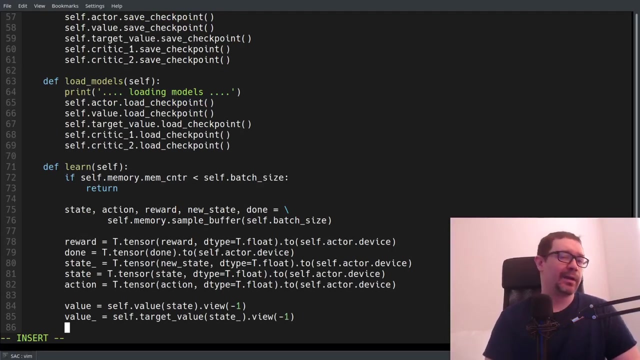 You know you don't want each of those inner scalars to be wrapped in brackets. It doesn't make any sense. So you just return a view Along the minus one direction, Target value Along the minus one direction And if that is mysterious to you, get rid of it and print out the shapes of stuff to the terminal. 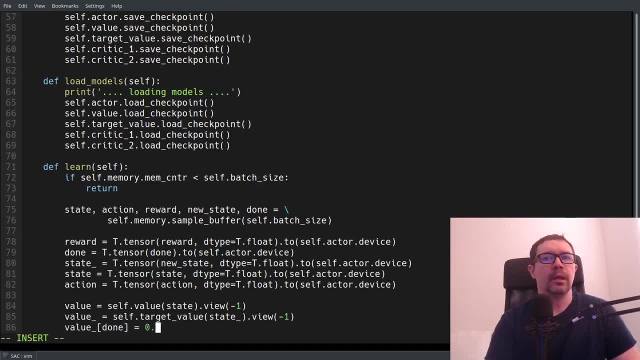 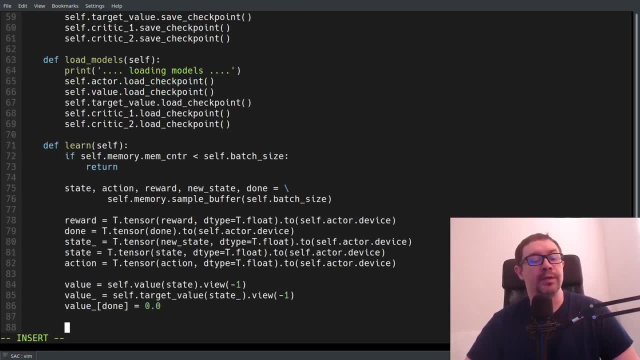 And that'll make it a little bit more clear. And then everywhere that the New states are terminal, we want to set the value to zero, because that is just the definition of the value function. And I'm kind of looking at this funny because I noticed that here I use the, basically the call method. 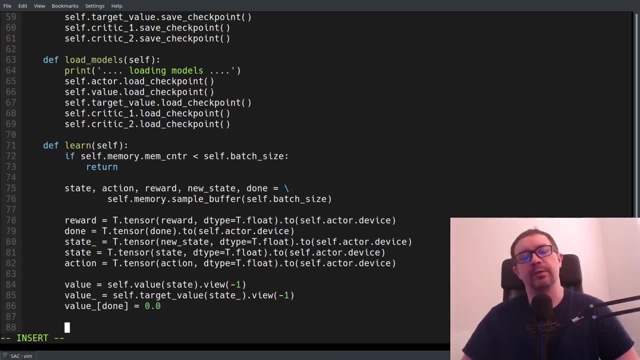 And then down there I do the dot forward, which is pretty funny. So I kind of switched up my nomenclature halfway through the learning function And I didn't realize it when I was doing the video for the course. It's a little bit funny. 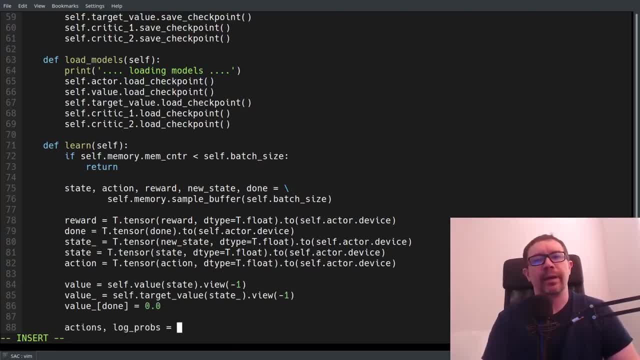 It doesn't affect the execution of the program. It doesn't really matter, It just affects the execution of the program. It doesn't really matter, just looks weird. so the next thing we have to do is we have to get the values, we have to get the. 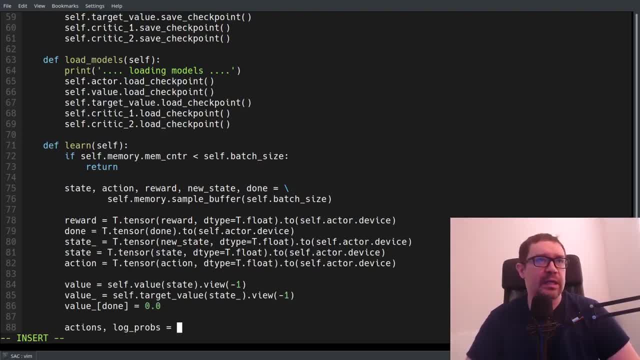 the actions and log probabilities for the states- uh, according to the new policy- and not for the actions that were actually sampled from our buffer. we'll use those later, but in the calculation of the loss for our value network, we, as well as the critic network, we want- sorry, the value network. 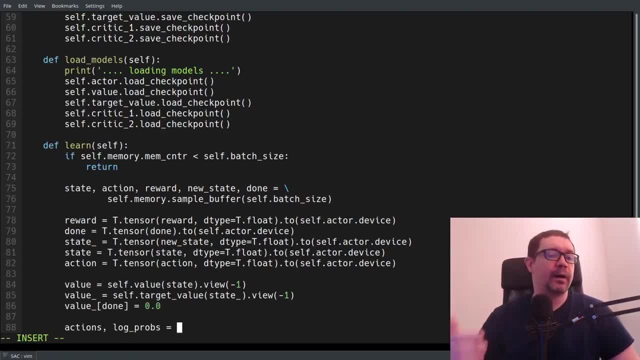 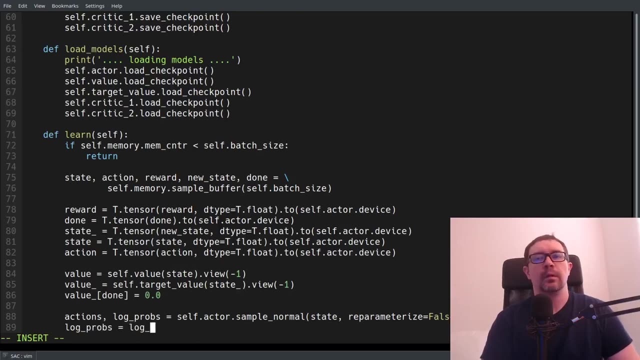 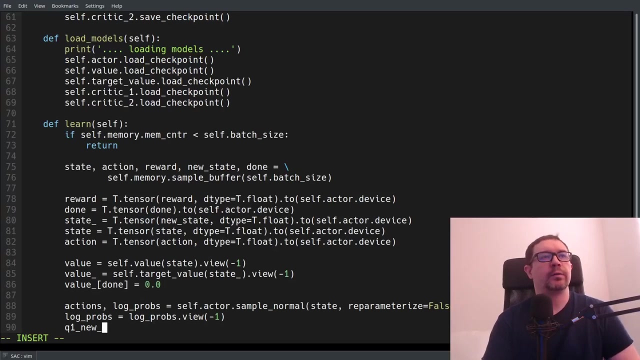 and the actor network. we want the values of the actions according to the new policy and we don't want to use the reparameterization trick here, but we do want to use the view. and then we're going to need the q values, the critic values under the new policy. 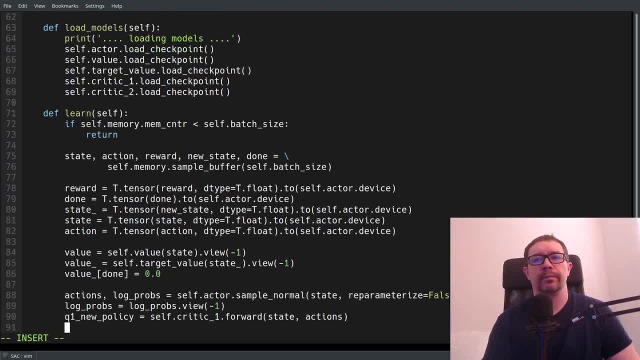 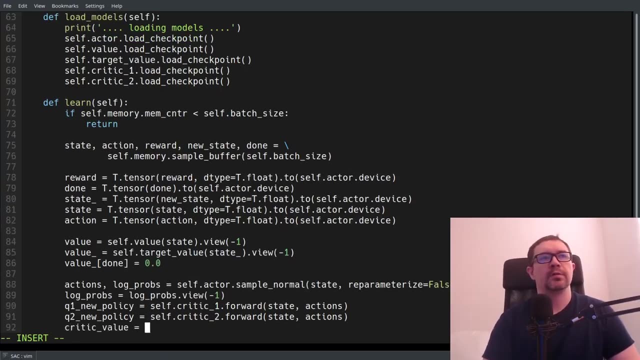 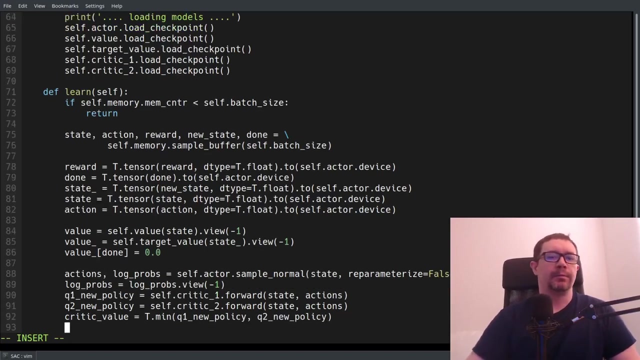 state actions- notice I'm using actions and not action. then we have Q2: new policy, state and actions. our critic values and going to be is then going to be the minimum of those two. If this is mysterious, we do this because you actually improve the stability of learning. So 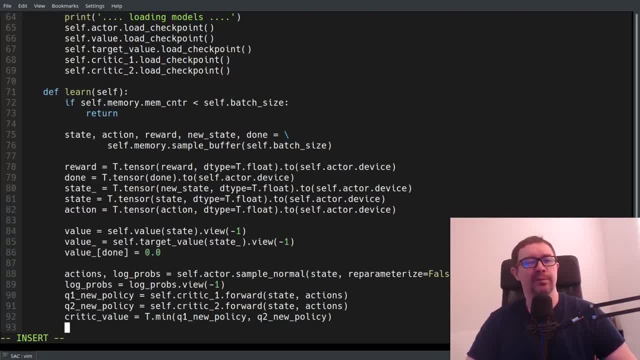 if you're familiar with Q learning, you know that there is a problem of the overestimation bias. So overestimation bias happens not just as a consequence of the fact that you're using a max over actions in the Q-learning update rule. It happens also as a consequence of using deep neural. 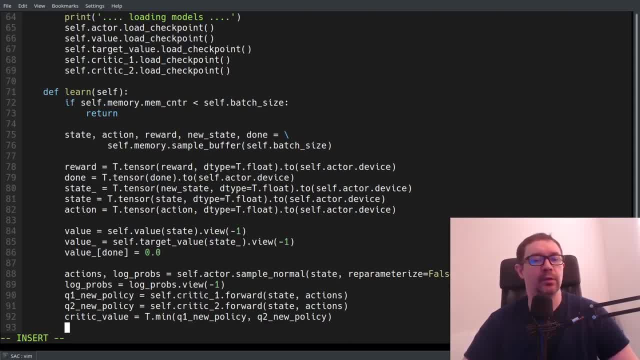 networks. So they kind of demonstrate this conclusively in the TD3 paper. And so one way around that is to make a direct analog of the double Q-learning update rule by taking the values of the states and actions with respect to two different q functions and then taking 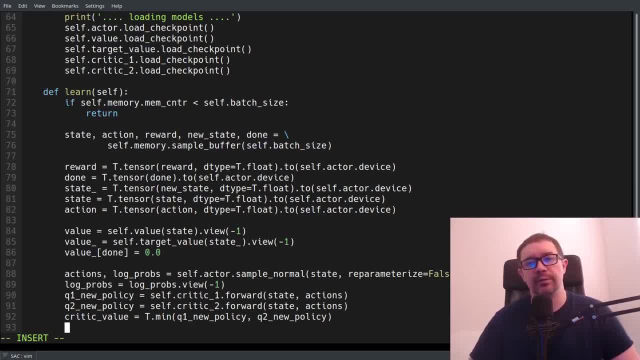 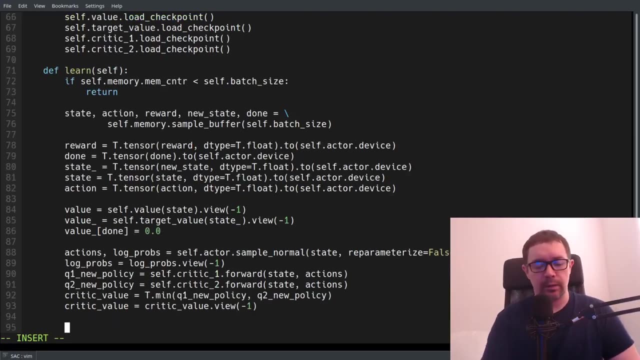 their minimum instead of a maximum, so it's a pretty clever solution. you can see more of that in the video on td3. but that is the basic idea, and of course we want to return a view and collapse along the bash dimension here, and then we can go ahead and calculate our loss and back propagate. 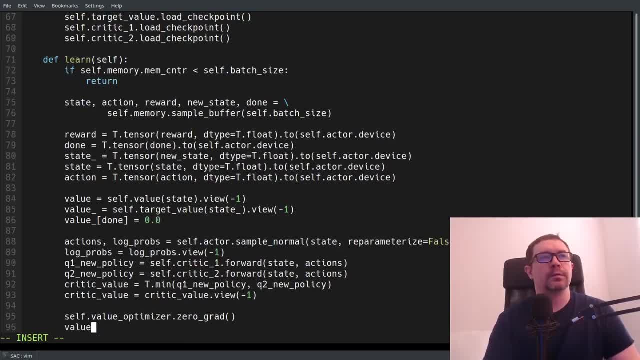 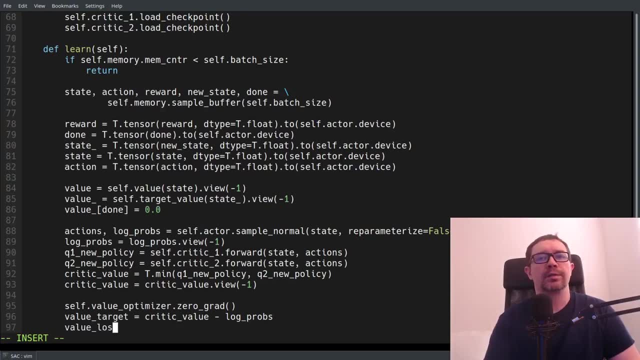 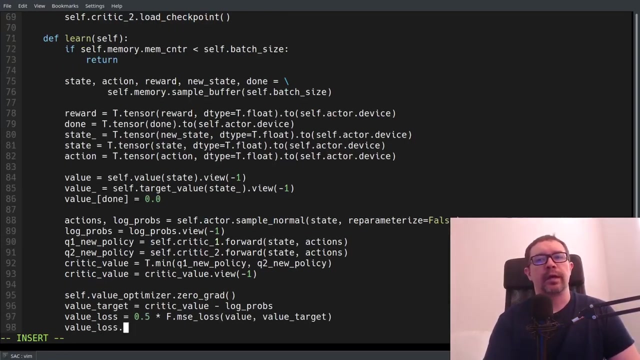 so our value target will be the critic value minus the log probs and then our loss will be 0.5 multiplied by f, dot, msc loss value and value target. then we want to back propagate, but i don't know if you're aware of this. 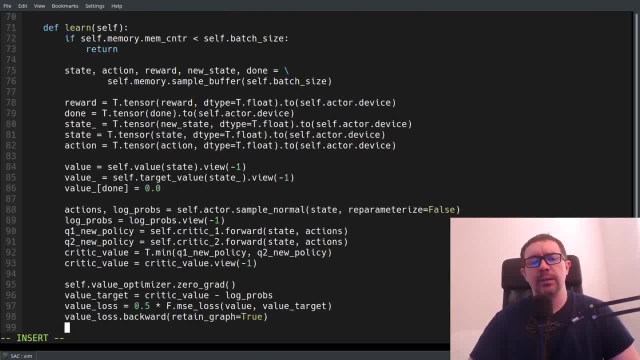 option for the back propagation function. but you can actually retain the graph between back propagations by default. pytorch will discard the graph calculations every time it back propagates and we don't want to do that because there's coupling between the losses for the various deep neural networks. so we want to keep track of that graph. 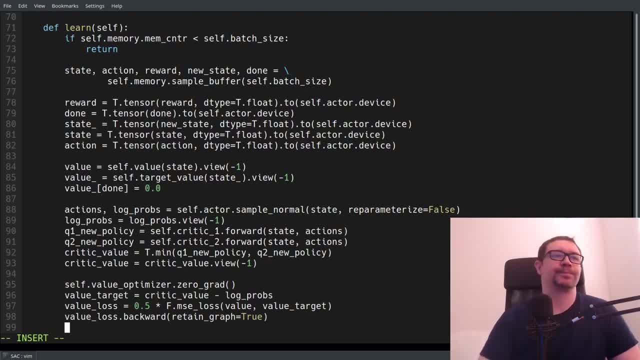 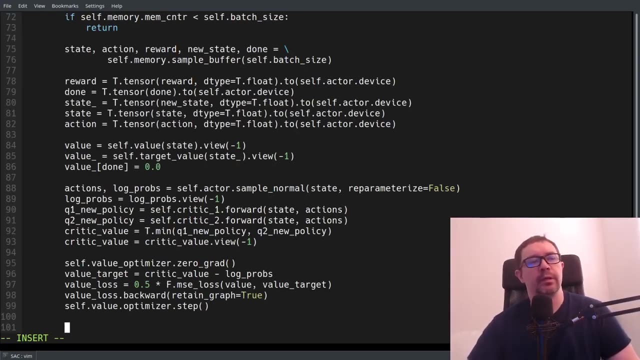 for the losses, for the value and actor networks, and then we say value maximizer step, so that handles the value network loss. now we're ready to deal with the actor network loss and so we start by doing another feed forward to get the actions and log probs. but in this case we do want to use the reparameterization trick. then we'll say log probs. 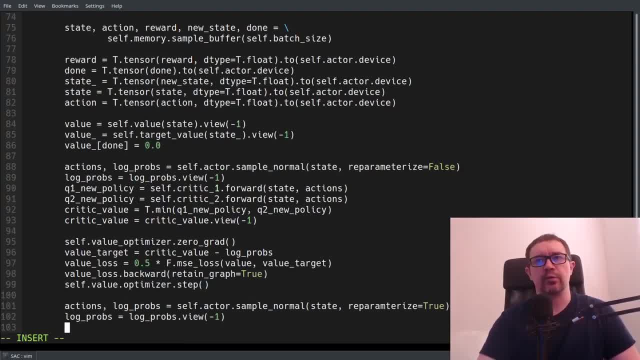 view minus one. it's otherwise identical to that other chunk of code up there. uh, it's just that we have to do the reparameterization trick here. so q1 new policy. in fact, i'm just going to copy this code now, if you wanted to be a good little data scientist. 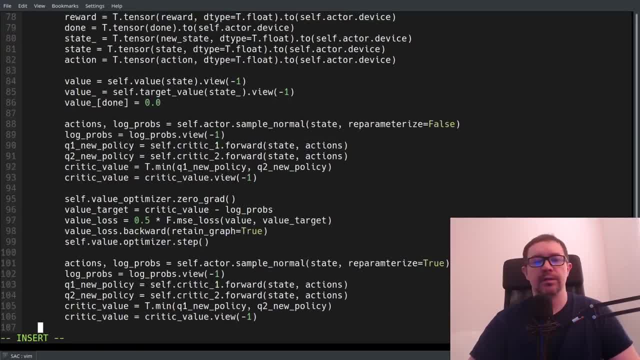 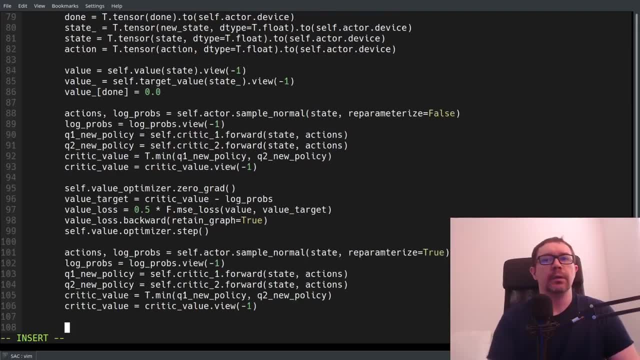 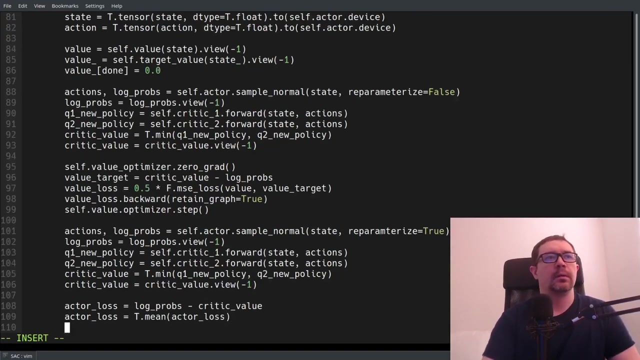 you? um would stick this in a separate inner function, but i included all of the code here twice just for clarity. so then we see actor loss log probs minus critic value, and then we say actor loss t dot mean. and then we want to zero out our optimizer. 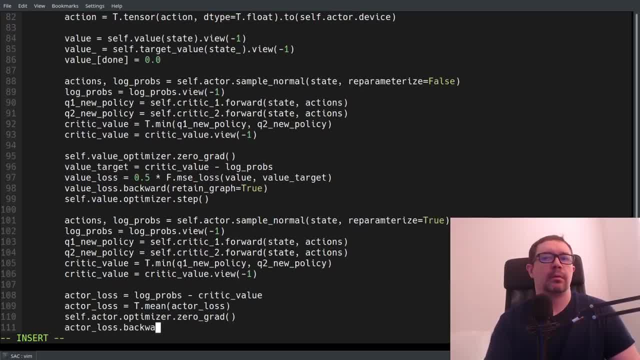 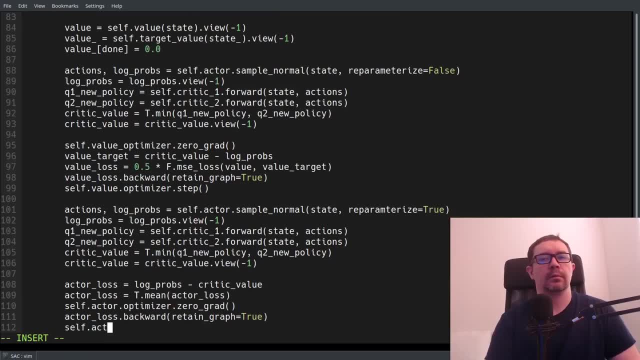 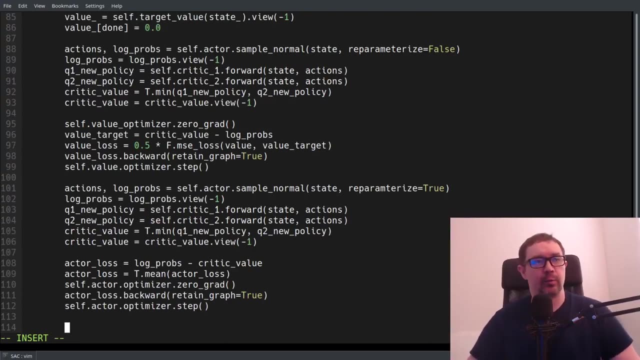 back, propagate again with retain graph equals true and step our optimizer okay. so now we only have one last thing to deal with for this particular function. we have to deal with the critic loss. so this one is a little bit more straightforward. it's more similar to what you would get with something like q learning, so we'll say let's go. 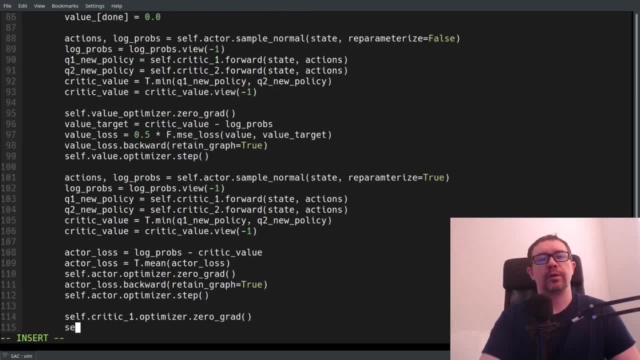 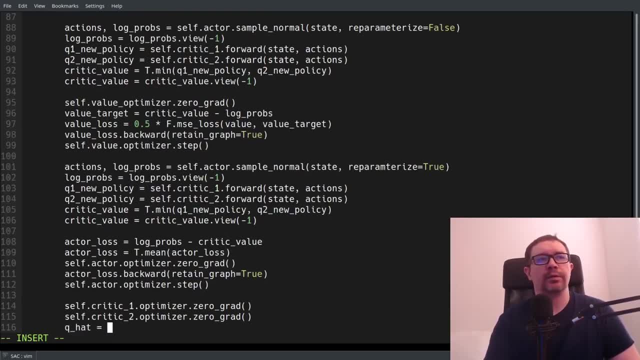 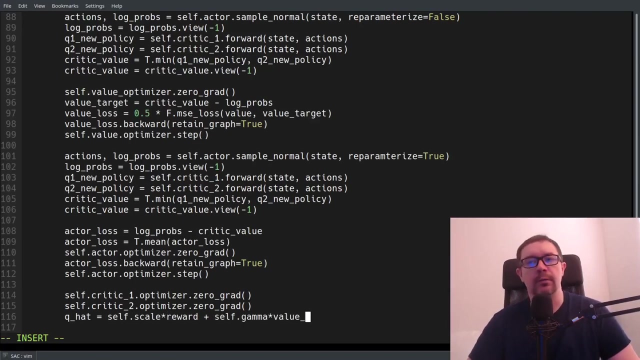 ahead and zero out our gradients for both critics and calculate this quantity called q hat. that's our scale factor multiplied by our reward plus gamma times value underscore, so that scaling factor handles the inclusion of the entropy in our loss function. so that's what helps to encourage exploration. uh, and we also, of course, need gamma. 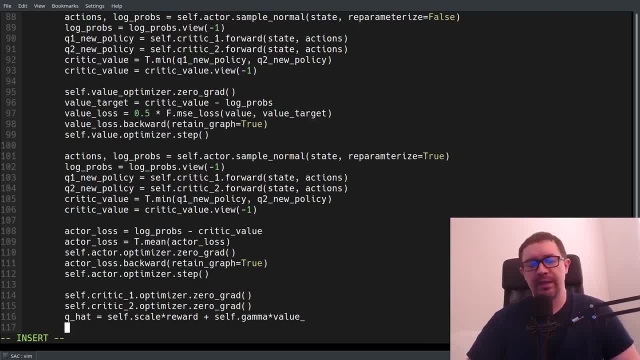 multiplied by the value of the uh loss function. so that's what helps to encourage exploration states resulting from the actions the agent took. so then we have q1 under the old policy. this is where the actions from a replay buffer come into play. critic one dot forward. 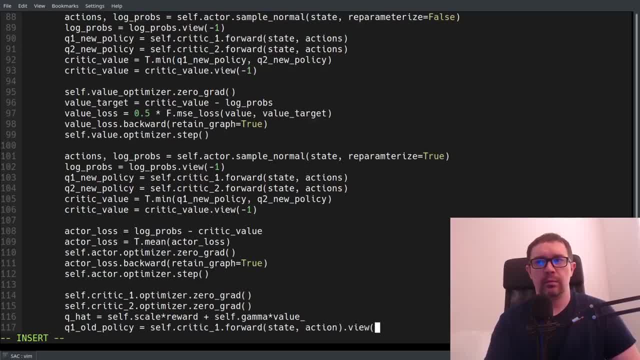 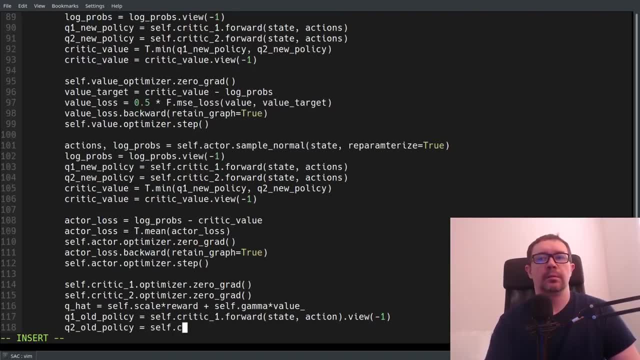 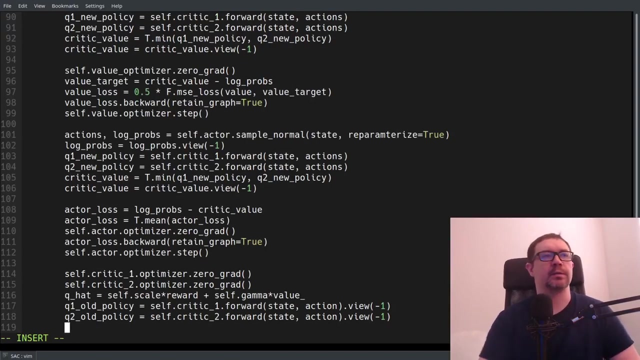 state action view minus one. it would help if i spelled action correctly. and note again, i am using the action from from the replay buffer here, hence it is under the old policy, not the policy as it is right now. one loss equals one half of the mean squared error loss. 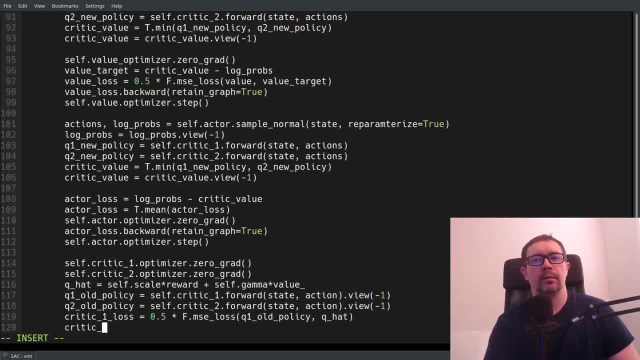 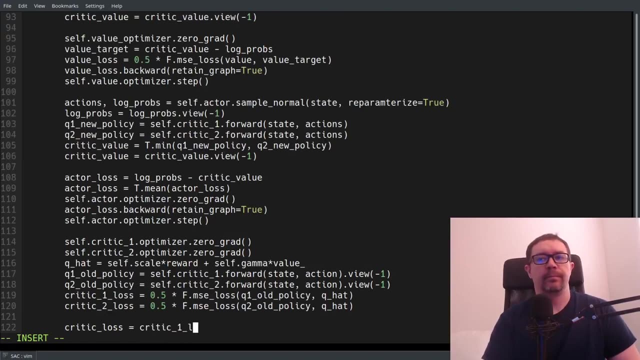 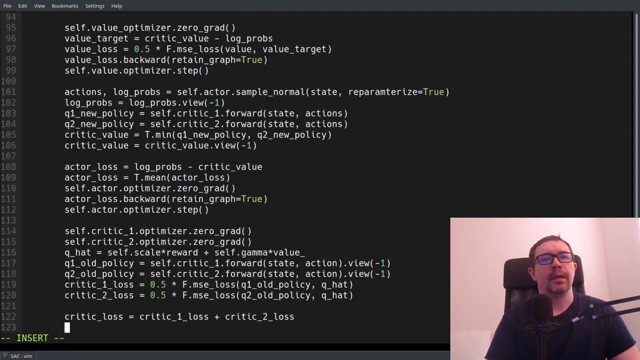 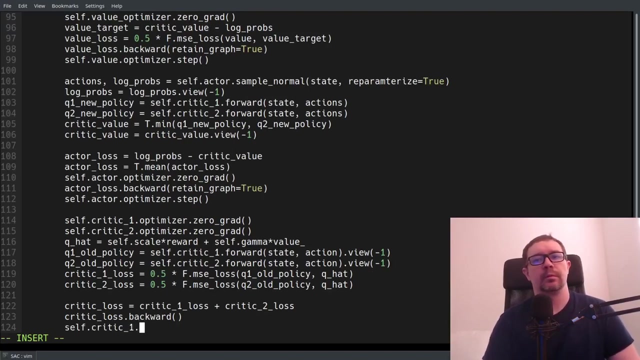 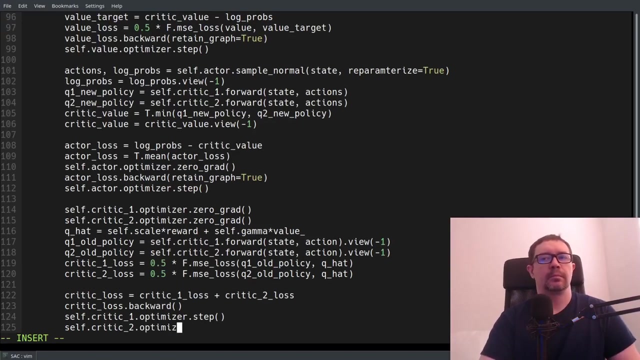 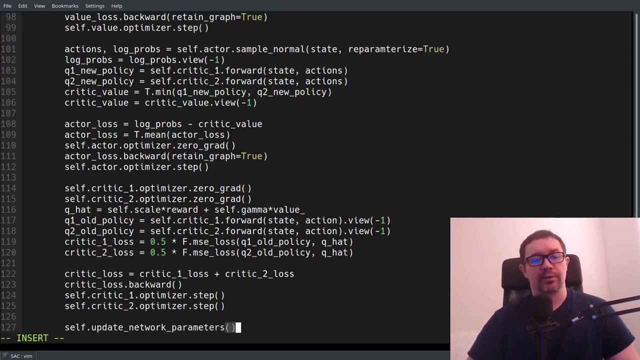 policy and q hat, and then we'll take the sum of the two- the sum sorry- and back propagate, and then the step are two optimizers and finally we want to update the network parameters for our value function. okay, so that is incredibly long, but we're still not quite done. yet we have to handle the main loop. 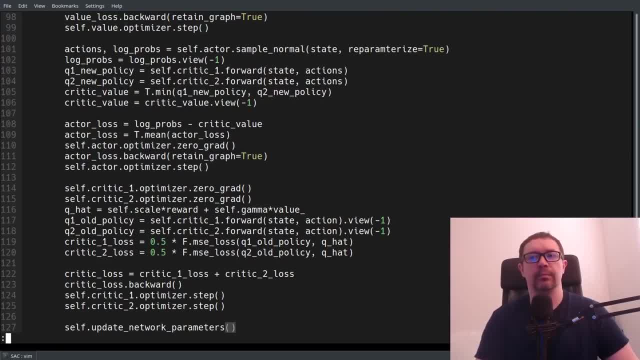 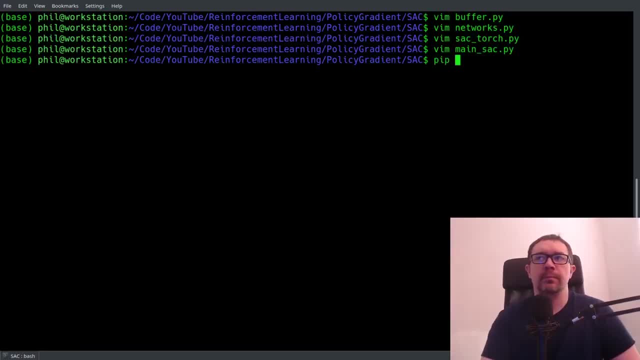 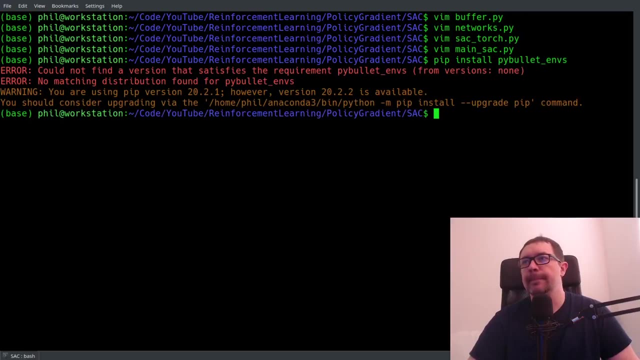 to test everything out. so let's go ahead and write that, but really quickly. before we do that, let's do the following: let's do pip, install pi bullet envs, and this will give us the pi bullet envs, the different chunks that we have in here. we copy it to the standoff. 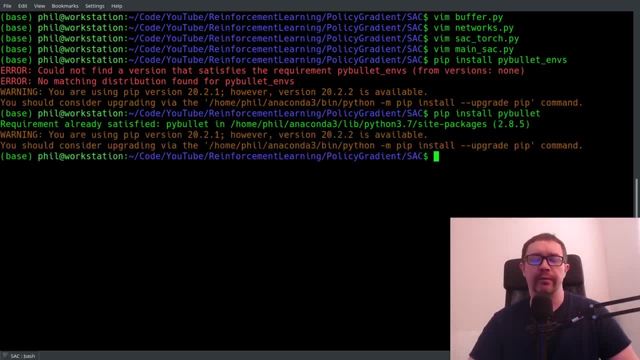 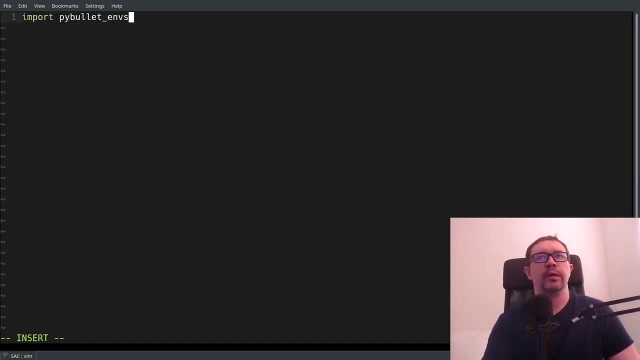 donne Hallelujah, and that will give anything to your comment. oh sorry, it's pip. install pieISbullet. that will give us the PIE-bullet package, which, of course, i already have. then we can come into the main file and say: import PIbullet envs. this will give us access to the pi-bullet environments. if you're not familiar with it, pi-bullet is an open source 3d rendering and physics engine. it's really cool. it has support for virtual reality. it has built in open AIGEM-compliant environments, is also successful thanks to Pi-bullet-envi r dupl. Erik rit, thankful for your interest in the community and the marketing of your own IR5.cart, as well as to keep you familiar with theідmmd and reическаяend for each other. 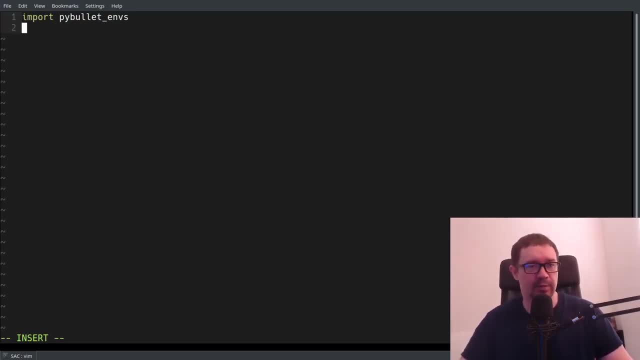 and for the LexSun들이- Haiti施 preguntas等, for It has a couple of built-in agents you can actually use, So it's a really neat package. It's something you can go do a Google search for and look up the documentation. 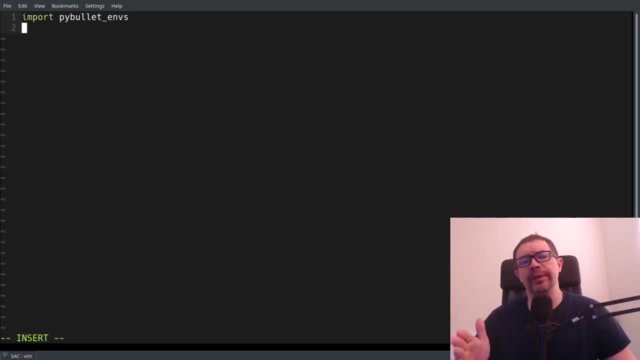 and start playing around with it if you're into that kind of thing. I'm using it here because it executes quickly and it has a non-trivial. you know the inverted pendulum is a little bit non-trivial. You can use the cart pull if you want. 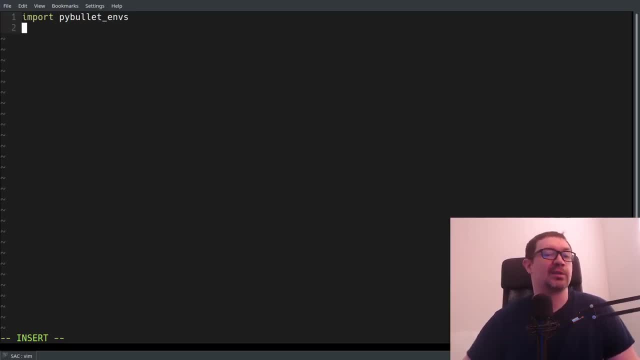 the continuous cart pull, but this is just a little bit less trivial. So we're also going to need Jim. We'll need NumPy- Okay, we'll need our agent. We will also need plot learning curve, So that is just a utility function I have. 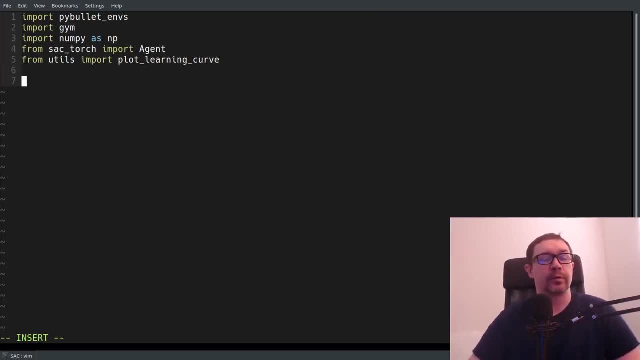 that does a plot with some axes labeled. I'll have to copy it over into this directory. If you want it, do a clone of my GitHub and you'll have it. And if not, just do, instead of plot, learning curve. just you know, do a plot from matplotlib. 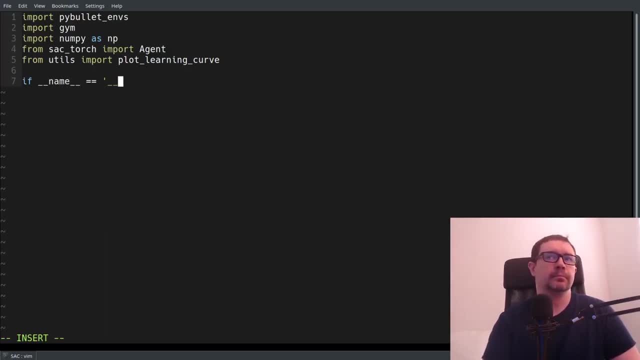 So our environment will be jimmake, inverted pendulum bullet. environment v0. Our agent. So we already have the strong defaults for our alpha beta reward scale. We need our input dimensions and that is envobservation Spaceshape. We need our environment. 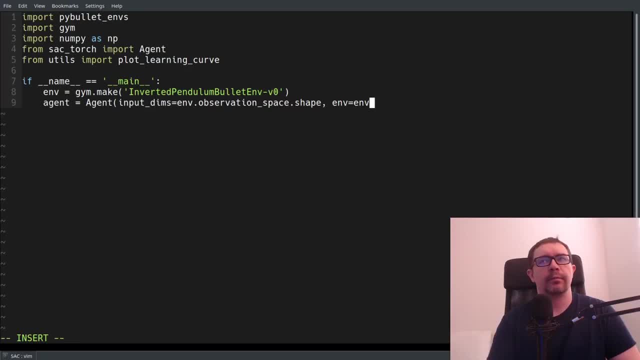 And then we already have strong defaults for everything except the number of actions. I believe Action space shape sub zero. We already have the layer one and layer two sizes, Batch size, I believe tau. we have a strong default for Okay, so that should work. 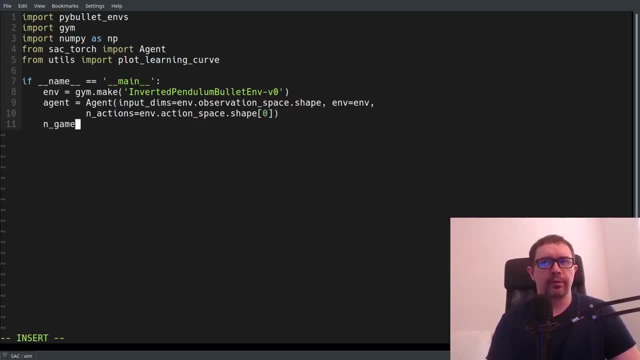 Otherwise we'll get an error. We only need to play 250.. games for this environment And inverted pendulumpng. In fact, yeah, we'll do that. I like to split it into a figure and a figure file. file name: into a figure file. 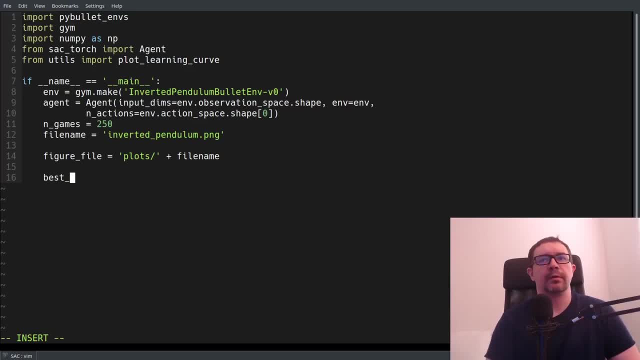 Just how I do it. It's probably not even the best way to do it. So we want the best score to be the bottom end of the reward range and a list to keep track of the scores the agent receives and load checkpoint. So this will determine whether or not. 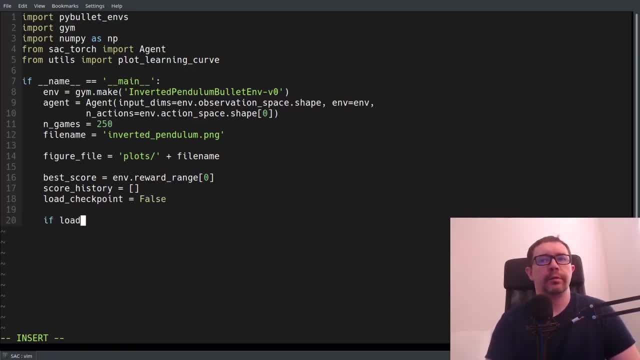 we want to load a pre-trained model, And if you do, then what do you do? So if load, checkpoint, agentloadModels and envrenderMode equals human, So what this will do is it'll render, you know, the agent playing the environment to the screen. 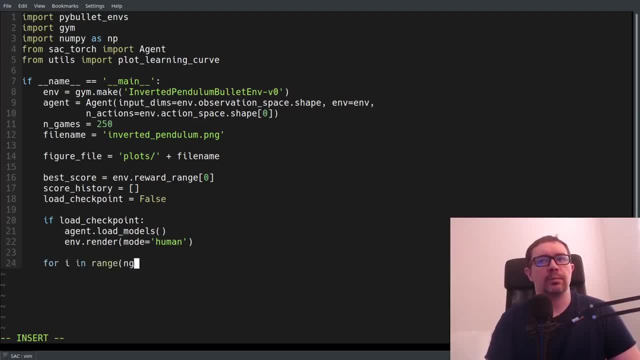 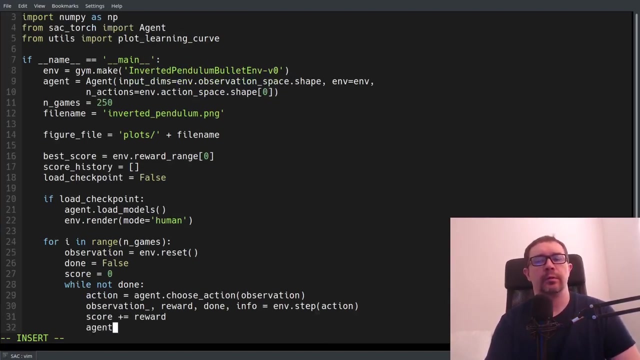 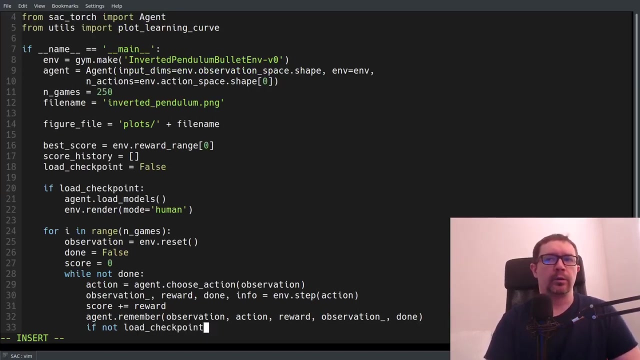 Then we'll say for i in range and games: observation equals envreset, Done equals false, Score equals zero, All not done. Observation: underscore: score plus equals reward, Agentremember, If not load checkpoint. So we only want to learn when we aren't trying to evaluate an agent. 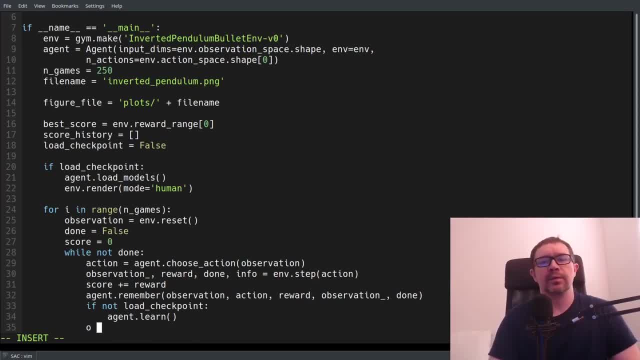 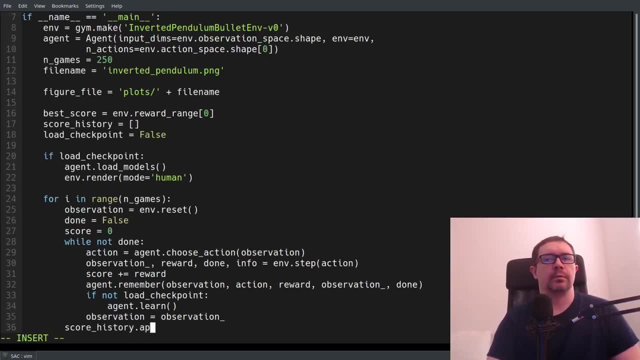 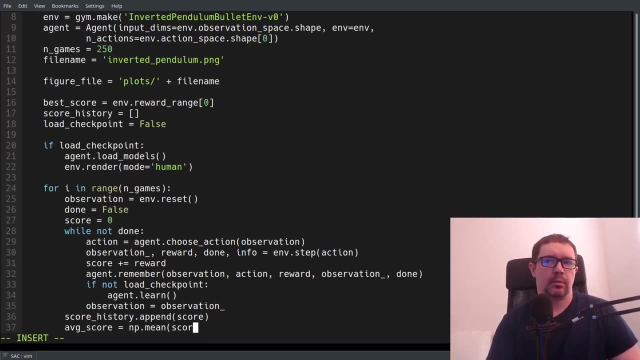 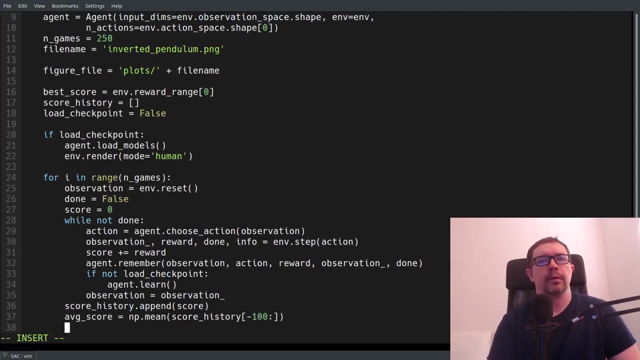 Sounds like my toddler is upset about something, Then we set the observation to the new state. So then at the end of every episode we append the score we achieved and calculate the average score as the average of the previous 100 games and say if average score is greater than the best score. 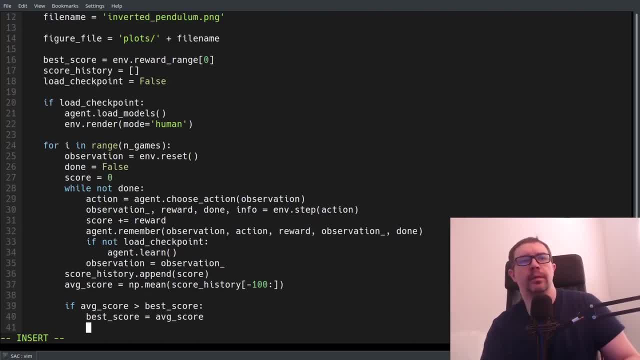 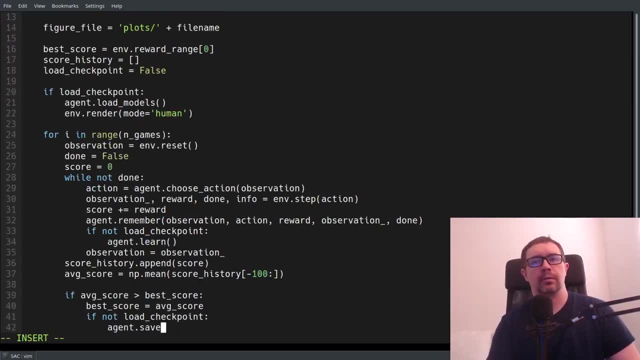 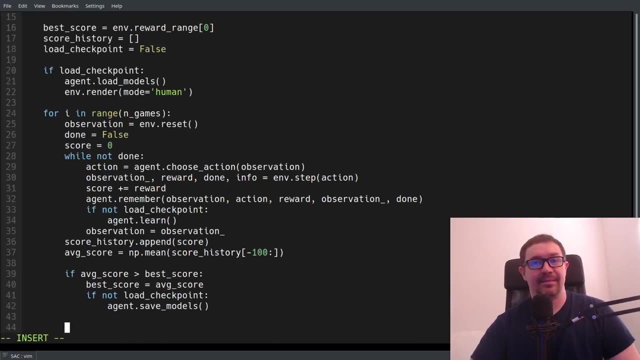 best score equals average score If not load checkpoint. So if we're not evaluating, then save the model. Oh Okay, So sorry. my toddler is throwing a fit His poor grandparents. Episode I: Score percent. 1F score: average score. 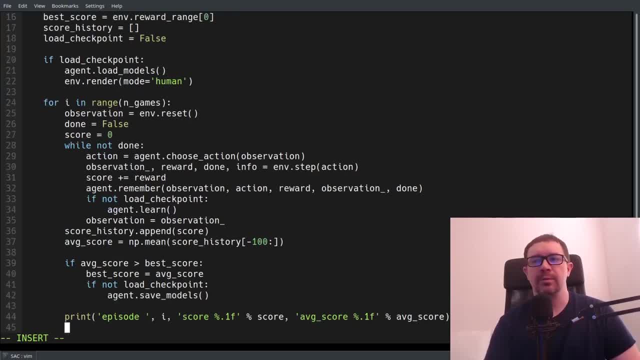 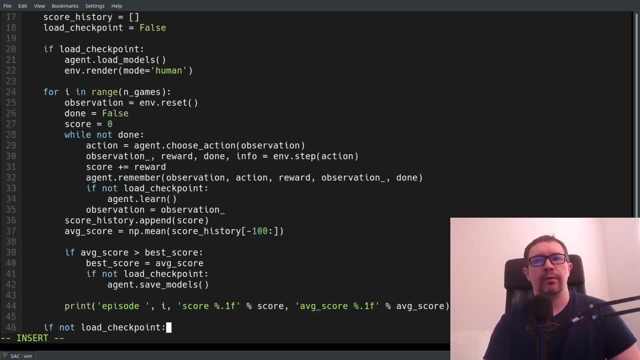 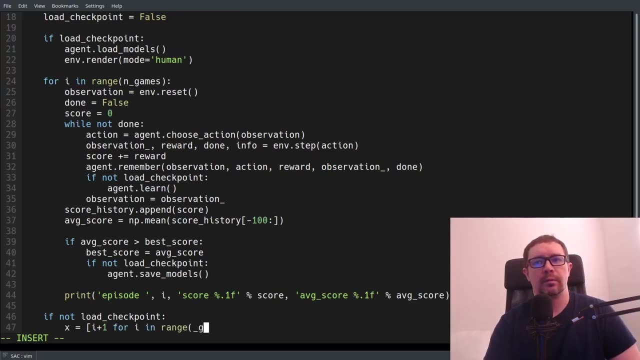 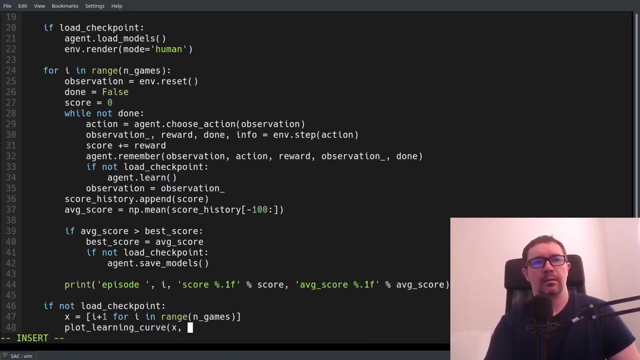 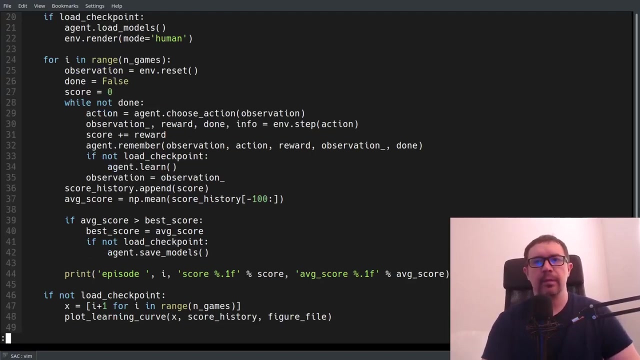 Average score. All right, So that will print some basic debug information to the terminal And then, if we are not loading a checkpoint, then we want to go ahead and plot our learning curve and games and plot the score history. okay, so that is it for a main file. let's 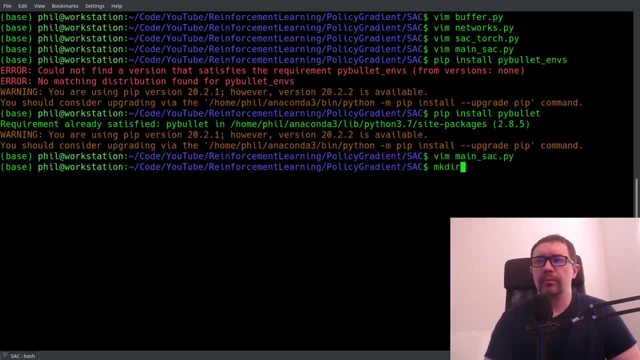 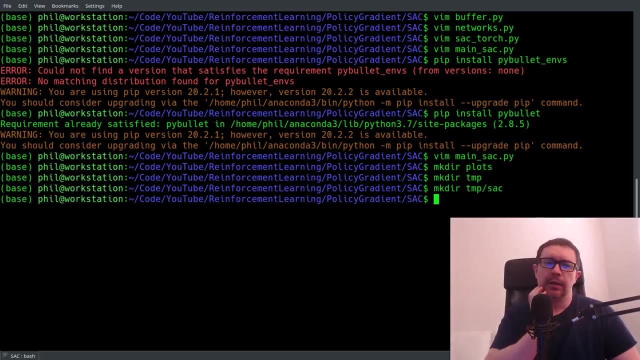 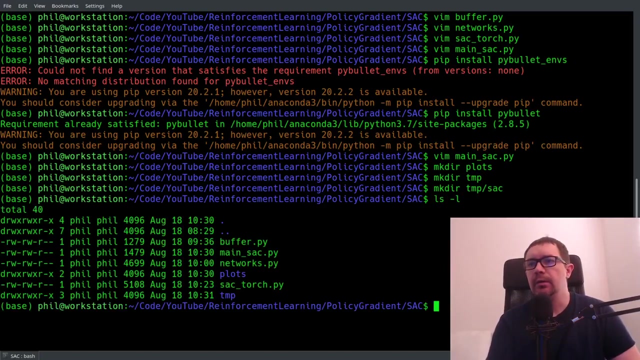 see how that works. so I want to do and make their plots, make their temp. do I need temp slash soft actor critic? I think I do. what else do I need? that's for the, you know, saving models and plots. I want to need to get my utils file, so I 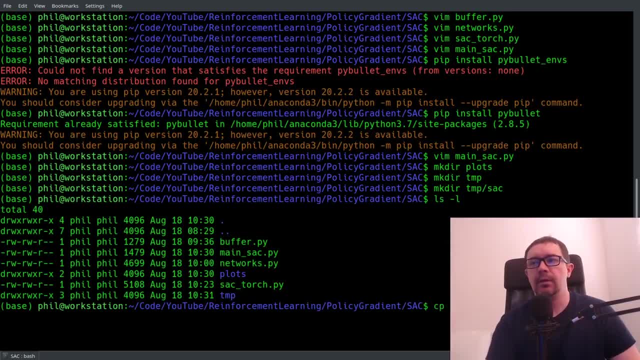 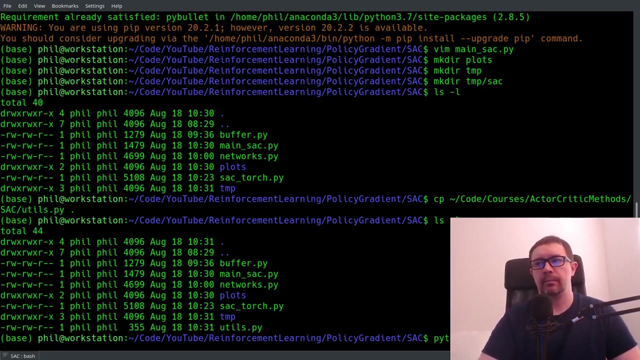 do not have my utilities, so we will do a copy. this is just something you shouldn't do because this is local to my machine: core code courses, which you can't see. that's fine actor critic methods. so I've got your critic utils. you can copy that here and now I have my utilities. okay, now we're ready, I think. 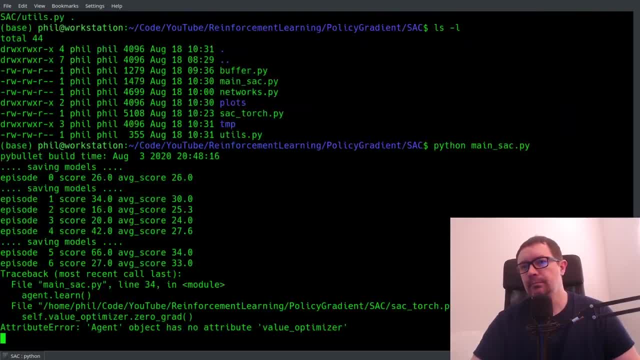 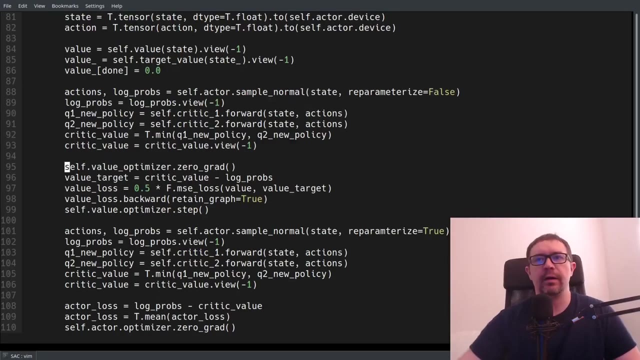 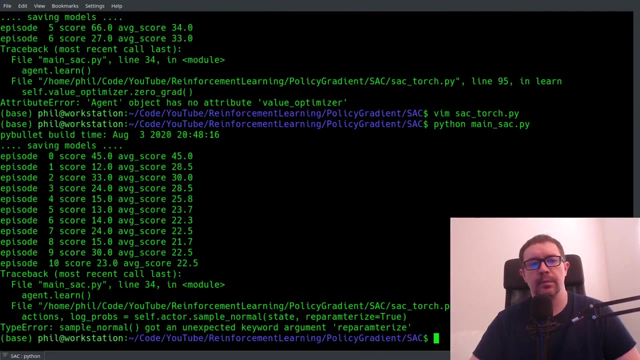 see how many typos I made. value agent has no object, no attribute, value optimizer. it's because it's a value dot optimizer, not value underscore. so that is in sack. torch. line 95: value dot optimizer. okay, try it again. I read I misspelled re-parametrize in line 1. 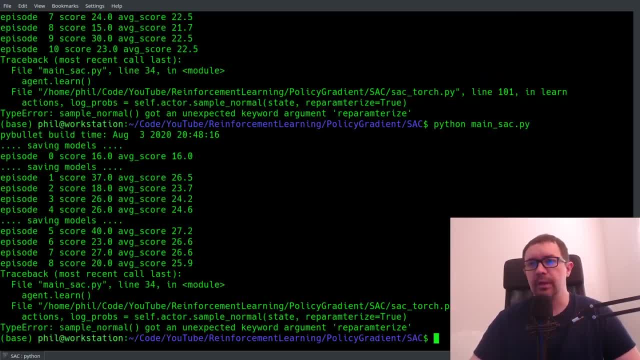 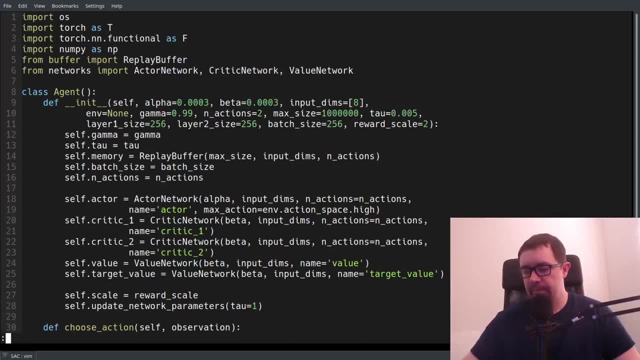 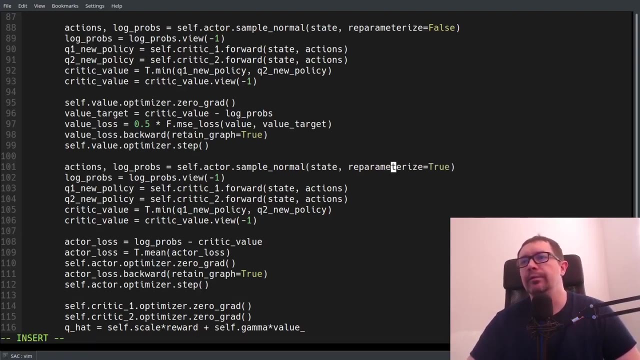 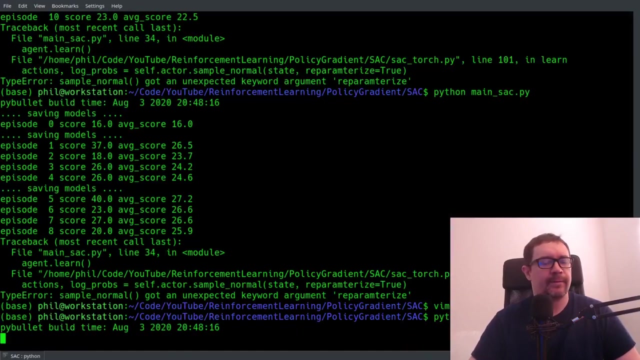 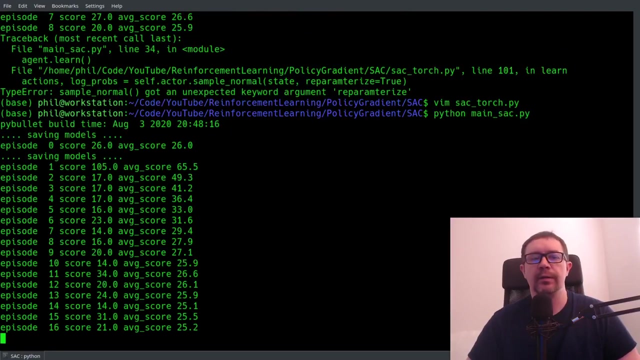 whoops one. do them not try to run it again? sue them, that's in line. I'm getting a spam call. all sorts of chaos today. line 101: Reparameterize. I think that's right. All right, So there it goes. So I'm going to go ahead and 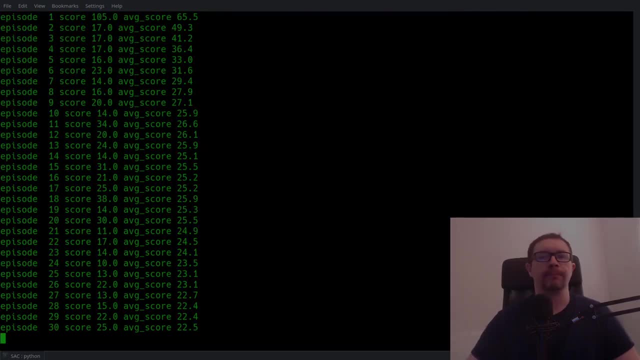 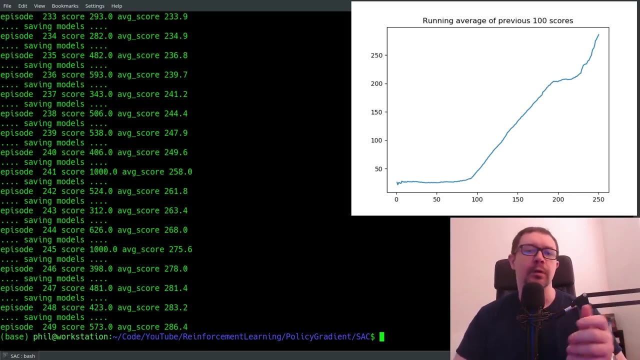 pause the recording here and come back when it finishes running. All right, So this has finished running and you can see that it is in the process of learning, So there is a little bit of run to run variation. When I run this for the course, it achieves a score of a thousand within 250 games. 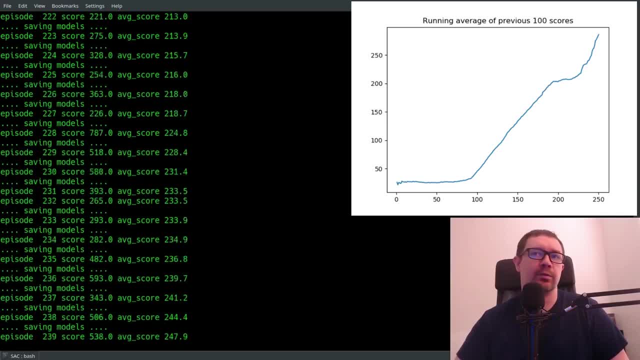 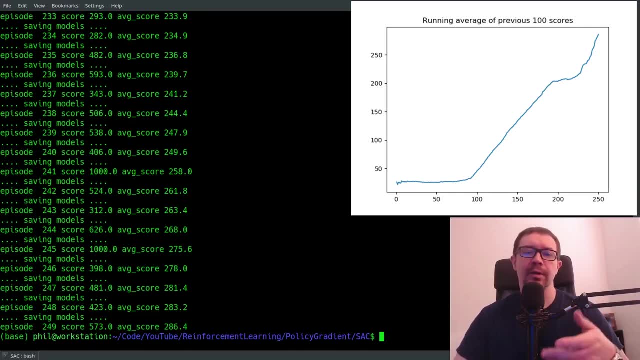 You can see here it was generally trending up when the last 30 or so games scores that were going sky high towards a thousand. So it learned a little bit slower on this particular iteration. Sometimes it learns a little bit faster, sometimes a little bit slower, despite the fact that the 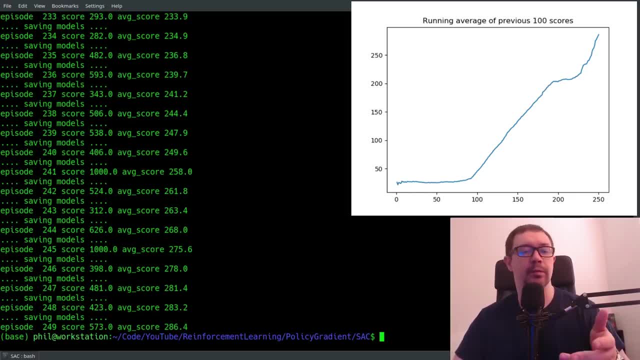 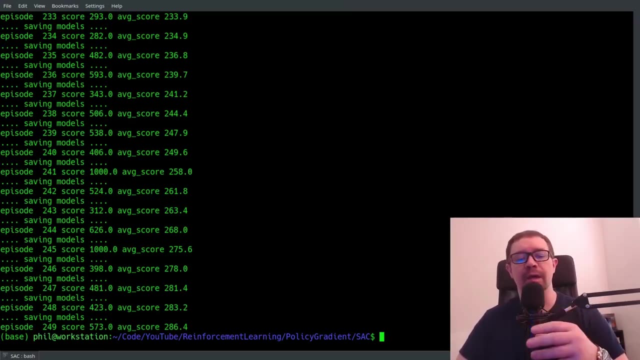 algorithm seeks to minimize run to run variation and improve stability. There is some run to run variation and not rock solid stability. That's to be expected with deep reinforcement learning. But again, to recap, the fundamental idea behind soft actor critic is that we are using a maximum entropy reinforcement learning framework, but the entropy comes from. 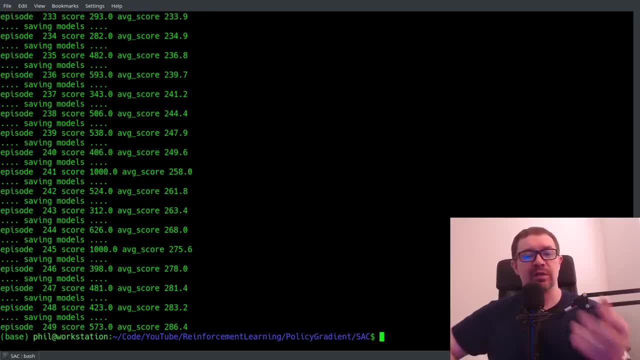 scaling the reward factor. This encourages exploration or encourages exploitation, depending on that scale factor. As that scale factor grows, then the signal to exploit grows. as the reward scale decreases, then the tendency to explore increases. So it is a way of fine tuning. 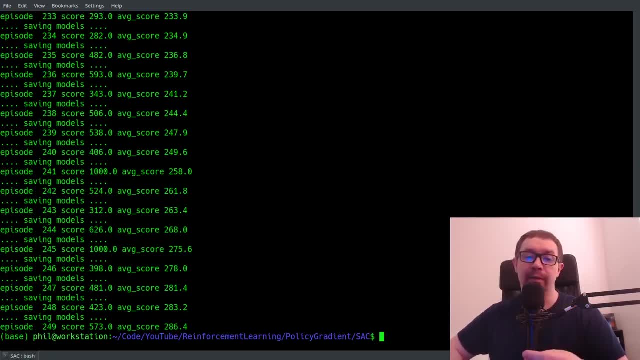 the performance of the model And in fact it's the only real parameter you have to play with for the performance of the agent. You don't have to tune learning rates, You don't have to have to tune the number of neurons for your hidden layers. You just tune that reward scale to get an idea of 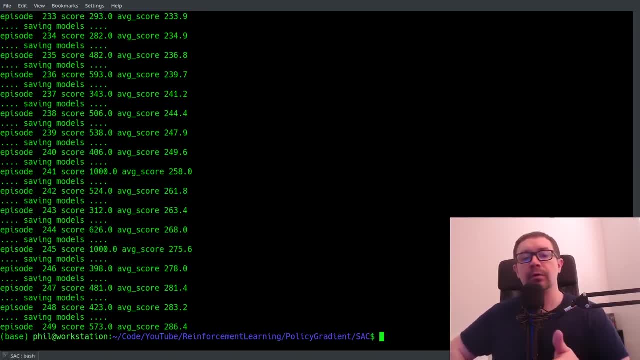 how to improve the performance of your model. If you want to learn more in depth on this, if you want to learn more in depth about other deep reinforcement learning models, such as TD3, DDPG, double Q learning, dueling, double deep Q. 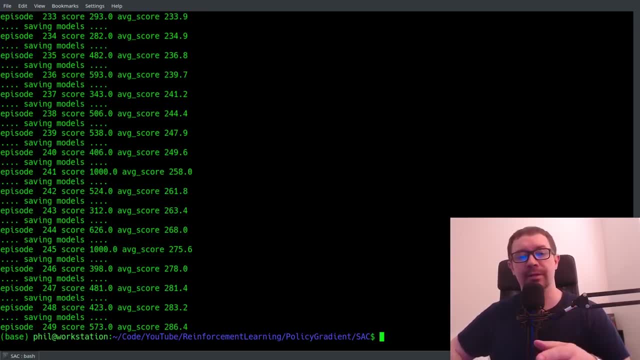 learning. check out the links in the description. I sell courses on all these topics through Udemy and they're on sale right now. If you can't afford that, then by all means please subscribe, because that is free. Hit the bell icon so you get notified when I release new content. 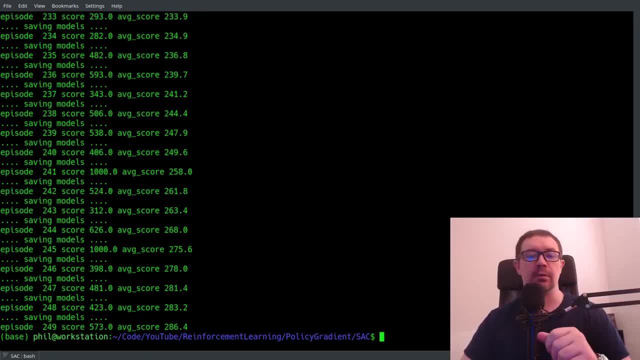 hit a like, leave a comment and I'll see you in the next video.